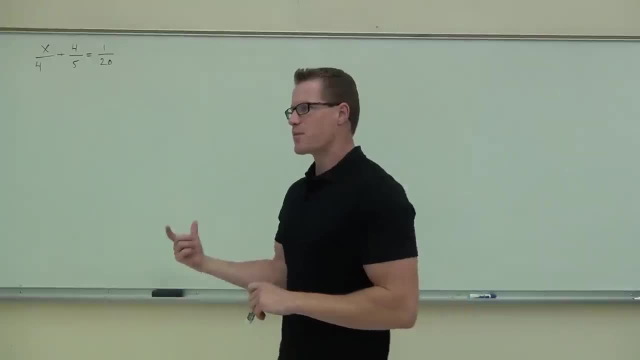 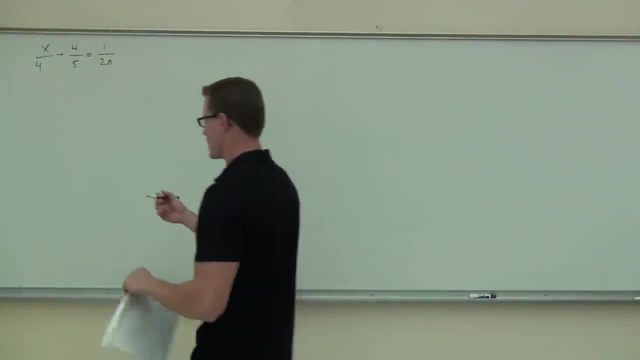 We just cross things out. That's what we do. So, with this type of problem, the first thing we need to do, just like anything else, just like on your homework, we're going to find the LCD. So, on our steps, which we're going to write down right now- hopefully you're waking up, because some of you guys look tired. 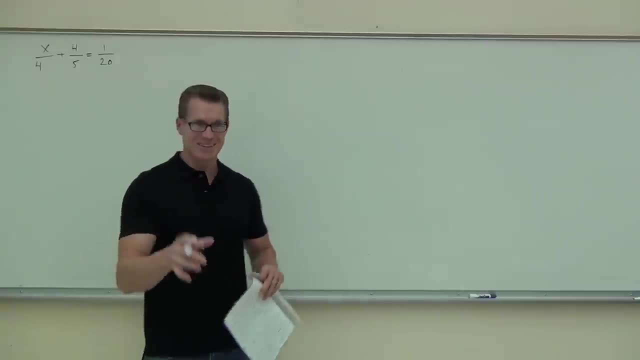 Man, you've got to wake this up today. This is a good lesson. I practiced this one over the weekend like in the mirror and stuff. No, I'm just kidding, But you need to have this one down. What's really important is that you see the difference between this section and the last section. 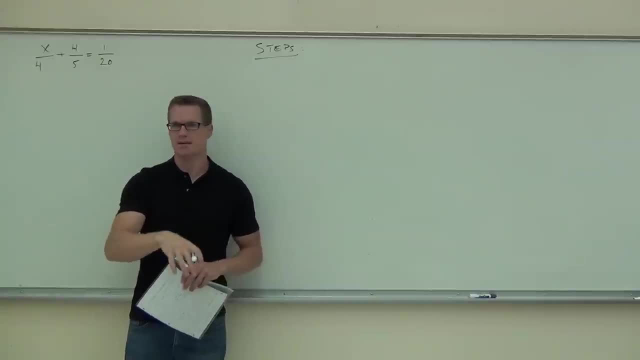 I cannot have you do the same thing. You do the same thing on this section and the last section and you mess yourselves up so bad you're never going to finish the problem. You have to see the difference here. So first big difference: these have equal signs. 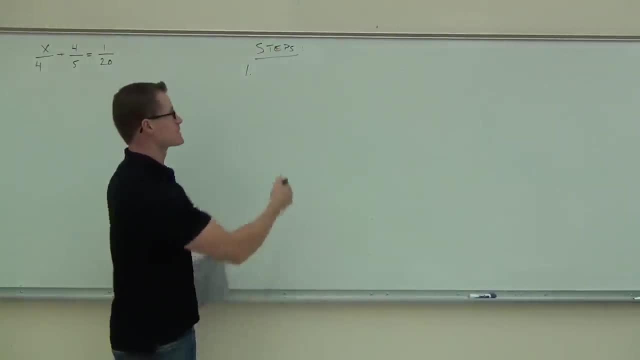 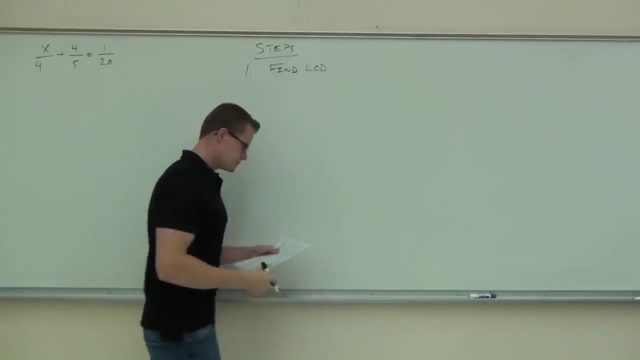 That's why we're going to do it completely different. What thing is similar is step number one. you must find the LCD, And in order to find the LCD you might have to factor first. We learned that on your homework, right. 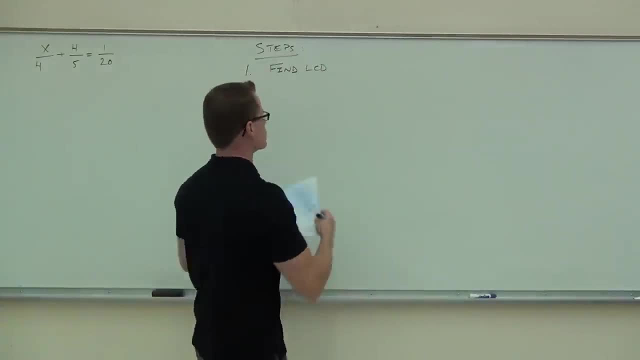 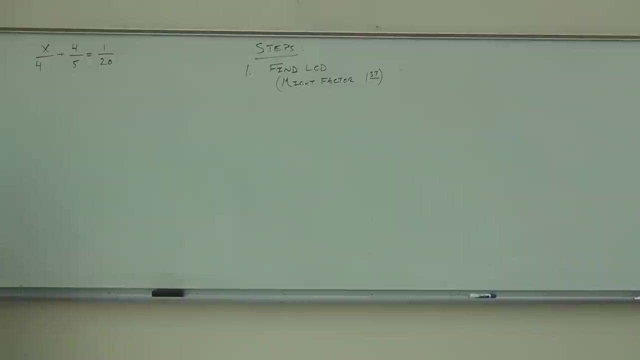 You have to factor those denominators in order to find that, So you might have to factor this first. Let's go ahead and do this with this example. Now, this is kind of an easier one because, well, we have these numbers. 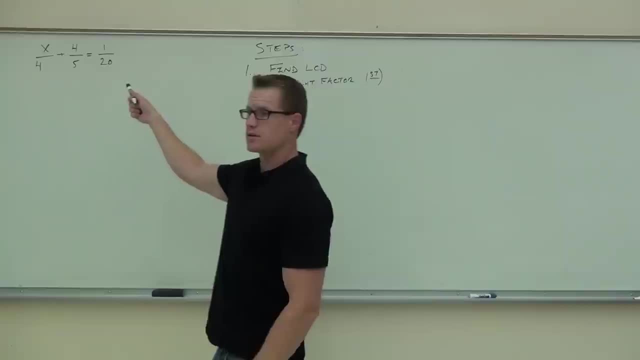 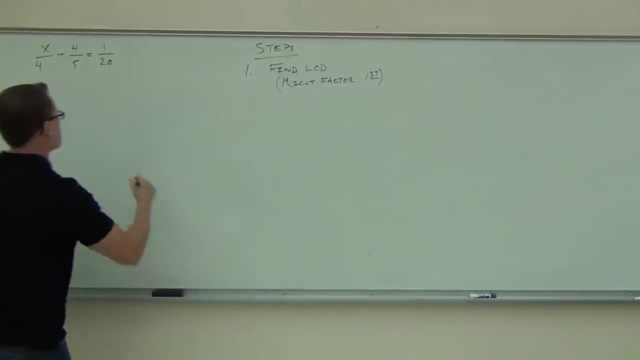 But let's practice that. What is the LCD in this case? Is it 20 from these two, or 20 when you consider all three of them? So we're still looking at every fraction you have and we're going to take. LCD is 20.. 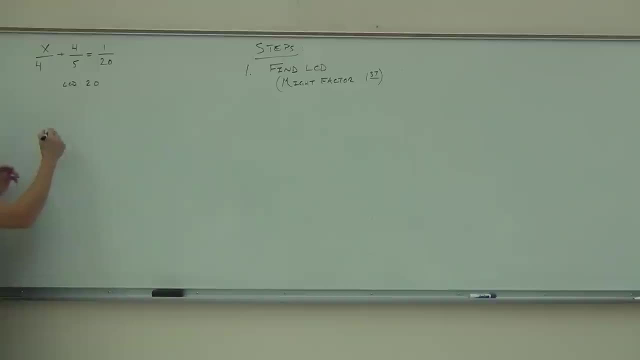 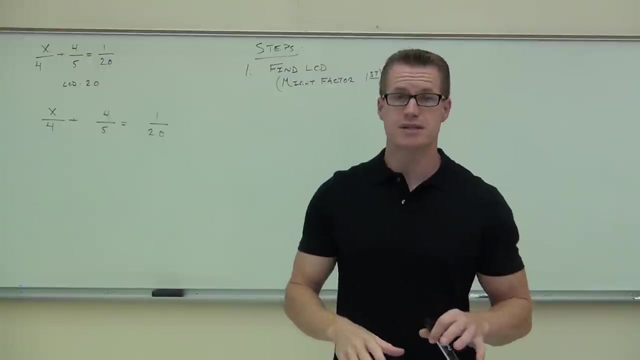 And I'm going to rewrite this problem down here because I'm going to show you what to do. I have a little bit more space, though. Here's where the difference is happening. This is what you need to see in this section. Last time, what you would do in the last section if there was no equal sign is right now. 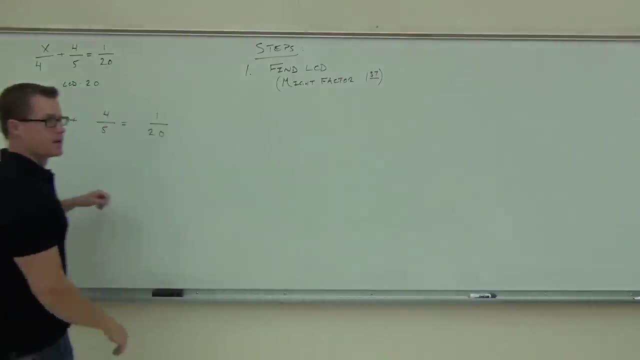 pay attention to the board real quick. what you'd be doing is you'd multiply this by 5 over 5, this by 4 over 4.. Are you with me on that? And you'd get 20.. That happens if you don't have an equal sign, because you don't have two sides of anything, right? 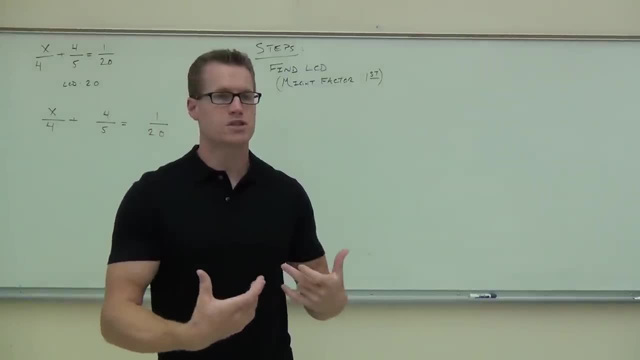 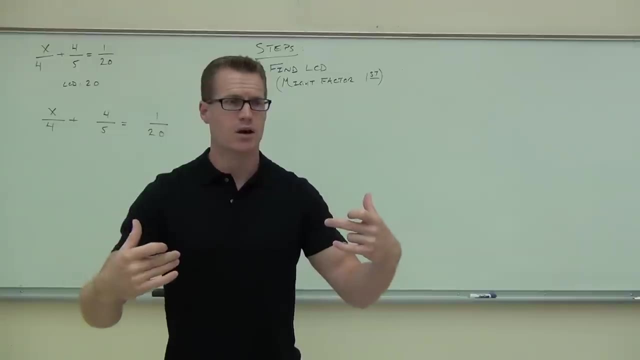 You just have expressions that are added or subtracted. When we have two sides, the process changes. We're going to use the fact that we have two sides of an equation and the fact that I can multiply each side, or, in other words, every term. 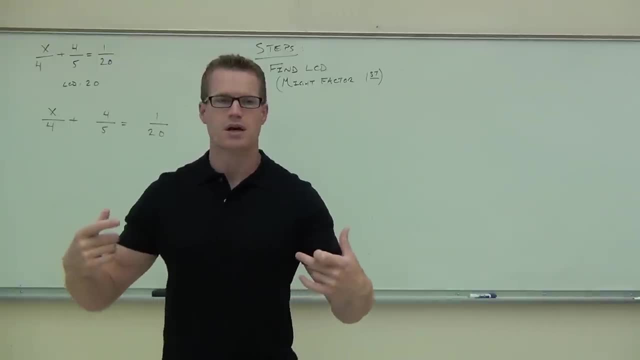 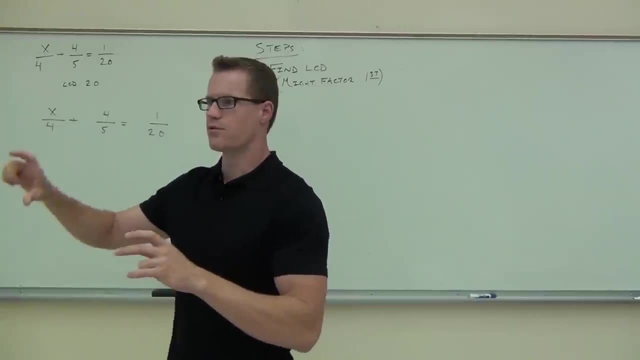 Those words should be ringing a bell for you in first day of class, first week of class: that if I have two sides and multiply every term by the same number, it's still equal. So instead of doing the 4 over 4 and the 5 over 5,. 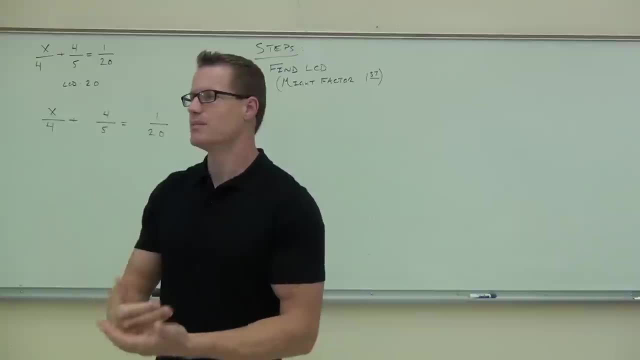 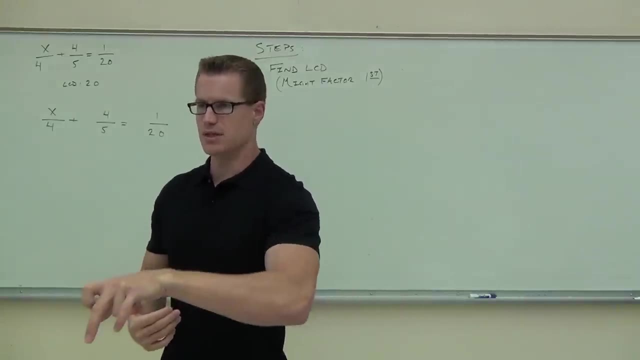 we're going to make this a little bit easier. We're going to go ahead and eliminate the denominators in one step by taking the LCD and multiplying every term by the LCD. This is what we did the first day of class. is we got refractions this way? 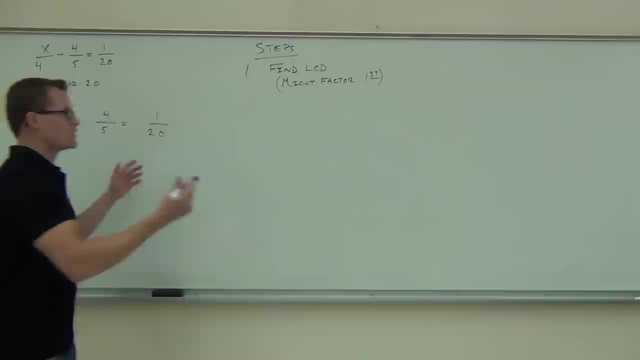 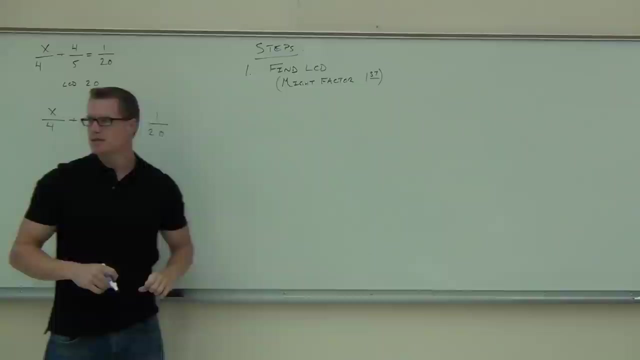 So what I mean by that? hopefully this looks familiar to you. we say: okay, what's our LCD? Oh, we have 20.. What we're going to do with that 20, we're going to multiply both sides. When you multiply both sides of an equation, we get that the equation is still a true statement. 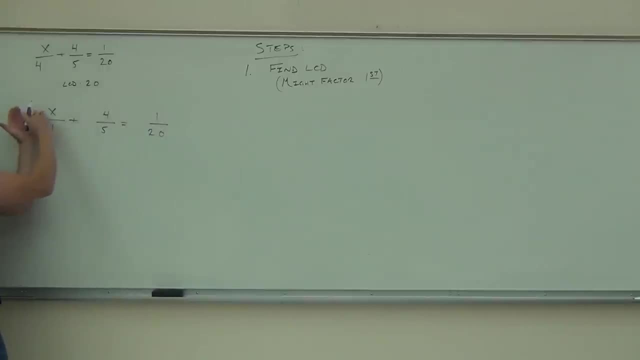 So we'll say: I'm going to multiply both sides. If you remember both sides, that meant every term. If you don't remember that, go back and watch that video. We've already done this particular problem already. So we're going to say, okay, I multiply this by 20.. 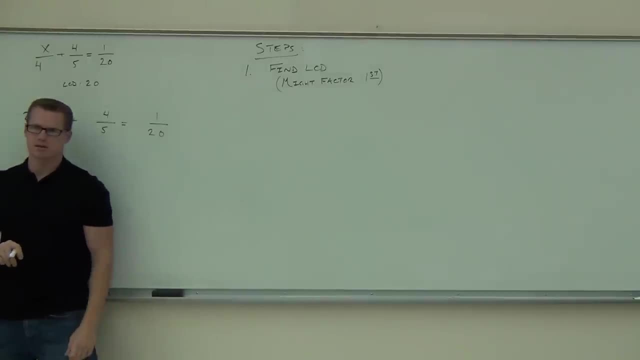 Do I mean 20 or 20 over 20?? Which one? in this case, Just 20.. I don't need 20 over 20.. That's going to make your fractions huge. You don't want to make huge fractions, do you? 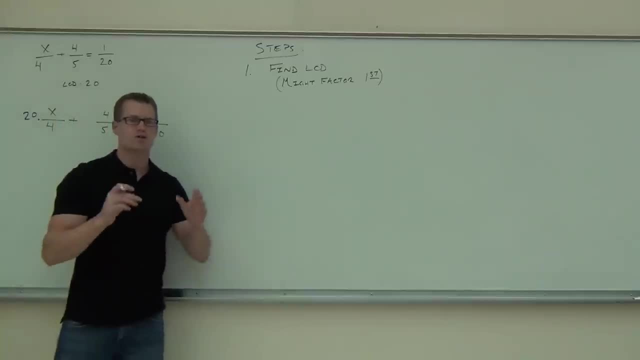 You want to get rid of fractions. That's what we're trying to do here. Don't multiply it by a number over something. It even makes it a fraction. That's what we're trying to do here. Don't multiply it by a number over something. 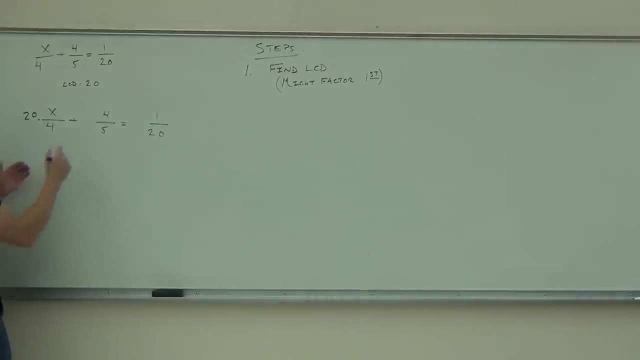 That's what we're trying to do here. Don't multiply it by a number over something. That's what we're trying to do here. So we have 20,, we have 20, and we have 20.. Not 20 over 20.. 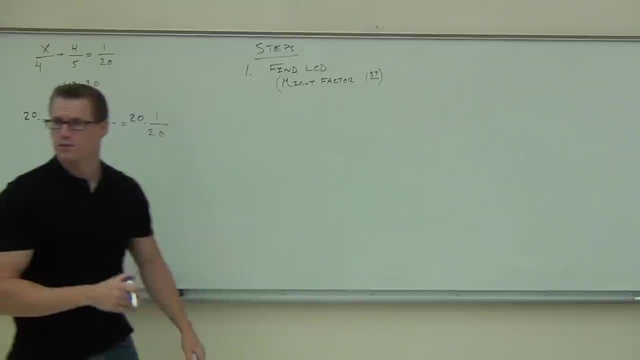 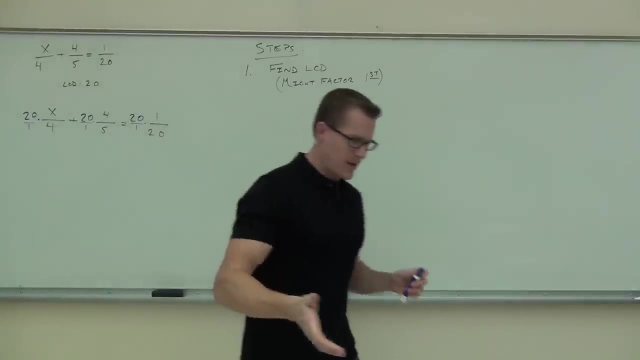 What is it? 20 over what? 1.. Yeah, you can put 20 over 1 if you want to. So we found the LCD. We might have to factor that first here. We don't have to. We're going to multiply both sides. 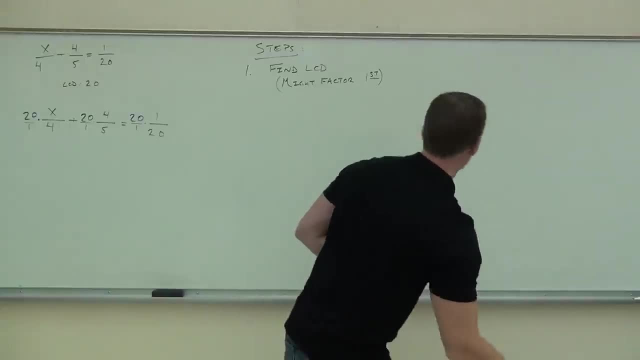 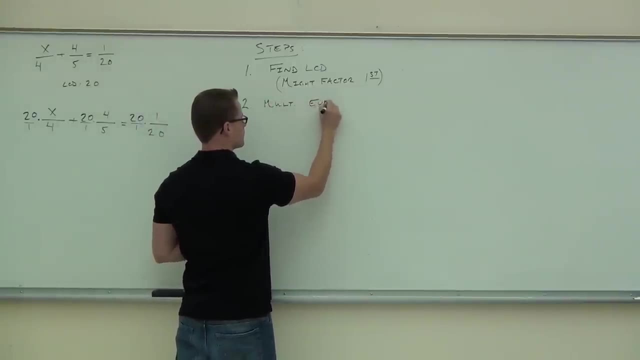 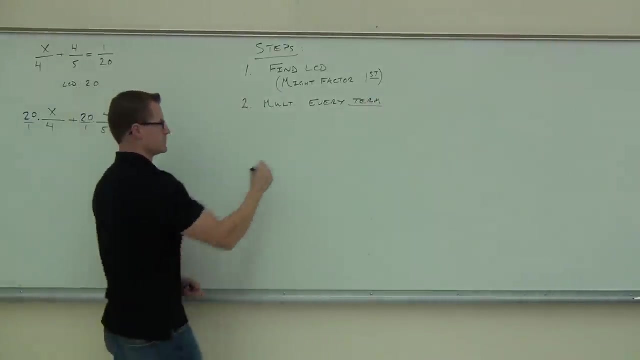 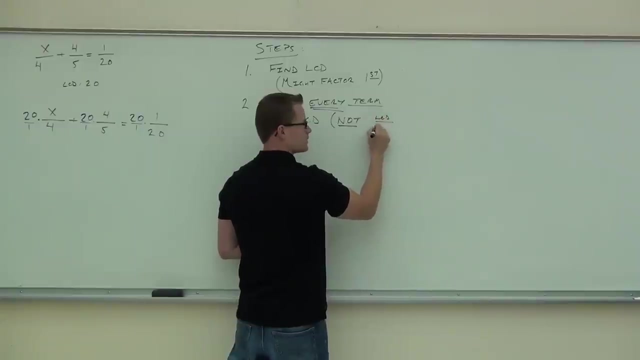 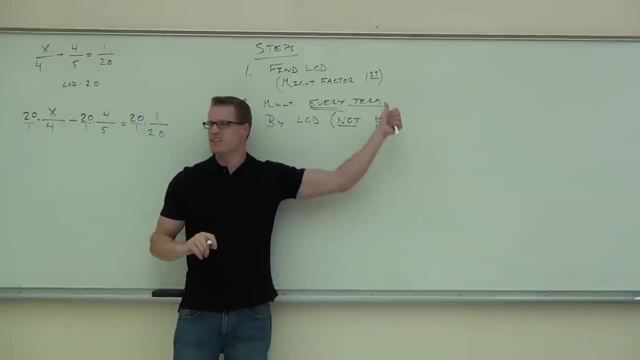 I'm going to make a little note here. When you have equations, you're never multiplying LCD over LCD. You never do that. That doesn't work for us. for equations, We're trying to get rid of fractions, We're not trying to make them bigger. 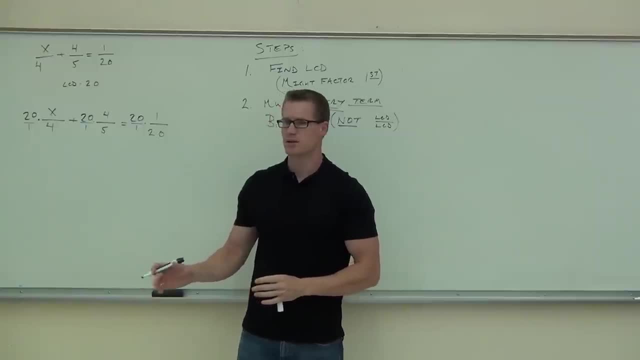 This is not like addition and subtraction, where you have to do that. Here we have equations, You have two sides. We're using that fact to get rid of fractions for us. How many people feel okay with what we just talked about so far? 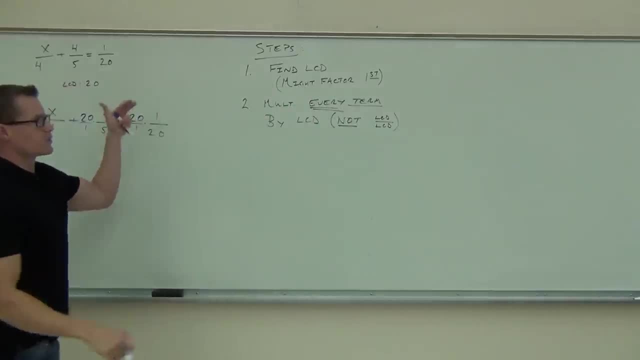 Good, Now let's see why this works. So we found LCD. We've multiplied every term by the LCD. That's right here, Hey, we don't have to multiply. Does that simplify? Well, it simplifies here. That's why we have the 1 down there, right? 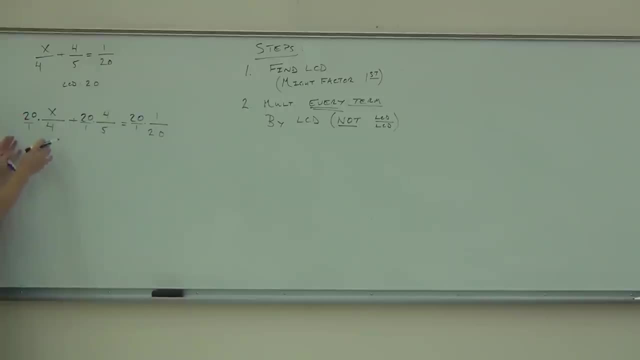 Because we don't need that 1. to simplify with anything, It's not. we're not going to make a 20.. We don't need that. The 4 changes into a 1.. The 20 changes into a 5.. 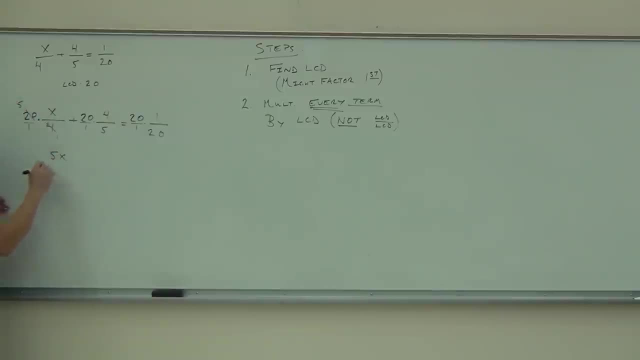 And what's this going to be? 5x Here we have. 5 goes into 5 one time. 5 goes into 24 times. So we have plus 16.. On the right-hand side, what happens there? 1. 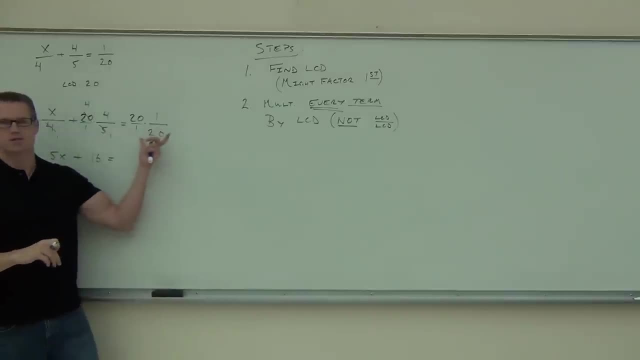 Can you notice? look and notice something. This is the easiest one to notice this on. I'm going to change it slightly. Don't change your problem, Just watch. If I put 20 over 20, if I did that, that's going to be 20 over 400. 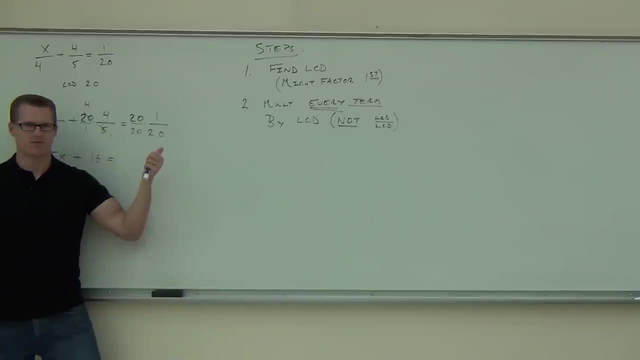 Do you want 20 over 400?? Probably not. That's not going to be very fun. You don't want to do that right. You want something easier, not something harder. So we multiply every term, because we have two sides of this thing. by the LCD. 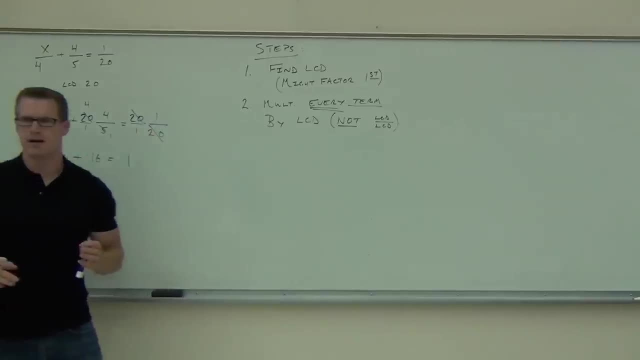 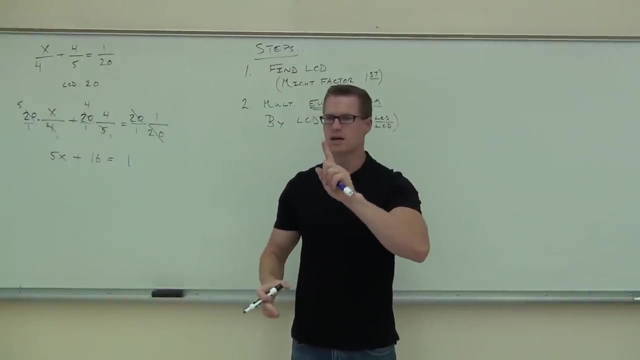 We simplify what we do, We can, And now we have a very easy equation. after that, Isn't that nice. Isn't that nice Something from fractions into something without fractions, by one step. All you have to do is find the LCD. 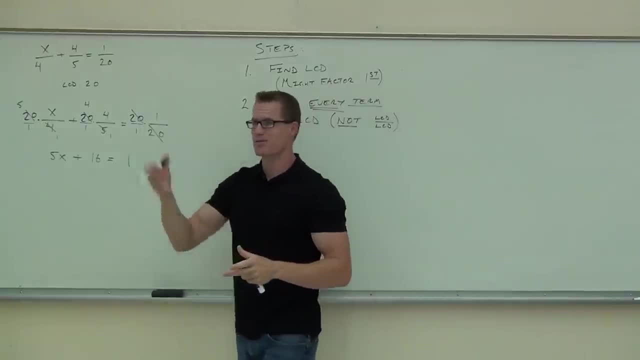 Don't do the LCD over the LCD, but multiply every term by that and cross stuff out. It's going to work. You will get rid of fractions Now, after this. this is a very easy problem. We well, for you guys, it is. 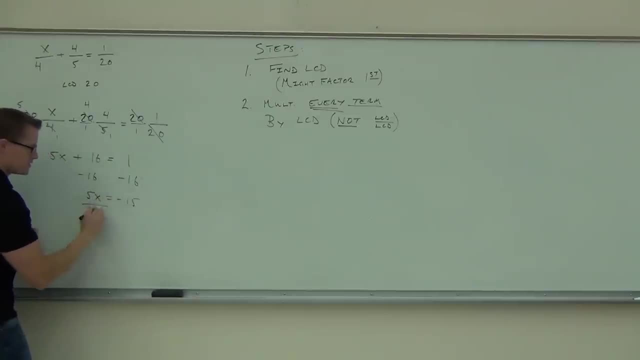 Subtract 16. We get 5x equals negative 15. We divide by that 5. We get negative 3.. 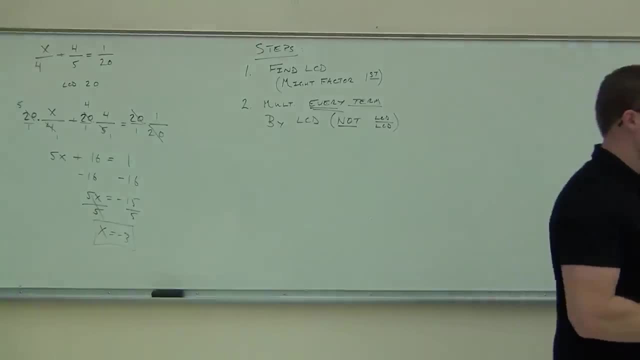 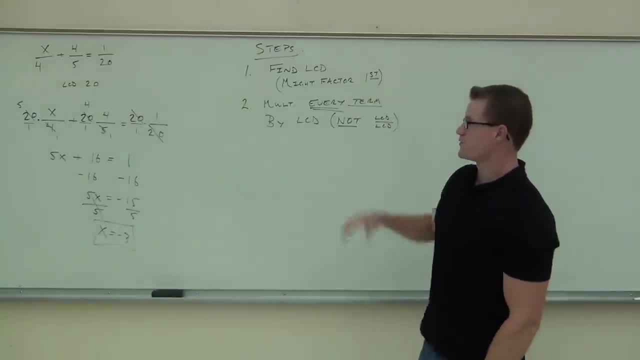 We check our work. You can plug that in and check your work. That's going to work out and we're done. So a couple things. Of course we still have to find the LCD. Of course we're multiplying every term. 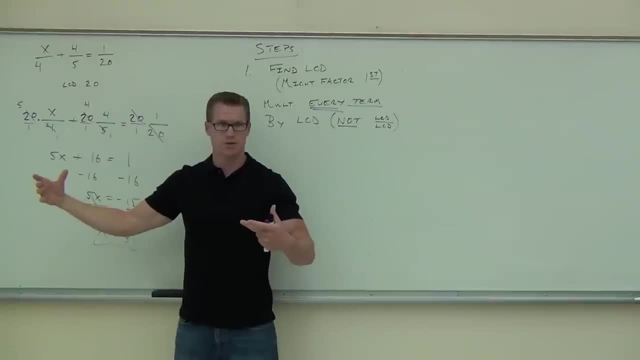 You can't skip a fraction on this case. You can't do this. in other words, You can't just multiply these two and forget about this one, or multiply this one and forget about one of these. It's got to be every term in there. 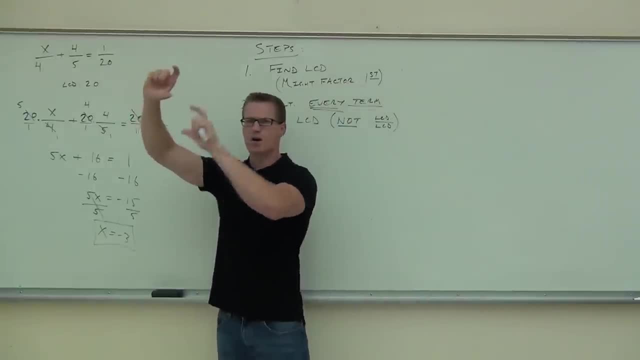 You have to do that. We'll also just multiply the LCD, not LCD over anything Besides. 1. It's not LCD over LCD, Or it's not 4 over 4, or 5 over 5. We're not doing that sort of thing here. 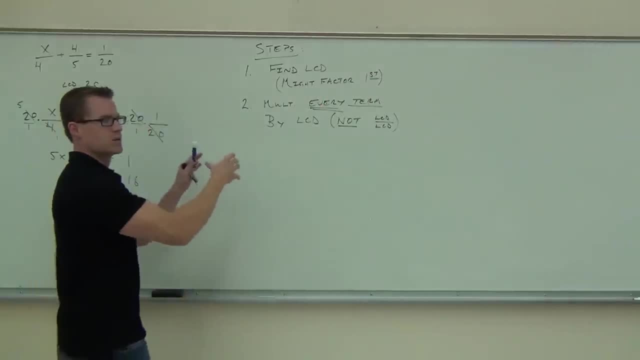 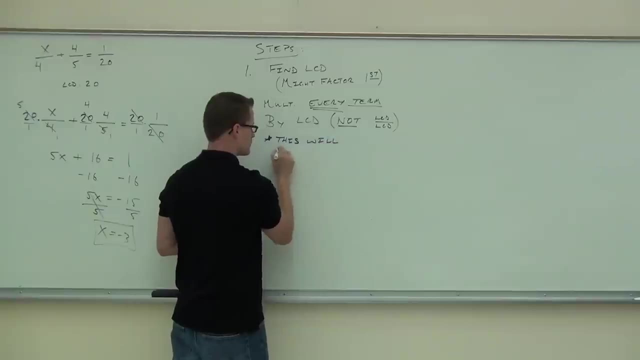 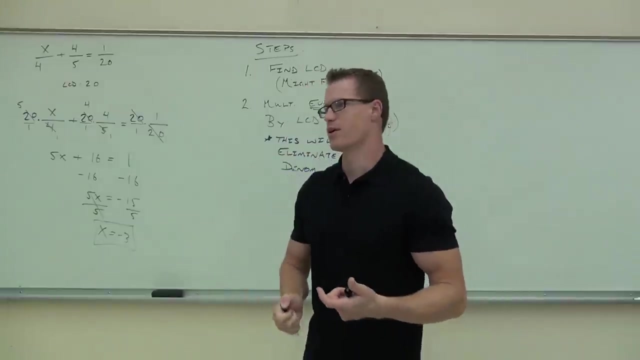 We're trying to get rid of fractions. These are meant to eliminate denominators. Now let's try this with a couple more. We're going to build ourselves up to ones that look really hard. All right, They're not going to be very hard, because you can get rid of denominators. 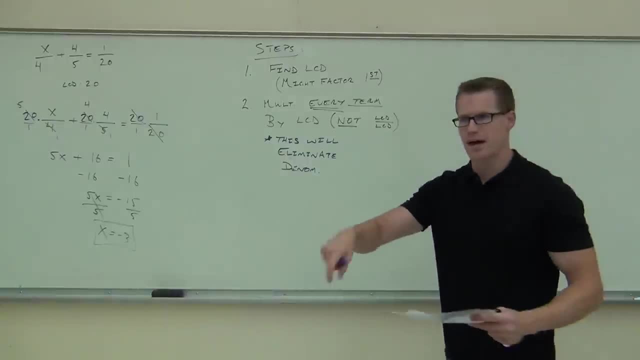 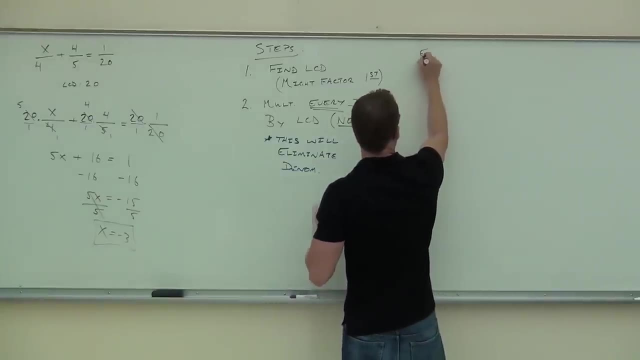 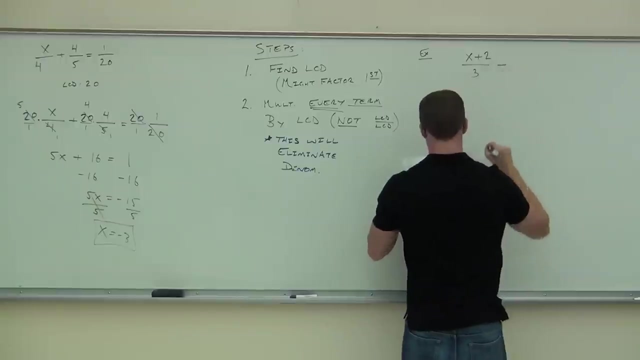 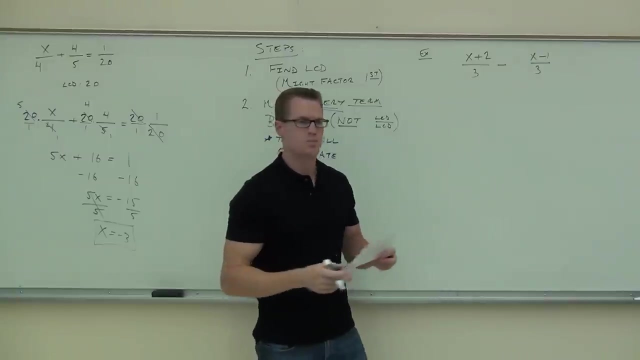 That makes things really easy, But they're going to look really hard, So we're going to build up to that to see that we can really do this. in any case, By the way, when I'm writing these problems down, I'll often leave a little bit of space. 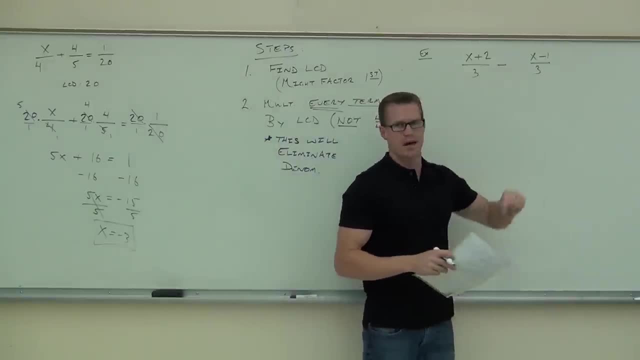 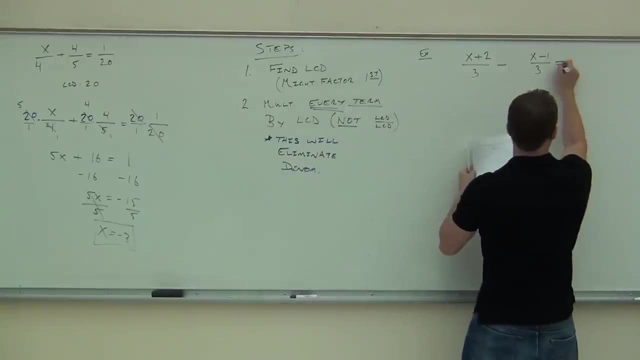 in between the sign and the fraction, Because I know I'm going to have to multiply by something. Is that clear for you? That way you don't have to have it all scramped like crunched in. Oh, you know what? 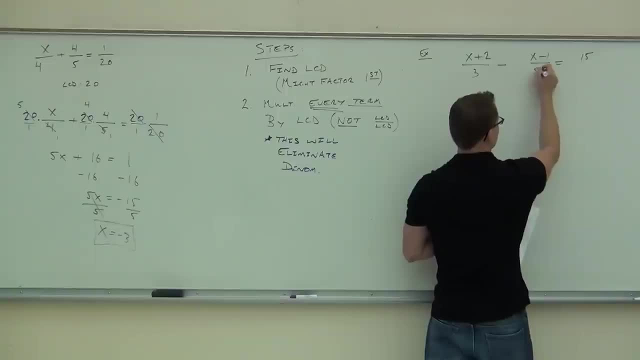 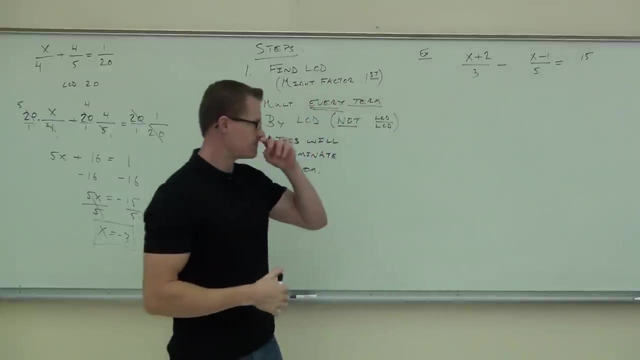 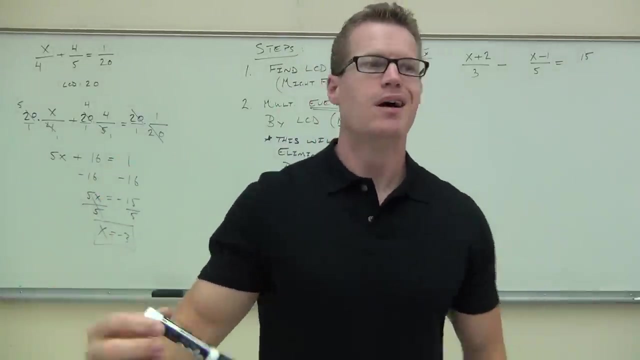 I made a mistake already. Change that to a 5, please. Okay, Let's do this problem together. Now, one thing that I'm going to show you, because you're going to have to do this Before we do even the very first step here is: you might want to make things. 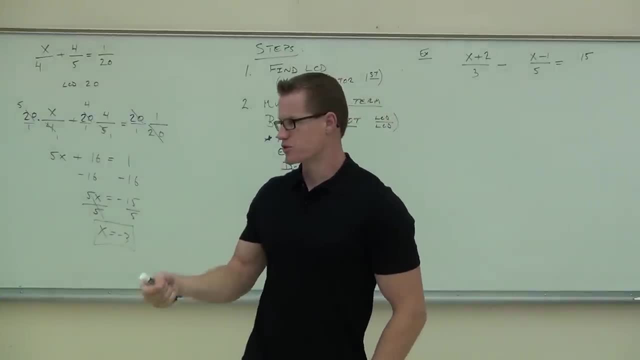 just like in the last homework, make things into fractions first. Right here do you see? we have one term that's not exactly a fraction, yet Make that into a fraction. That way you don't confuse yourself with your LCD. Here that number wouldn't really matter for us. 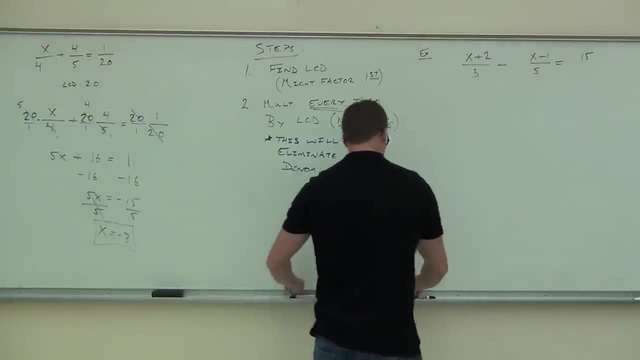 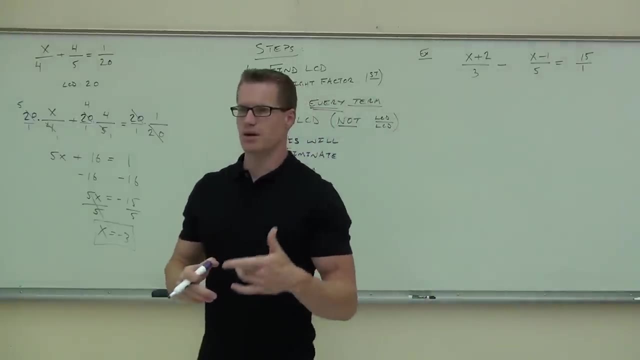 But the point is, let's make this into a fraction first. And how do you make a number into a fraction? Just do that real quick. That way you don't let that 15 get confused in your LCD. All right, Because if that number was like I don't know 30 or something and you tried to find the LCD, 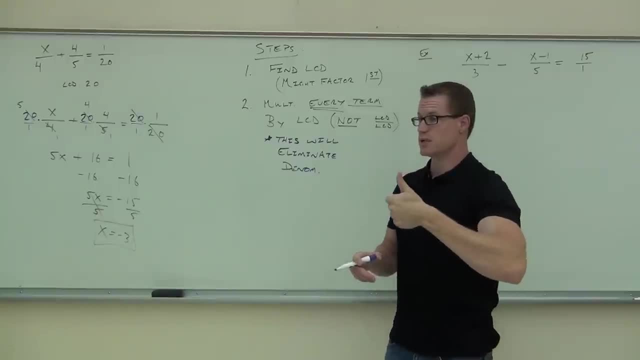 and you considered that that's going to make it a much larger LCD than what you need. Are you with me on this? So make your fractions first. Now let's go ahead and find our LCD. Let's look at those numbers. 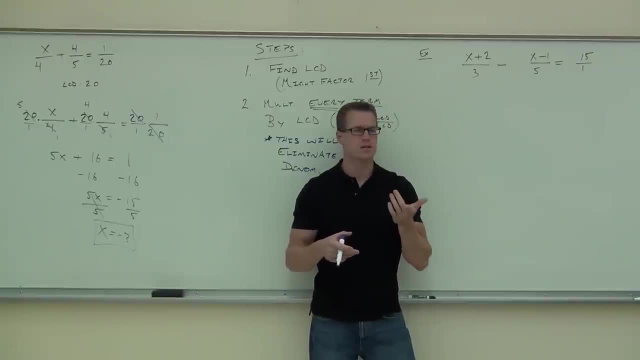 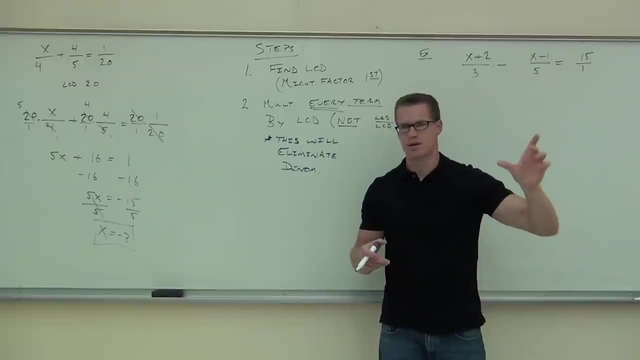 Our denominators are 3,, 5, and 1.. What's our LCD? Fifteen? Yeah, it is 15.. In this case, it is that number. I just didn't want you to think that that 15 had anything to do with the LCD in this case. 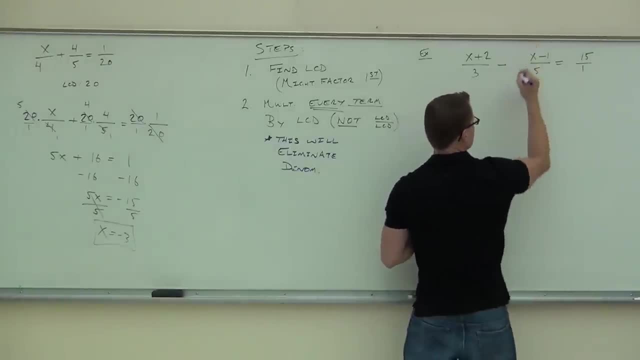 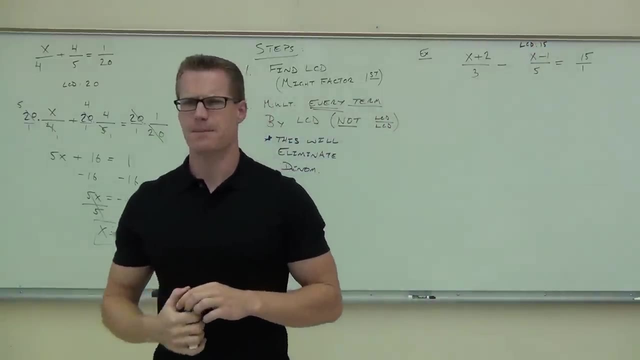 because it doesn't. It's just there. It just happens to be the number, So we're going to take it. Write that LCD 15.. What do we do with that LCD, ladies and gentlemen? Multiply it by the return. Return, Okay. 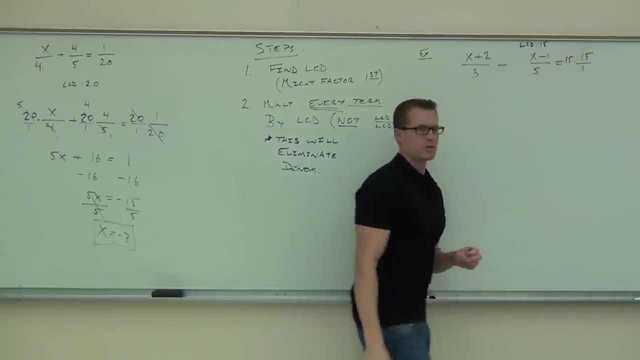 So that means definitely over on the right-hand side. I've got to multiply that by 15.. Hey, tell me something, Are those 15s going to simplify that? No, That's a yeses and some noes. What do you think? 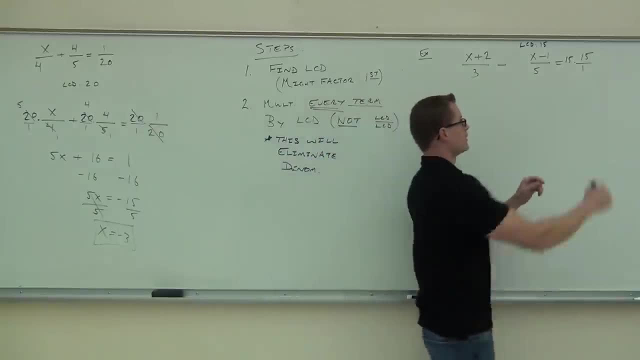 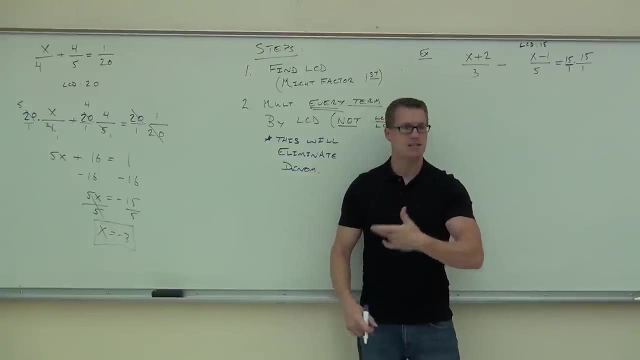 Is it like this? No, No, It's actually like that. Do you see the difference? That's why I gave you this problem. I'm not going to think that you can cross it out. It has to be set up correctly for you. 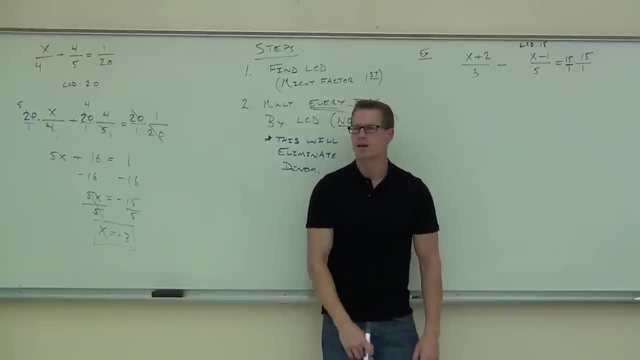 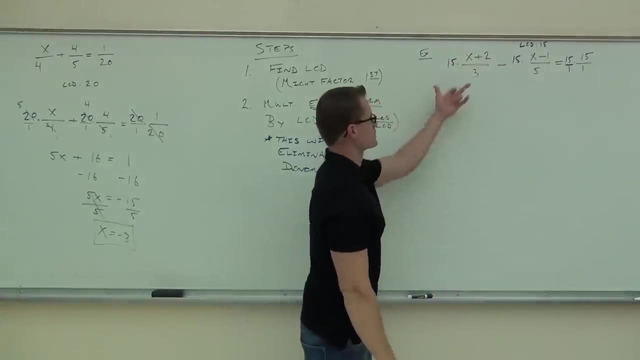 Is that the only thing we need to multiply by 15? No, How many other things? So 15, 15.. Let's make sure this is 1, 2.. All three refractions are multiplied by 15, and we need 15 over 1.. 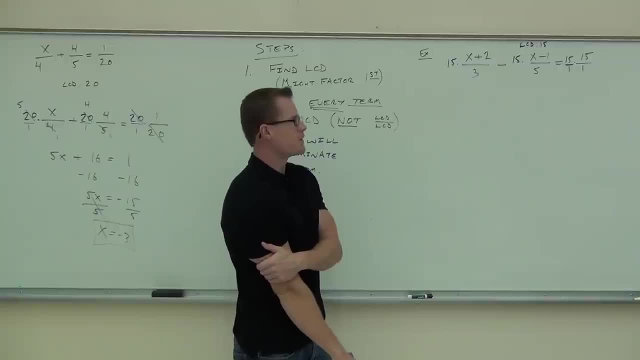 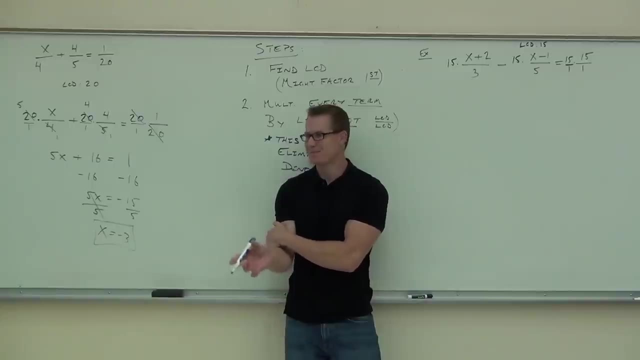 That's fine. One more thing: There's something I'm missing right now On these problems that we talked about: Yeah, Parentheses, What are we missing, Parentheses? Yeah, we're missing the parentheses. We're missing those parentheses. 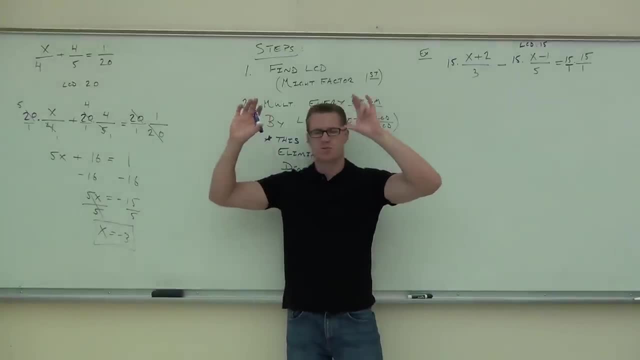 We talked about this. Every time you have a numerator- at least a numerator with more than one term- you need parentheses, because ultimately, we're going to be distributing here, right? So you have to add the parentheses. So we're going to do this. 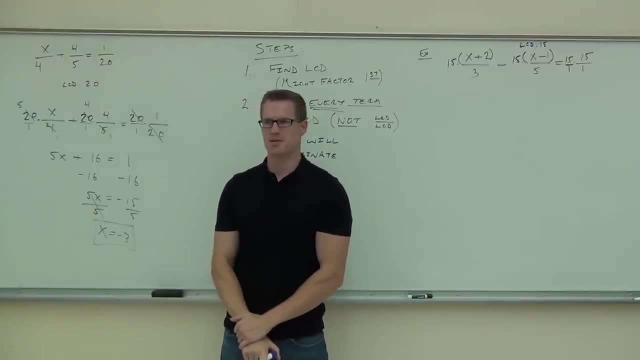 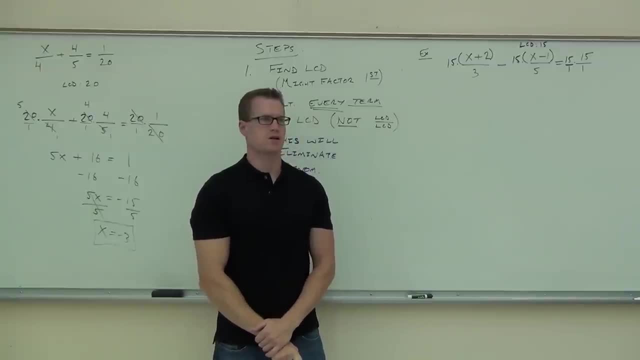 Should we, Should I be distributing here or should I be simplifying here? Should we be distributing? I had two people say two different things. What do you think? Distributing, Distributing, Distributing, What are we trying to do? 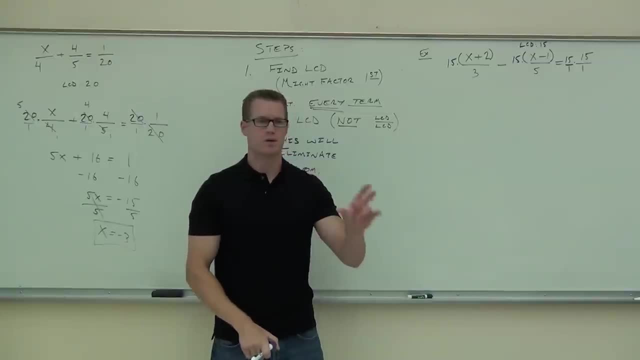 One. Are we trying to make our numerators larger or trying to eliminate our denominators? Eliminate our denominators. Okay, If you distribute, you're going to make your numerator larger and still not get rid of your denominator. Are you with me on that? 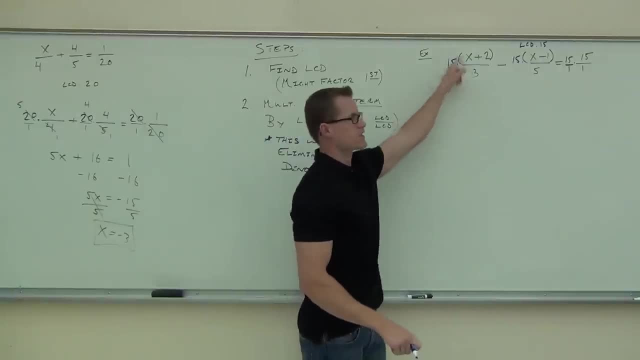 Yes, If you do that, look what you do. You have 15x plus 30, it'd still be over 3, right? How are you going to get rid of that 3? You're going to factor it back out. 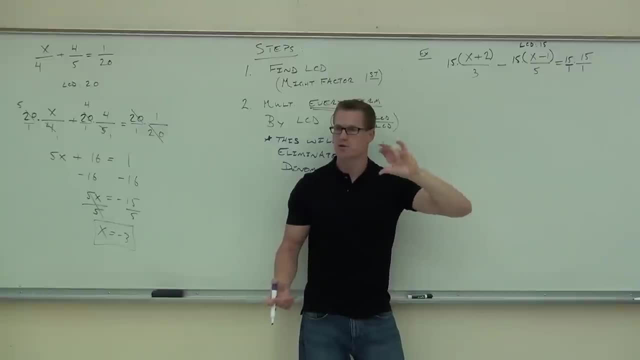 You're going to factor it back out to exactly what you have right here and then simplify it. So if you distribute now, you're wasting two steps. You're wasting distribution and you're wasting refactoring. Get exactly the same thing you have right there. 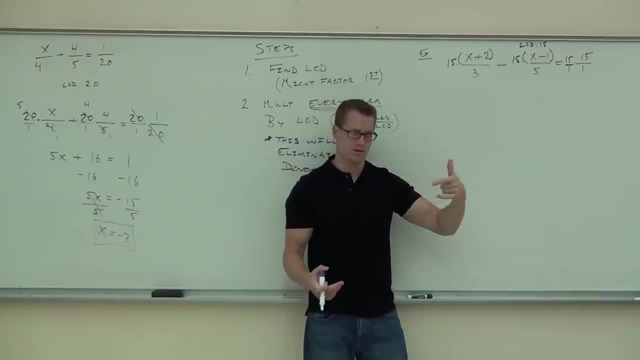 But this is why I have you think of this in class, right, That way, when you get home, you're not like, oh, what do I do now? So we don't want to distribute. Remember, you're trying to get rid of denominators. 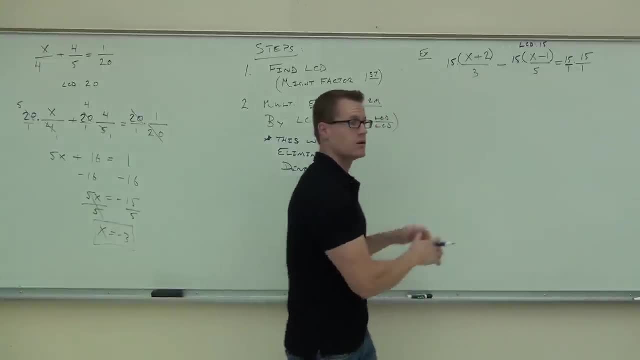 That's what you're trying to do, So do it as soon as you can. That's right here. So don't distribute now. Eliminate denominators now. Do you see that We can eliminate the denominators now? This really is 15 over 1.. 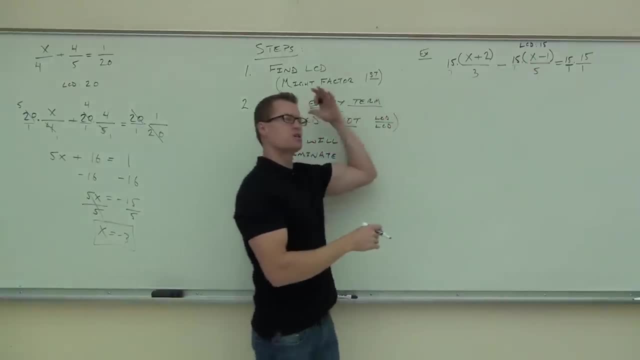 This is 15 over 1.. That's 15 over 1.. We have the same situation we had over here. It has to work this way because we're using our LCD. The LCD combined the factors of our denominators, so they must go into it. 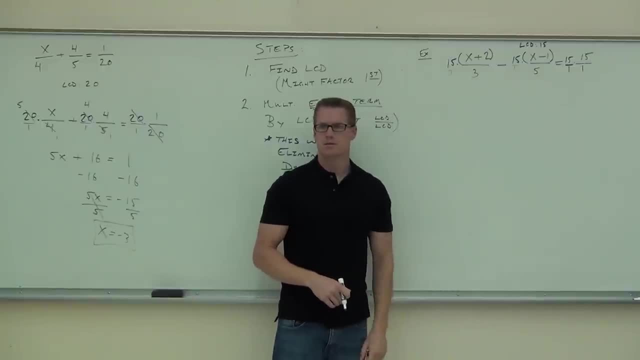 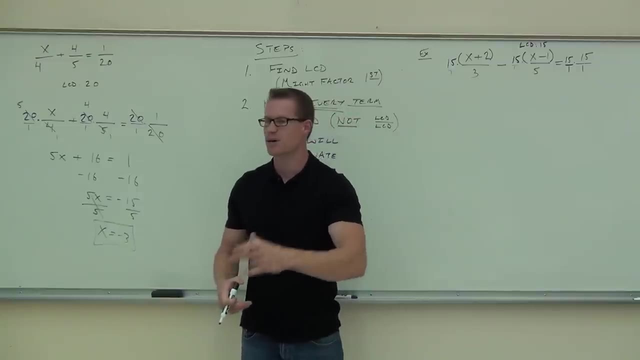 What goes into both 15 and 3?? What goes into both 15 and 3?? Oh, 3 does. That's it. It has to work right. 3 has to go into itself, 3 has to go into 15, because that's how we got 15.. 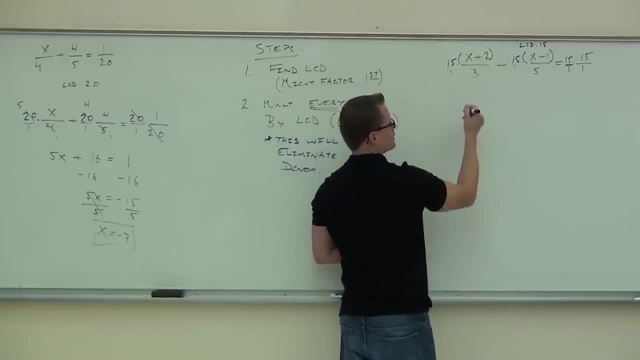 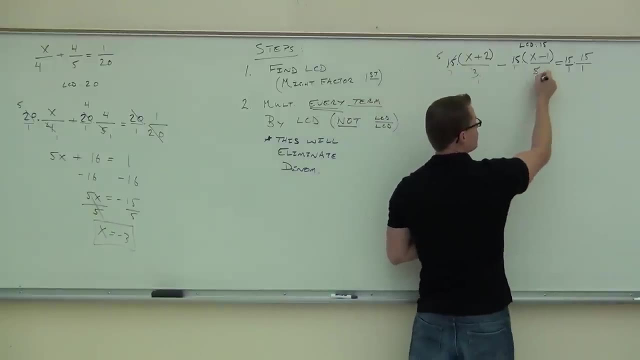 So we're going to cross out the 3 and put a what And 1.. We're going to cross out the 15 and put a what, 5.. And the 5. 5 goes into 5 one time. It goes into 15 three times. 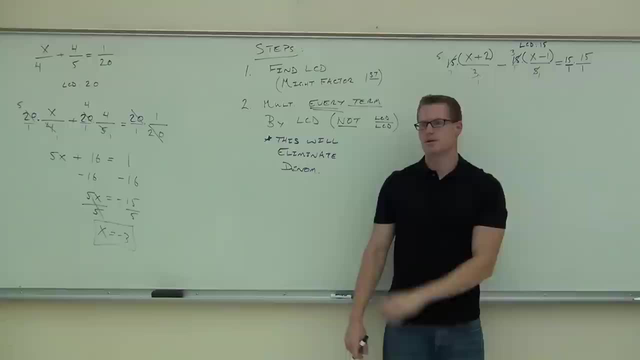 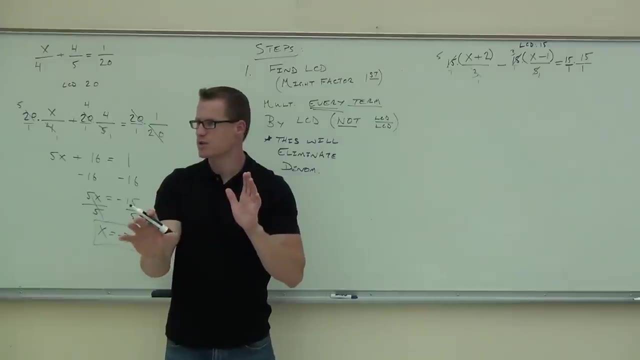 Again, do these 15's simplify? No, no, No, we can't do anything with that, So we're going to continue. We're not going to distribute right now. We're going to just rewrite the problem, just like you did with addition, subtraction. 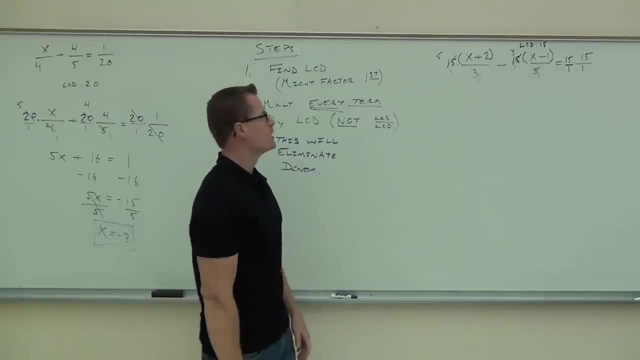 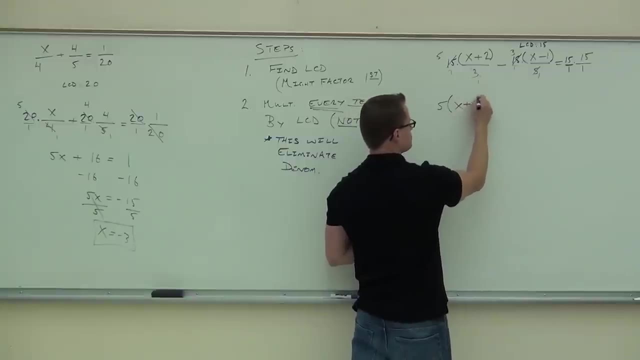 We don't distribute because I can't have you miss negatives or things like that. So we're going to say, okay, We've got this 5 here and we have the x plus 2.. By the way, nod your head if you're okay on getting the 15. 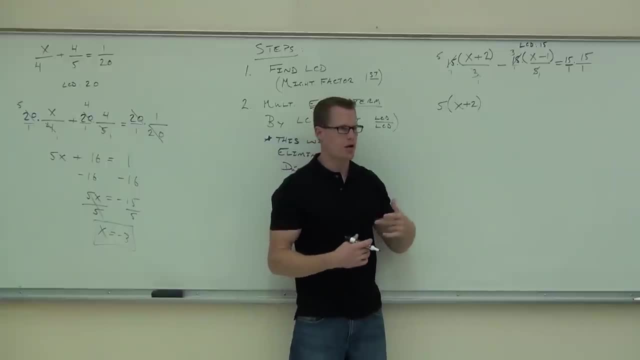 and using it appropriately, just like that. Are you okay on why we're not distributing right now, Why we're not distributing up here? We want to simplify that first. That's the main goal. What's the next thing I'm going to write? 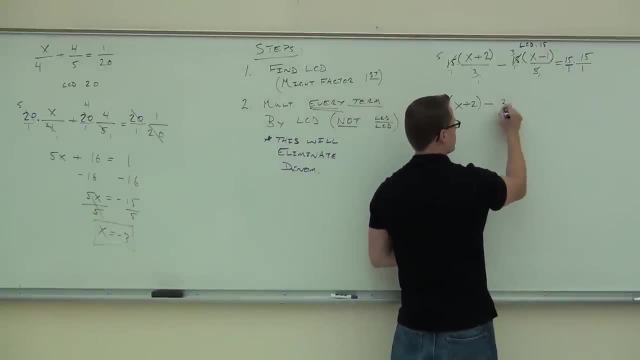 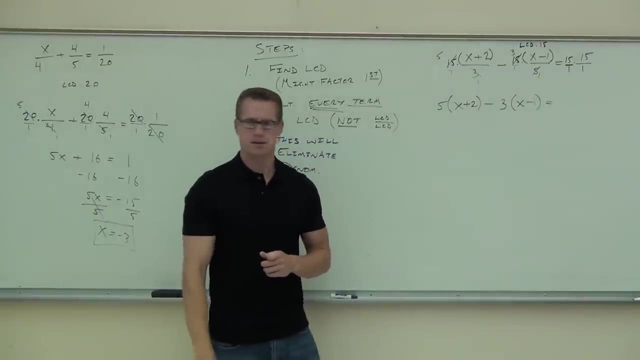 Minus. Okay, great, We can't forget about that. And then there's 3, and then there's a x minus 1.. On the right-hand side of our equation, how much do we get? Good, Do you notice what's going to happen here? 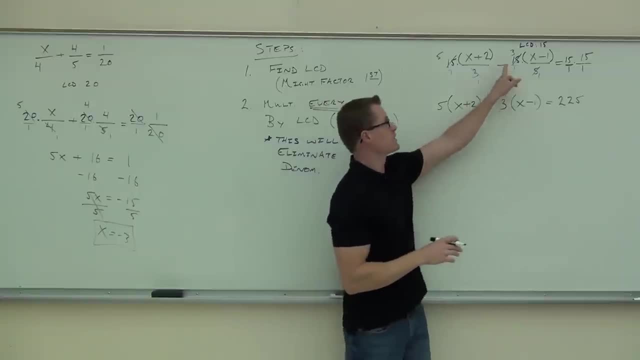 and why I can't have you distribute until this step. If we distribute up here with that 3,, some people are going to forget about that minus right. They're going to give me minus 3x, minus 3, when in fact what we're going to get is minus 3x. 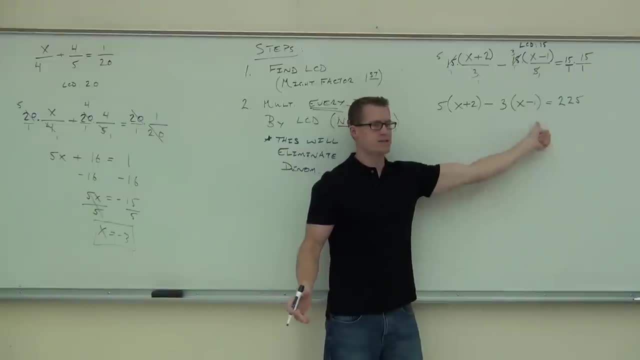 Everybody's going to get that part. Everybody always gets that part right. It's this one, the second one, that's important because that's going to change it, The value of your final answer here, So that negative that's going to distribute. 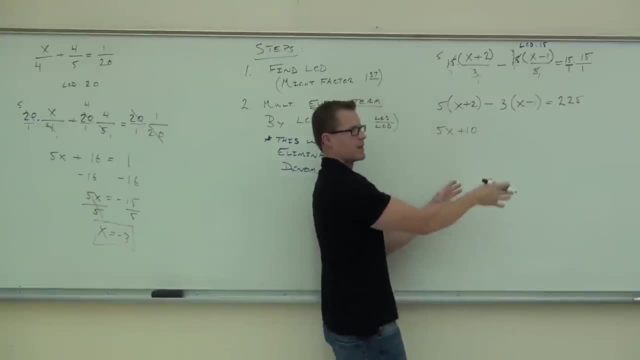 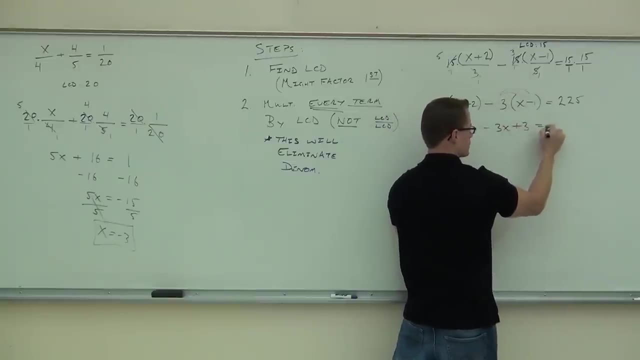 We get our 5x plus 10.. No problem there, That's an easy one Minus 3x. but then, sure enough, we're going to get plus 3.. And that's kind of the big deal If you get minus 3 there. that changed everything. 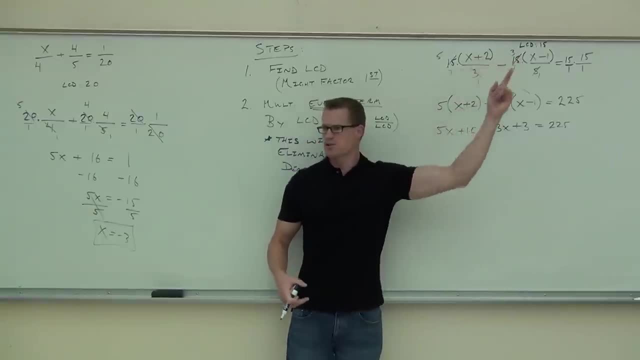 Okay, hey, we've seen things like this. This looks a whole lot better than that. one right No fractions, We just have something simple. This is like pre-algebra stuff. This is pre-algebra level. right Here it's combine like terms and solving basic equations. 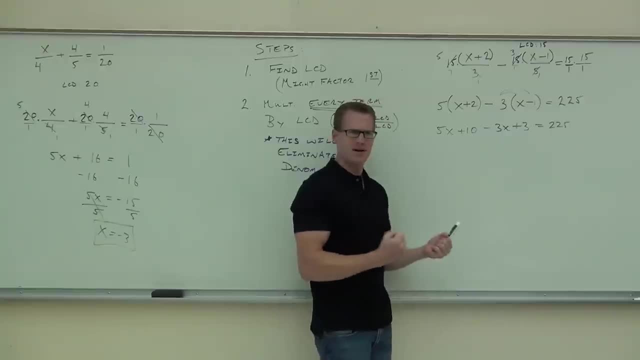 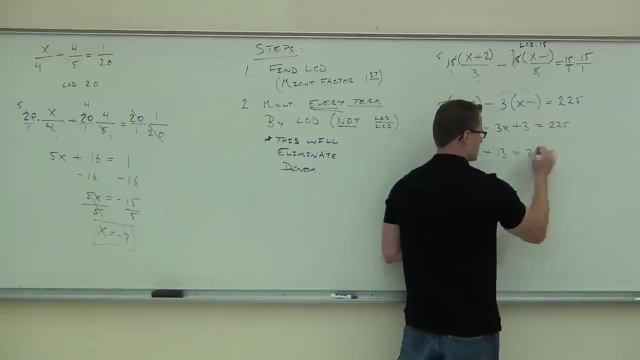 What do you do? Just give it away. Just give it away. So we combine some like terms. We get our 2x plus 13.. Subtract that 13.. We're on the home stretch. now. What is that? 112 or 212, sorry, 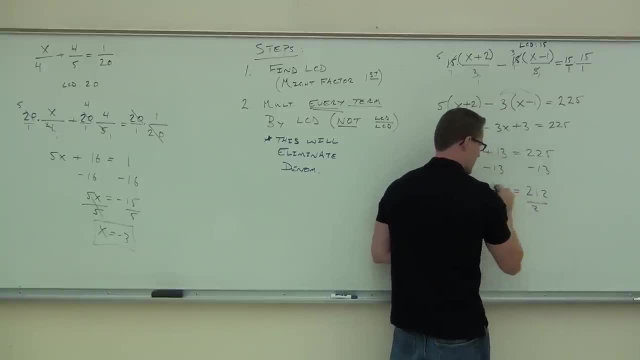 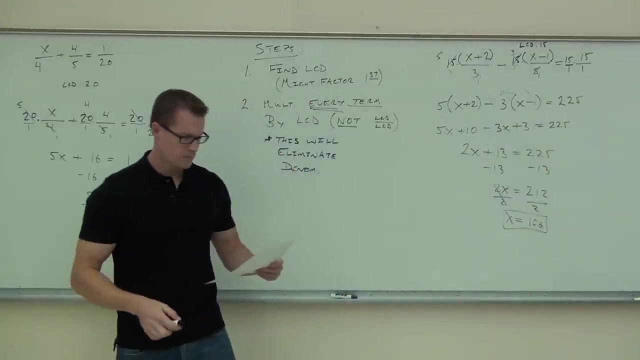 112.. Last step is always to divide. So when we divide it looks like we're going to get 106.. I think it is okay. THEADEUTIC GUITAR, Would you raise your hand and feel okay on doing a problem like this? 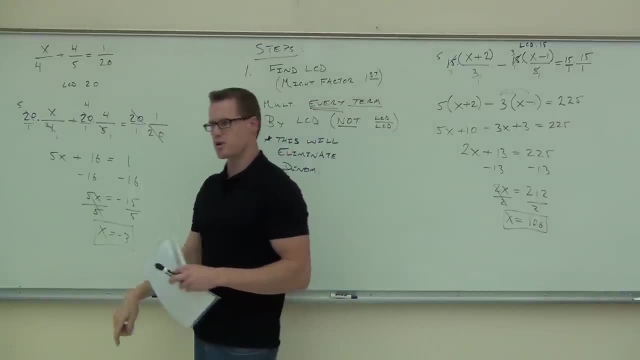 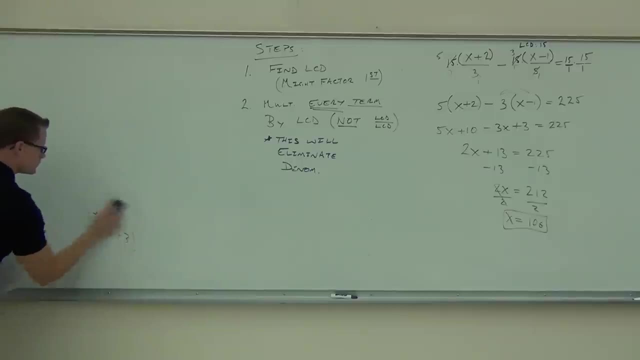 Good, I'm going to give you one to try it on your own. It's similar. Just make sure you go through this process. okay, I want you to try it once before we go any further. It's a long-term problem. 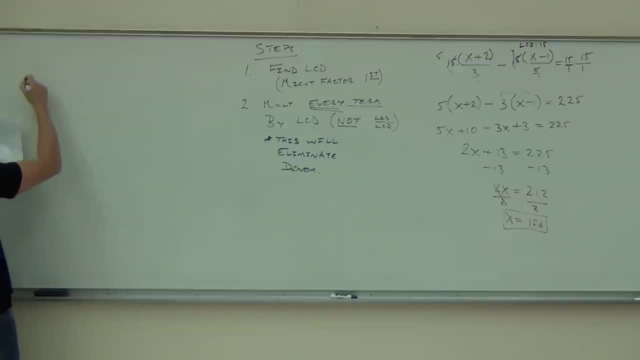 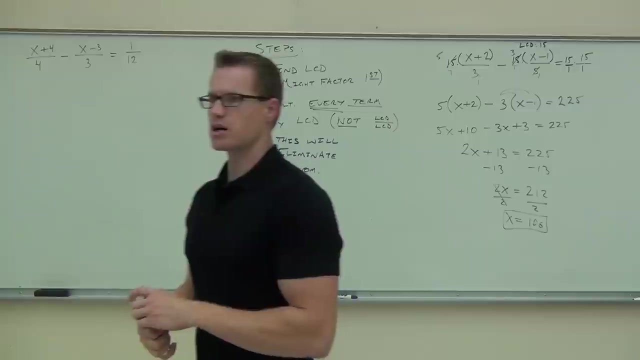 You want to try it once before you go any further? Right, We're going to go through this process, So go ahead and do that one and you do everything that we just talked about. So there's no factor involved here on the denominators, because they're just numbers. 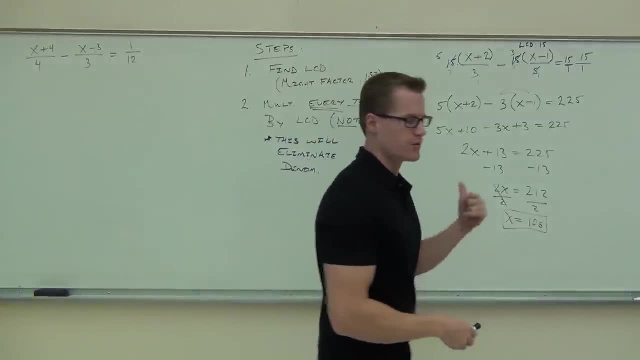 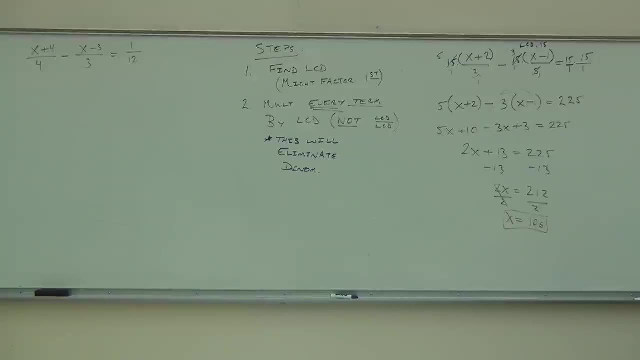 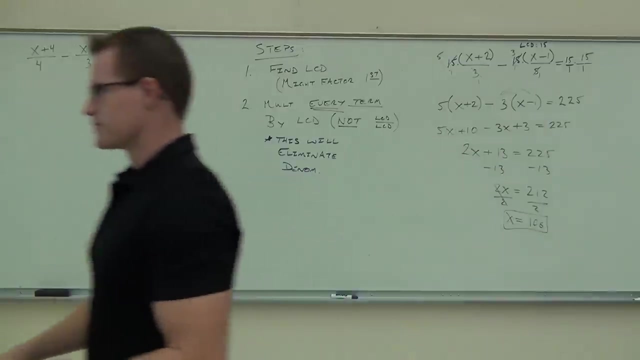 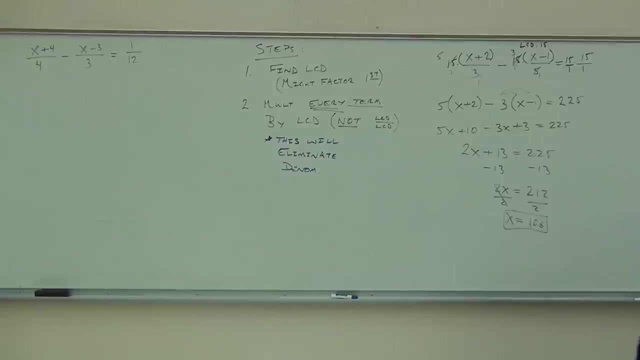 But find your LCD, use that, use parentheses where you need to and figure out what that's going to be. And again, if you are using, let's say, the number 1, you're not going to be able to find. 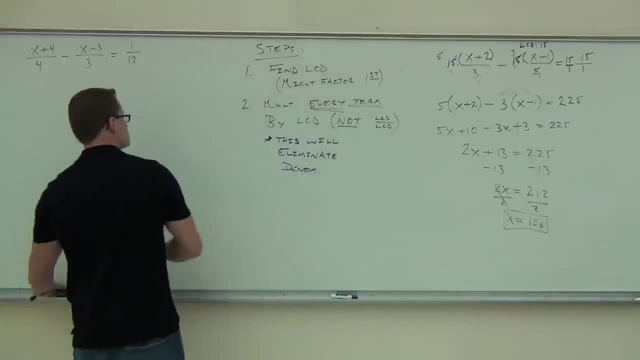 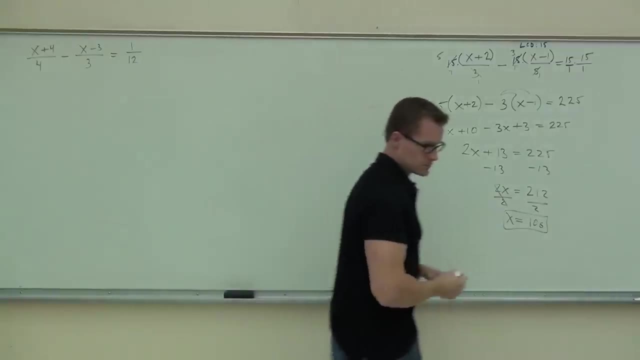 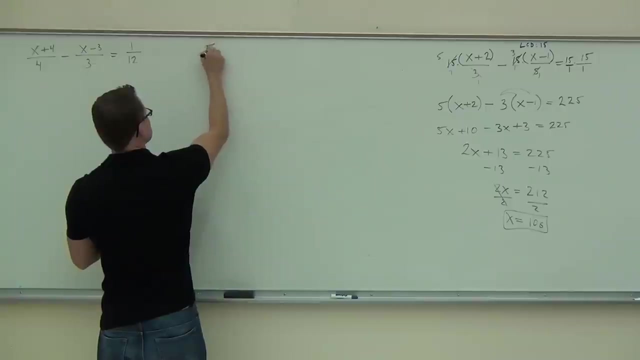 it. You're going to try and find it. Now, what's the best way to do that? Well, go ahead and run through this and see what you're doing there. So go ahead and do the math. So if I just want to do the math, 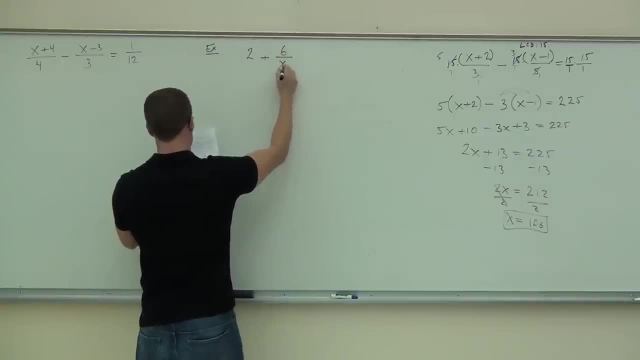 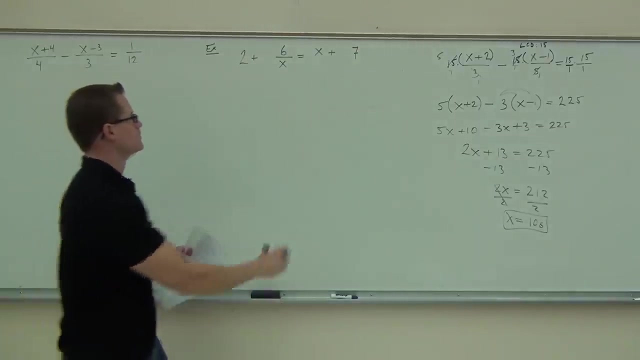 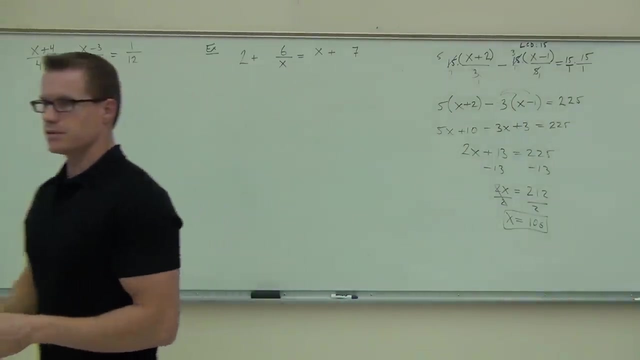 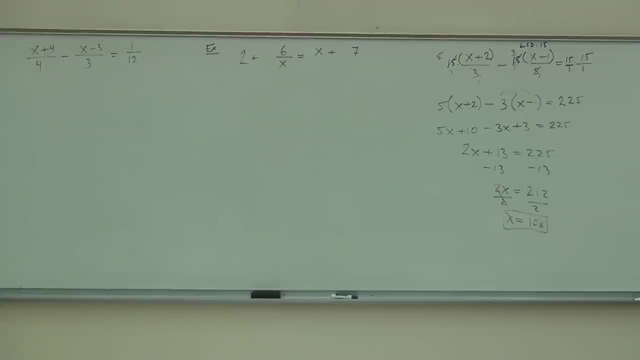 So if I'm going to do the math, then I'm going to do the math. Thank you, We should be almost done with that first one. Hopefully you found the LCD. Hopefully you multiplied that appropriately. Definitely need some parentheses on that problem. 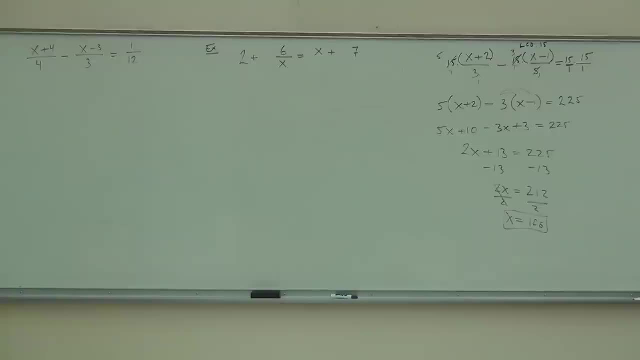 Distribute correctly and then solve the basic equation. So, first thing, what did you find for the LCD in our problem up here? Are we trying to find common denominators or eliminate denominators altogether? Which one Eliminate, Trying to eliminate? 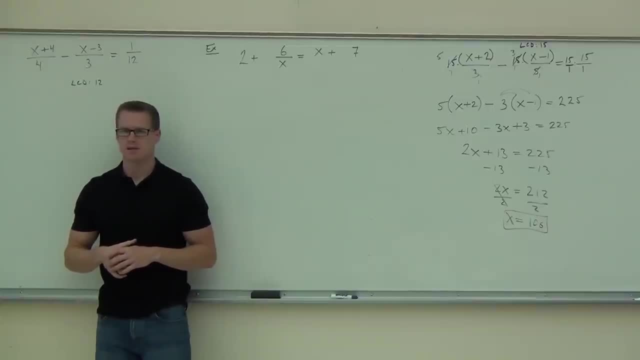 That's good. Ladies and gentlemen, when you get to your test, you're obviously not going to have me telling you what to do on this problem, right? I'm not going to say, oh, you need to eliminate your denominators. 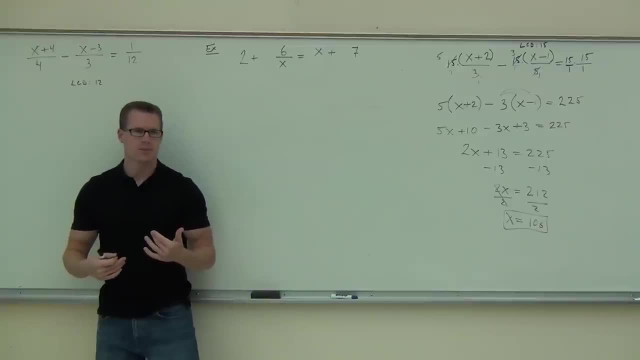 You're just going to have to know What tells you up here. Everyone should know this from this point. What tells you up here that you can eliminate denominators rather than just find a common denominator? Equals Good. That's very good. 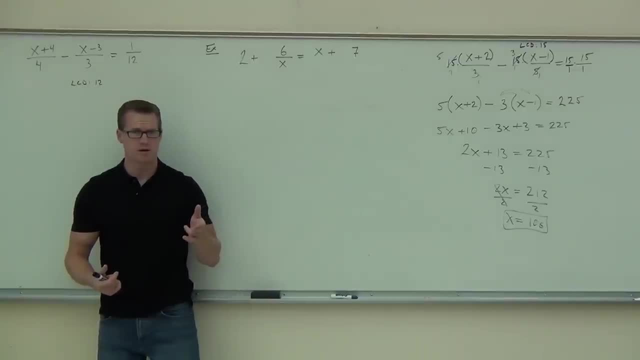 So if you have the equal sign, you know you can eliminate. Are you with me on that? If you don't, can you eliminate them? No, Just find common ones. That's the difference. Okay, so we have our LCD. 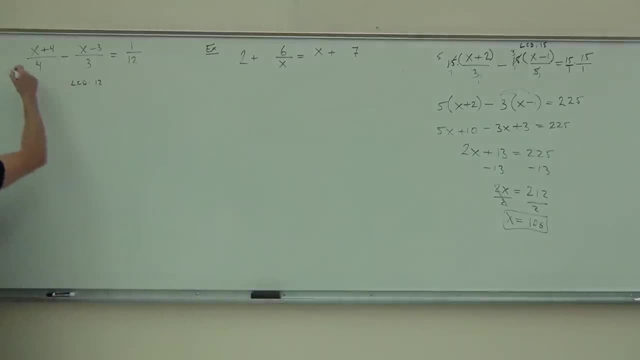 We're going to be able to eliminate denominators. but in order to do that, you have to multiply every term by the LCD. That's both sides, every term, Not LCD over anything besides one, because we're trying to get rid of things, not make it worse. 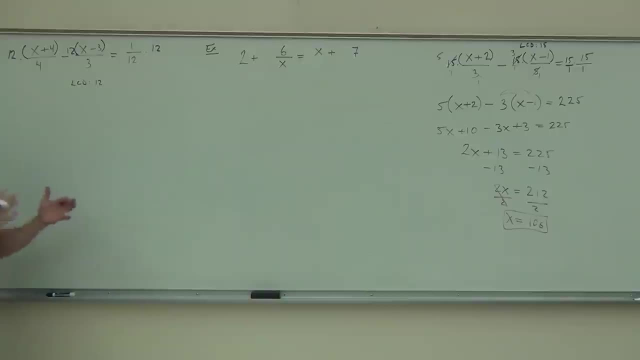 We definitely have to add some parentheses. I hope you put that. And now we get to do the fun part, which is simplify some stuff We don't want to distribute now We want to get rid of things. So the 12s. 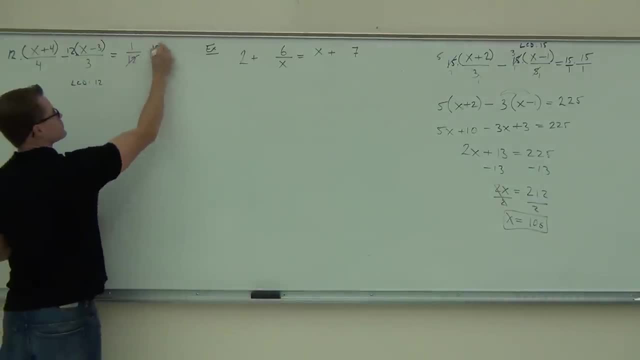 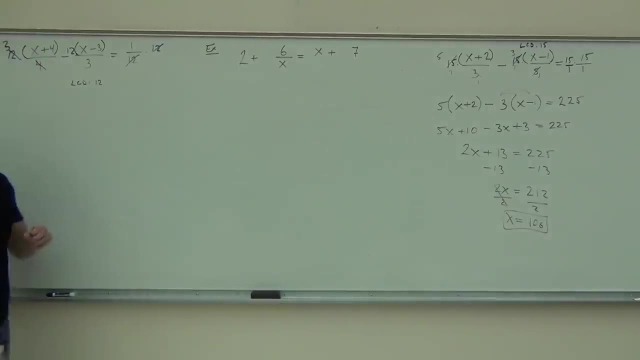 Oh, you know what? I had just been there. 12s are gone, The 4 and a 12,. well, that simplifies to a 3 over 1, because the 4 is a 4 one time and a 12 three times. 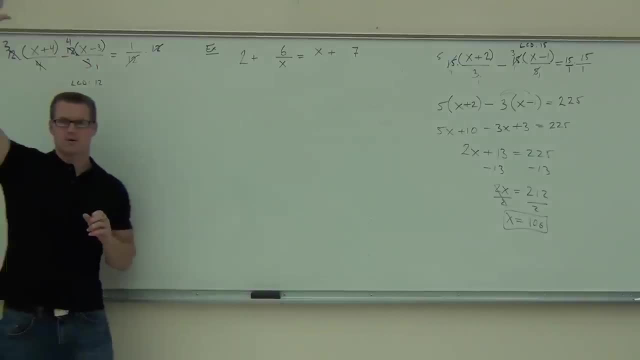 3 and 12, that's going to give you that 4.. How many people made it that far? Good, Fantastic, We continue. I'm not going to distribute it yet. I'm going to write it just to make sure I see what's going. 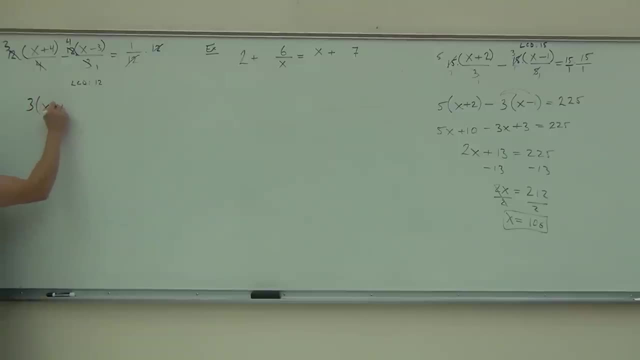 on in this problem, We're going to have 3 times x plus 4.. That's the problem. We're going to have 3 times x plus 4.. That's the problem. Minus 4, x minus 3 equals 1 over there. 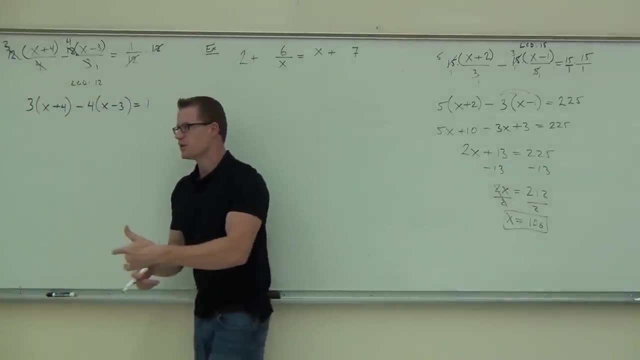 After this, really, I mean this shouldn't be too bad, right? This is just distribution. combine some like terms and solving the basic problem without even x squared. That's nice. So here we'll distribute. We'll get 3x plus 12.. 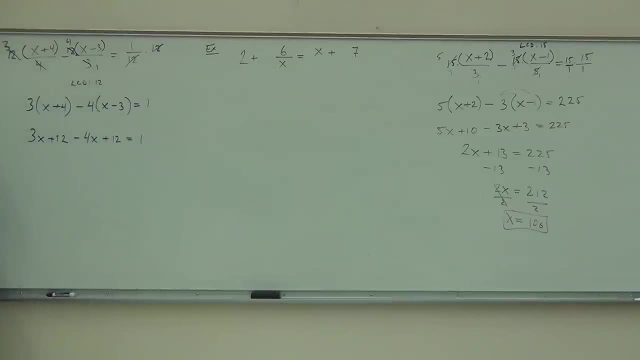 4x plus 12 equals 1.. So far, so good. Good, All right, We continue. We're going to combine some like terms. If I combine like terms, what do I get? Perfect, Keep going, Subtract 24.. 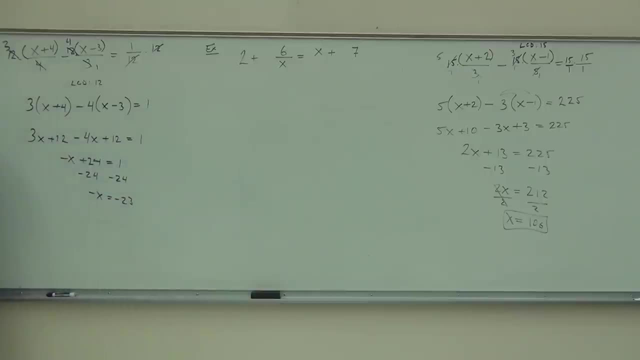 Negative x equals negative 23.. If negative x equals negative 23, x equals how much? So you can divide by negative 1 here or just switch both sides. That's fine, We're going to be positive 23 out of that. 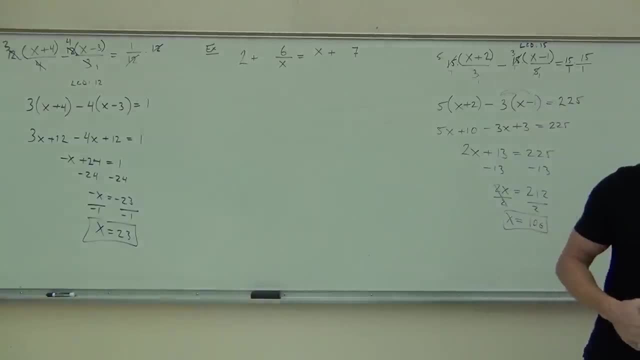 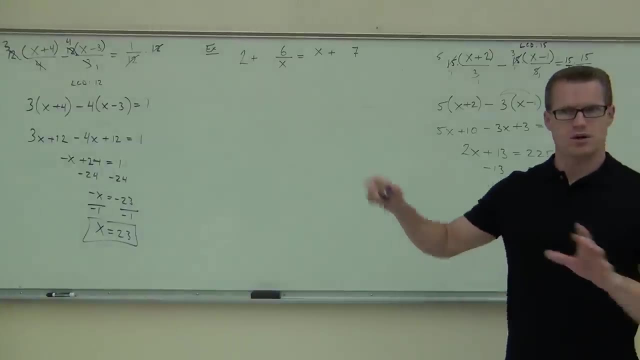 Now on the next one. The next one's the first case where we have something a little bit different here. What do you think? maybe the first thing that we should do is on this problem. Okay, That might be a good idea to make them all. 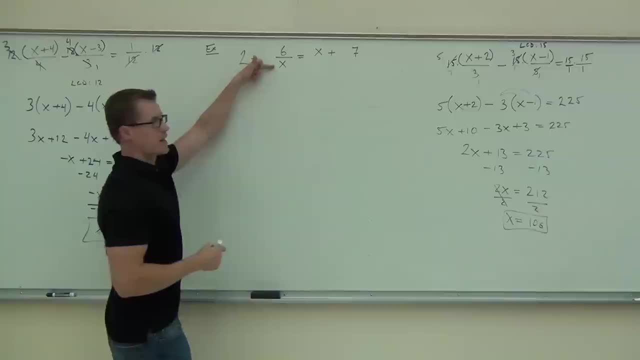 into fractions. That's great. So here we have 6 over x. That's awesome, but that's our only fraction. Let's change them all into fractions. In order to do that, really, we just have to put this over 1,. 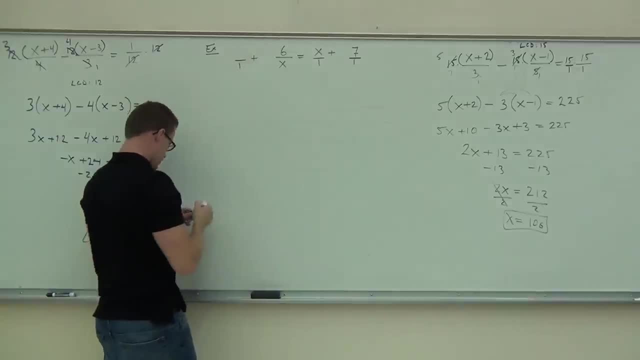 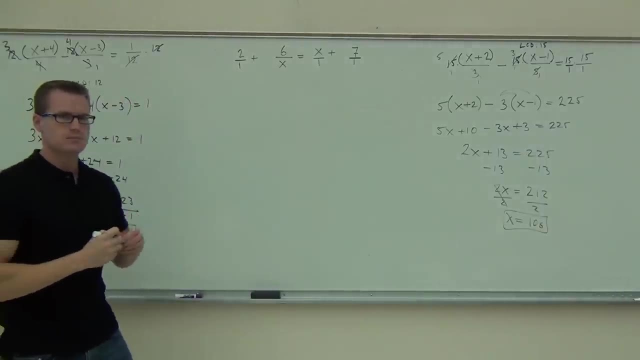 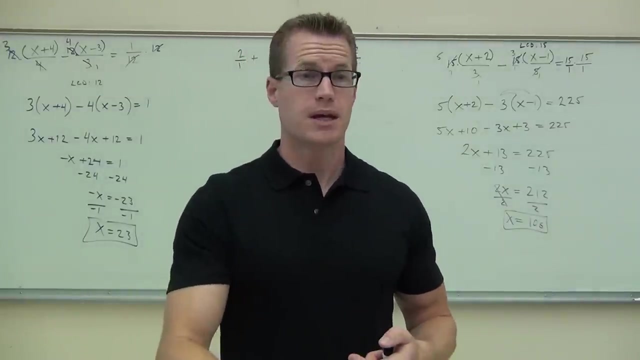 over 1, and over 1.. Take a look up there. The next thing for you to do would be factor- There's nothing to factor- And then find your LCD. Can you tell me what is the LCD in this problem X? 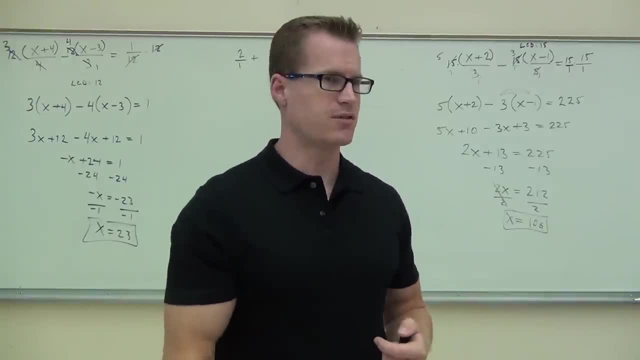 Do you notice how the LCD has nothing to do with the 2 or the second? There's 7 up there. Do you guys see that? That's one reason why we write them as fractions first, so we get those numbers out of our head. 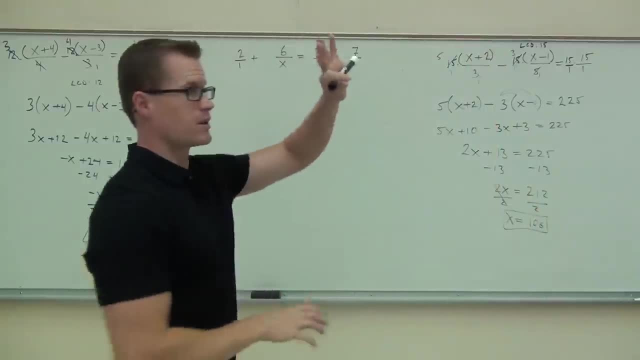 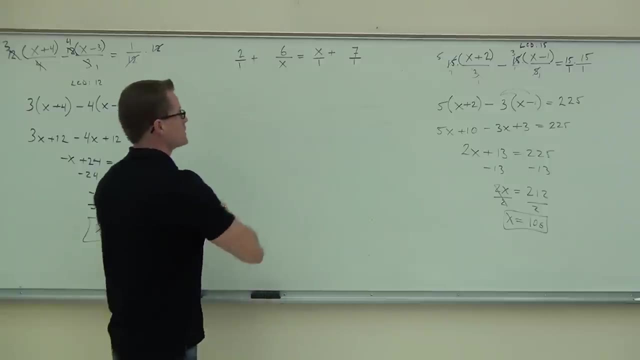 We're just looking at 4 denominators. We're looking at 3 1's and an x. So the LCD: yeah, it's got to be x. Not sure if you're still okay on that. So LCD, yeah, we're getting x. 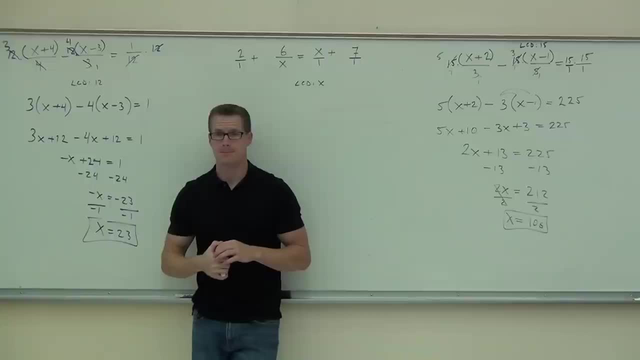 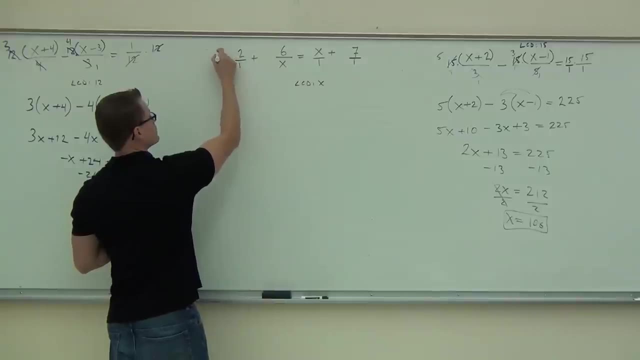 Okay, folks, What do I do with that x? Next step: Every how many terms is that up here? 4. Good, So that means here. That means here, definitely That means here. Oh, don't forget about that one. 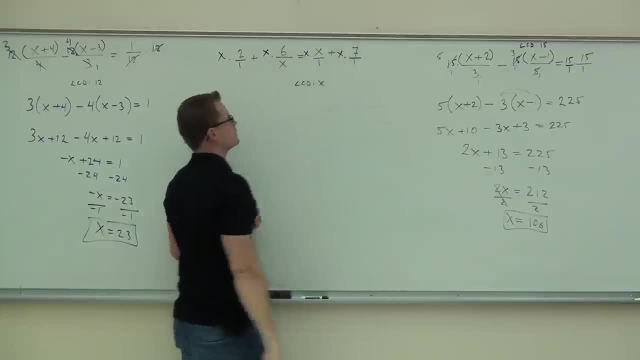 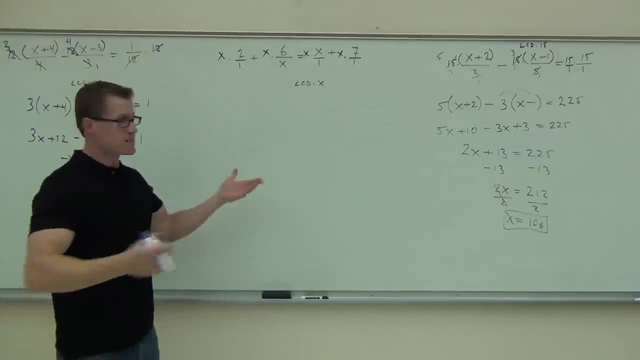 And that also means I can do it on either side. It doesn't really matter Here. So 1,, 2, 3,, all times x, Not x over anything, X over 1.. Maybe x over 1.. 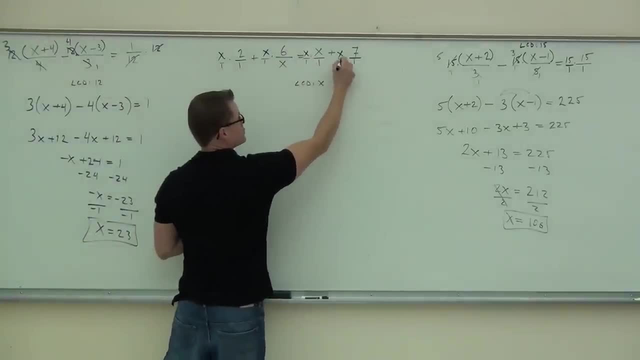 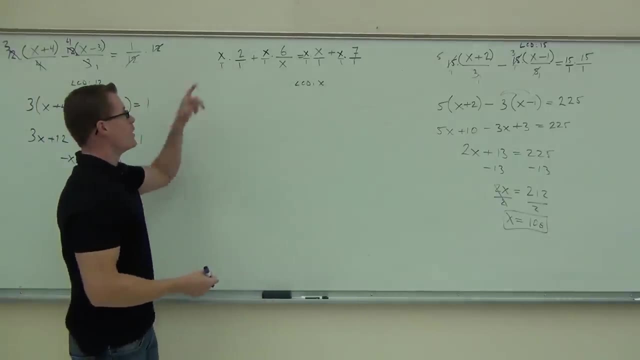 You can put that if you like, But it's certainly not like x over x or anything like that. This should be an okay problem for us to do. Let's figure out. Let's figure out what we're going to have On the first fraction. what do I get out of that? 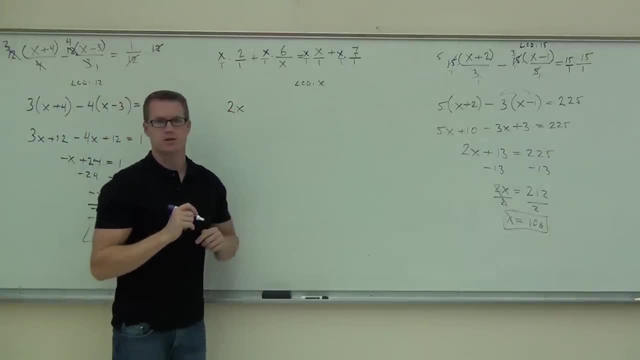 Well, that's not bad. How about the second fraction? How do you get in the 6?? Okay, X's are gone. Yeah, that's absolutely right. That's why we did that step right. That's why we did this whole process is to get rid of that fraction. 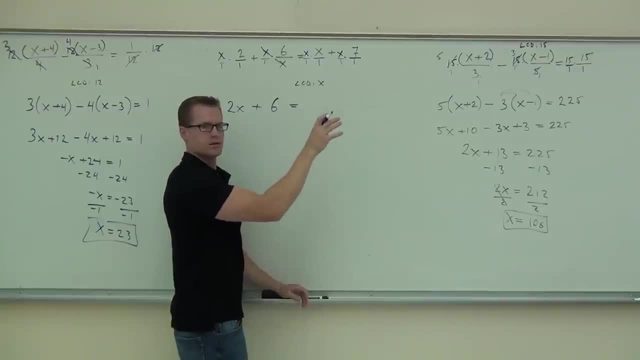 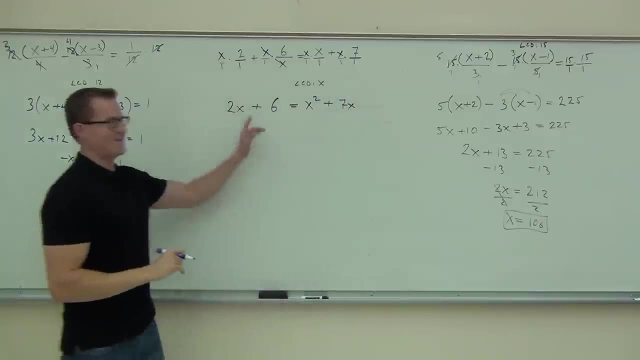 6, is it Equals on the right-hand side. what are we going to get? x squared? Good Yeah, don't forget about the exponent. That's fantastic. And then how much? 7x? Oh, oh, do you see it? 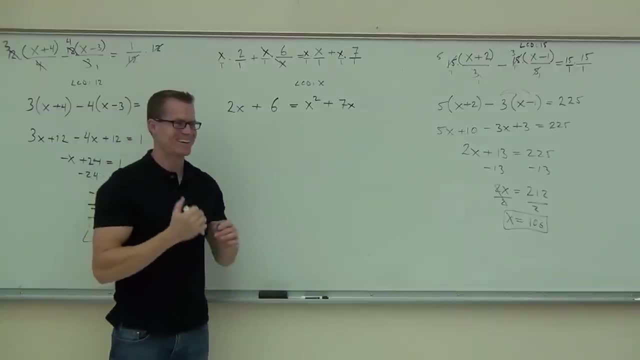 Look it, What is that? We've seen that before. What do you do when you have something like that? First, we get class Right here, Right here, Right now. Okay, You have an x squared up there, right, Can you solve this one like you did that one? 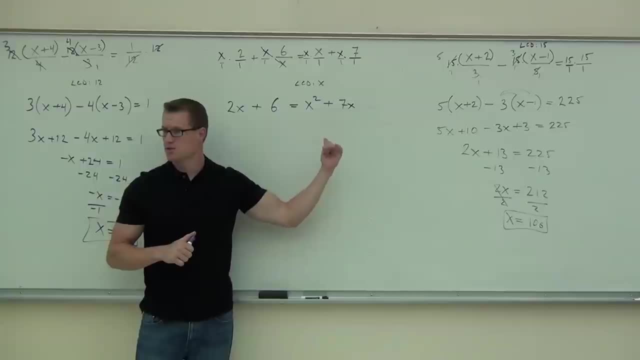 Totally different problem, right? We found out that when you had the x squared, you remember the diamond problem. Yeah, That's why we learned the diamond problem in the first place. Solve a problem like this When you have the x squared, it said. 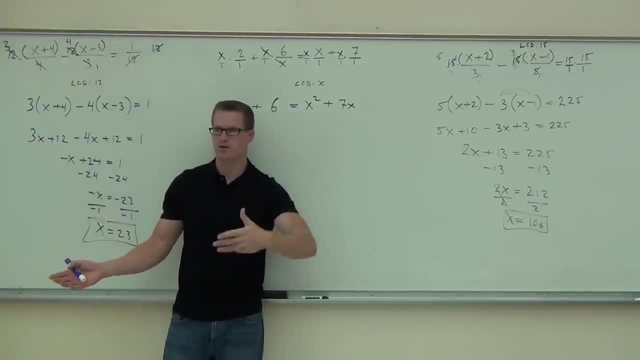 hey, if you don't remember this, go back and watch that Man that was. it's good. Nine parts or 11 parts. Every part was better than the last one, Part 11,. oh yeah, And it said: get everything to one side. 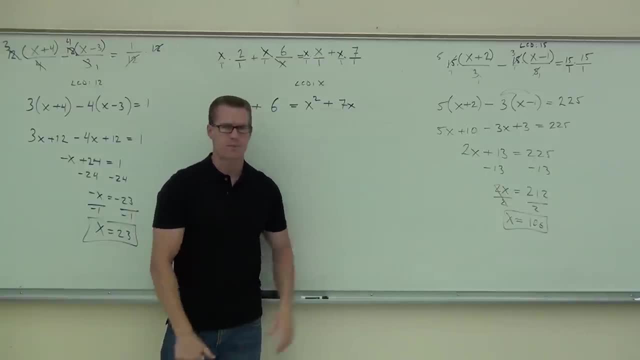 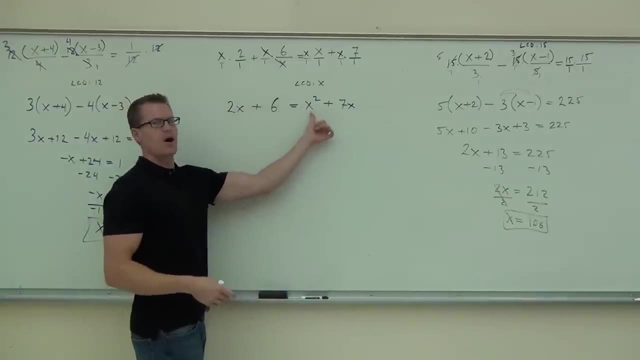 Zero on the other side. that way, you can use a zero product property factor and solve it. I'm not going to ask you about that, because we've covered it so many times and that's what we'll do. So we have our x squared. let's keep that thing positive. 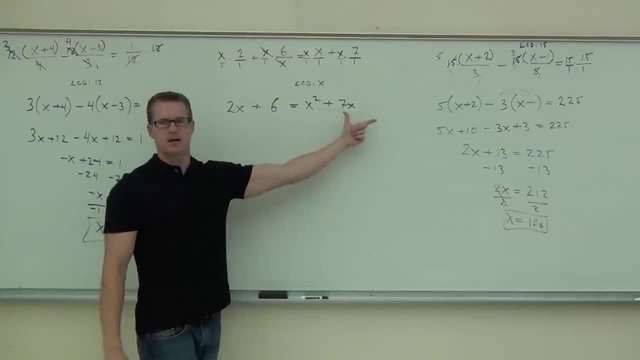 That's already positive. that's great. Get these two on that side. Are you with me on that? You try to go this way. it's going to be very hard to factor, So we're going to go This way. That means: subtract 2x, we'll get 6 equals x squared plus 5x. 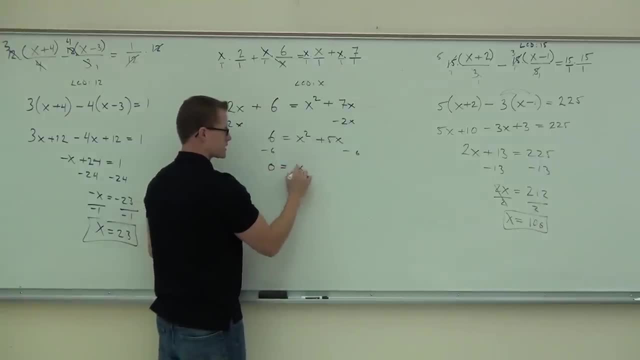 We'll subtract 6, 0 equals x squared plus 5x minus 6.. We've seen things like that for a long time now. You've factored them so many times in your homework. It's not even funny. I mean, you can do this all the time. 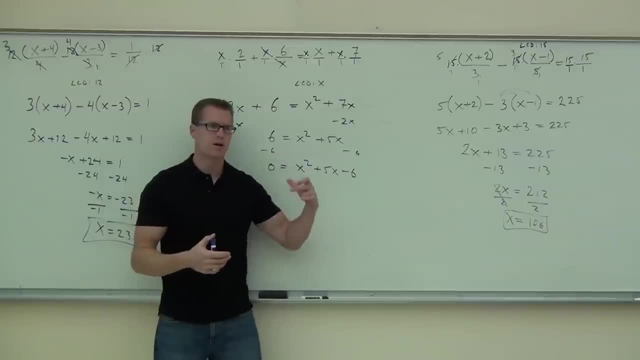 Now we have it equal to zero and we know that from section C.1,. if an equation like this is equal to zero, if an expression is equal to zero, we can factor this, set each of them equal to zero by the zero product property and solve it. 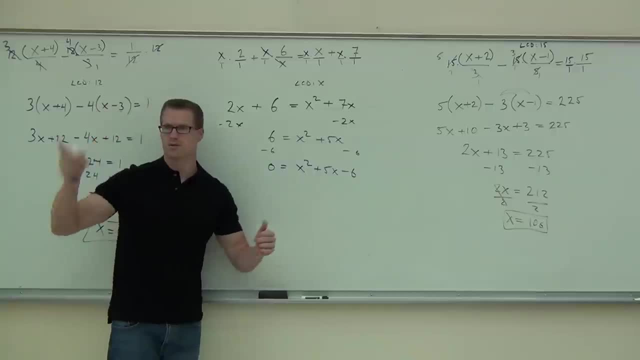 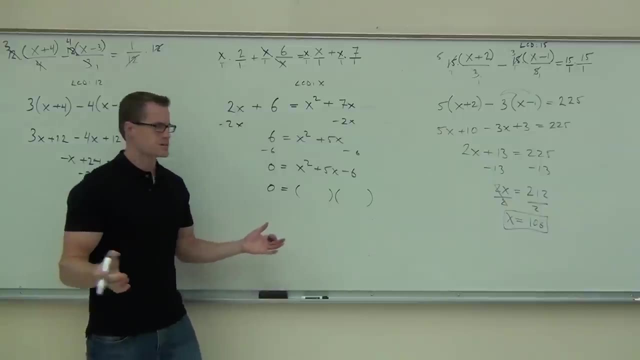 Do you remember how to factor that? Oh, so it should be like in your head, like automatically at this point. So we'll still have the zero diamond problem. No extra steps, that's no big deal. We just have 5 and negative 6.. 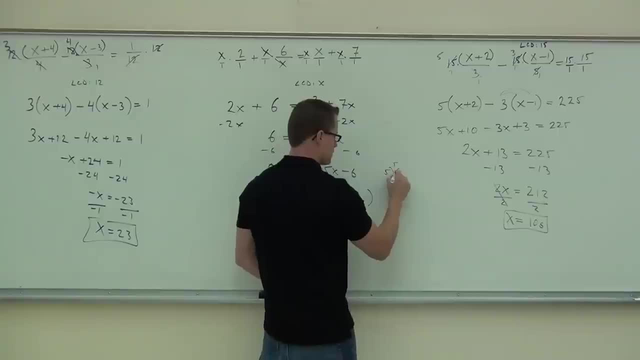 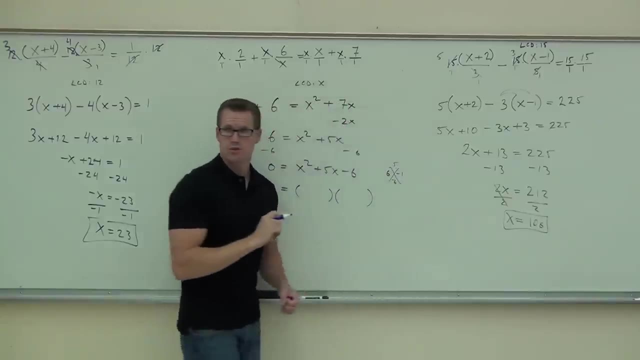 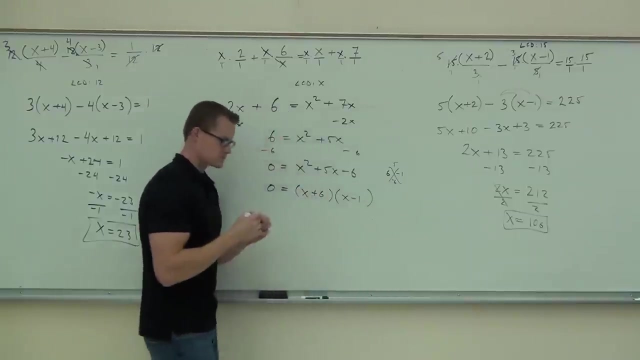 I'm thinking positive 6, negative 1.. That's coming to mind. Were you thinking of those numbers also? So, because there's no extra step, I just do x plus 6, and x minus 1.. Am I done? 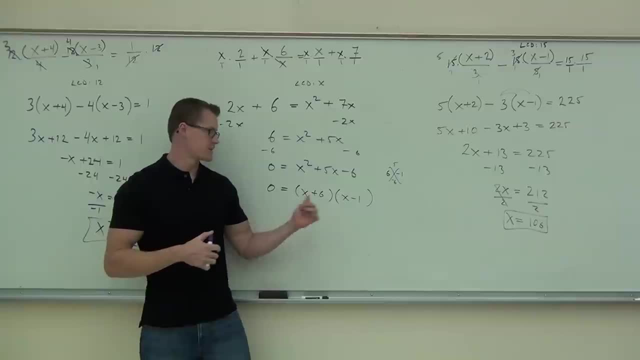 No, I'm close, very, very close. All you have to do from here is set each of these things equal to zero. This is the case where you do that, because it is equal to something right, You can actually solve these. 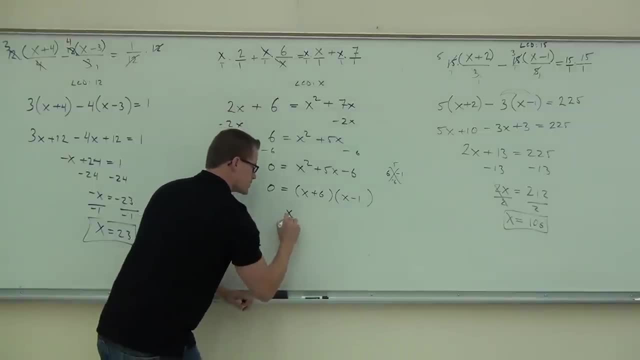 You don't just have to manipulate them, You can solve them. So we'll do: x plus 6 equals zero, X minus 1.. X minus 1.. X minus 1 equals zero. We're going to subtract 6.. We'll add 1.. 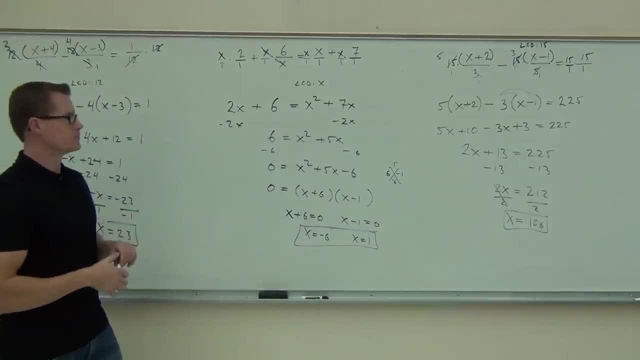 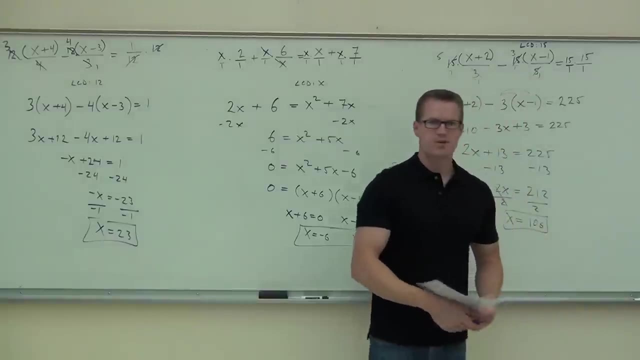 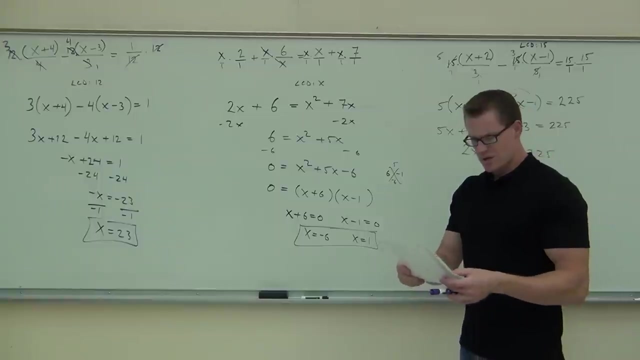 And we're done. Where's your hand? feel okay with that Good, Good deal. Maybe I'll give you one of these to try, and just Right now I want to go and do a couple other ones. We'll do about two more. 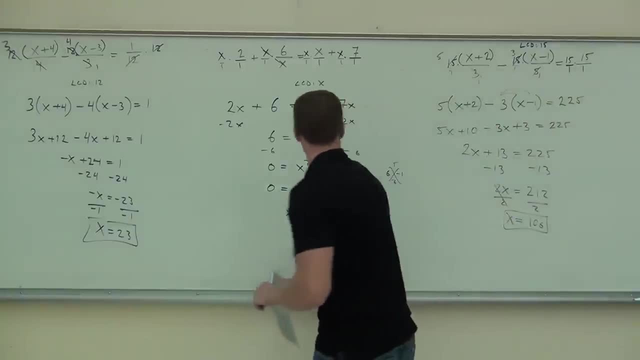 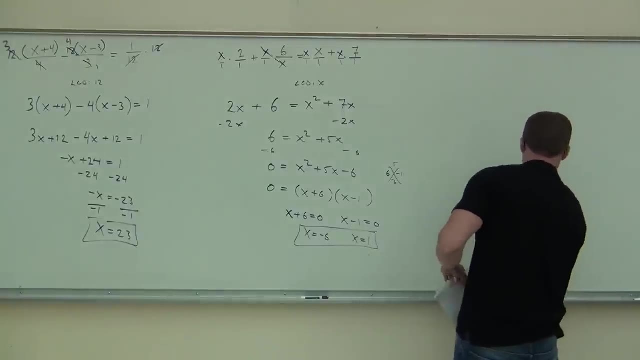 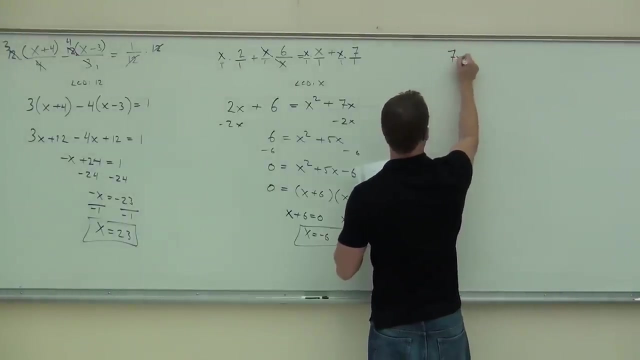 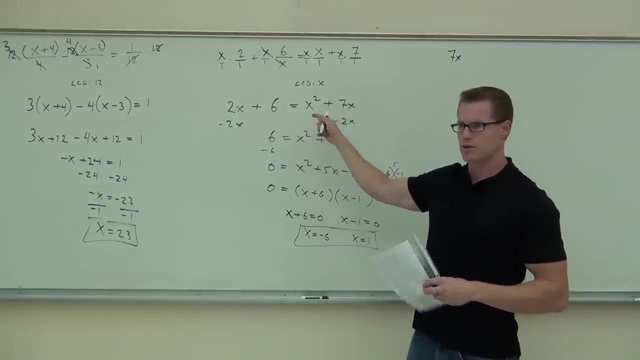 We'll do two together. I'll give you a couple doing your own. Fall in there, Two out of 3.. Do you need one like that to try on your own, Or do you feel good about this? You want one of those? 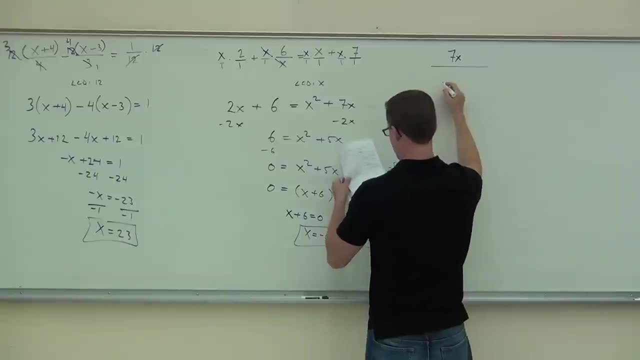 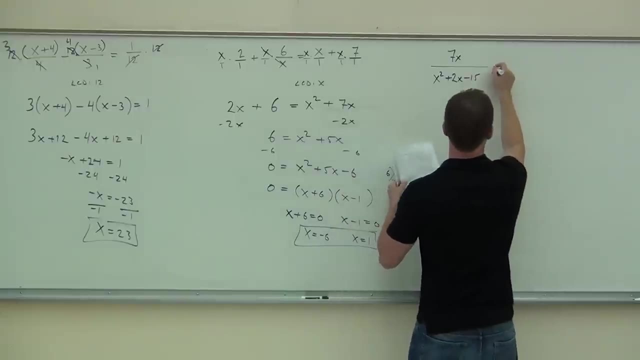 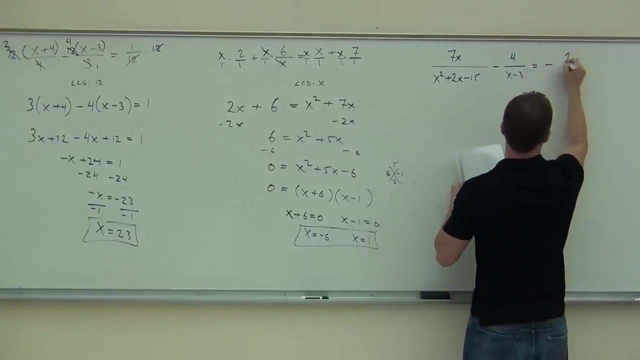 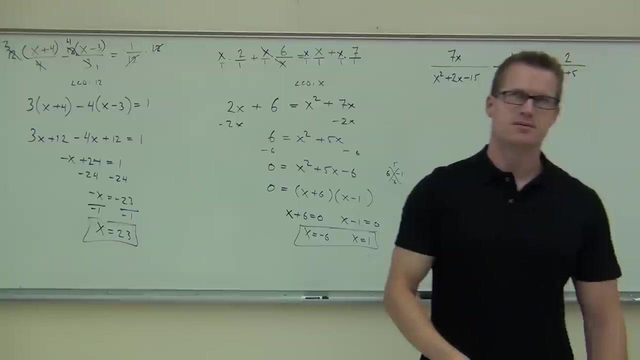 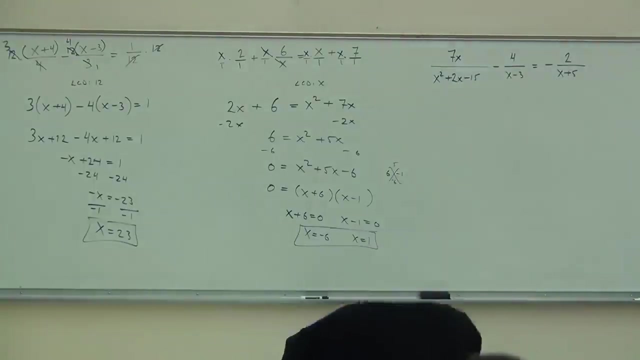 I'll give you one later then. Okay, Do you like it? Yes, Okay, Thank you, Bye-bye. See, it's getting better. it's getting better. Now they look more nastier. whatever, they look more nastier, but they're not going to. 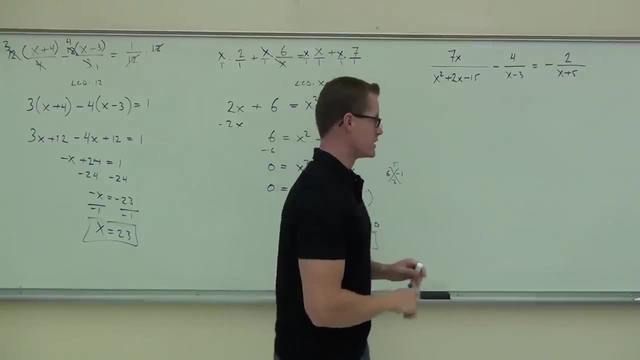 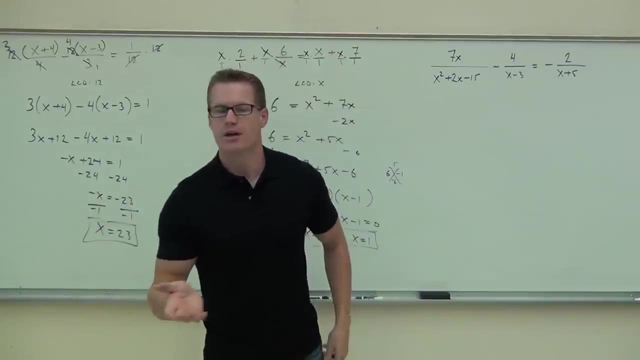 be any different from what we just did, not any different from what we just did. All you have to remember is that you're finding LCD and using the LCD to simplify denominators. that's what you're doing. In order to find the LCD on this problem, though, you have to do something first. what is that? 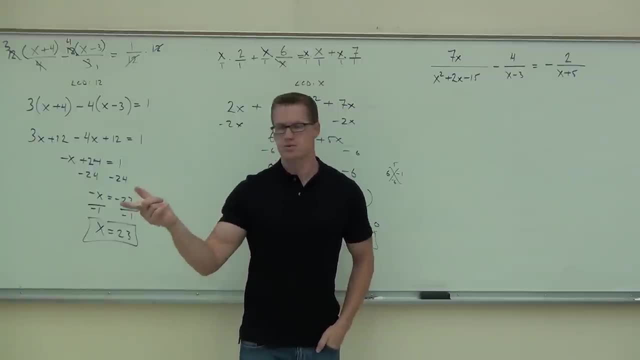 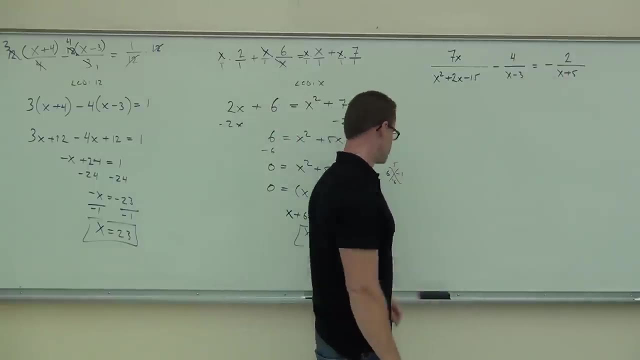 thing first. Then in the first one, Okay, and that means we're going to factor that. So right now, on your own, I'm going to do it on the board. factor that right now. These two, you're fine, they're all right. factor that one. 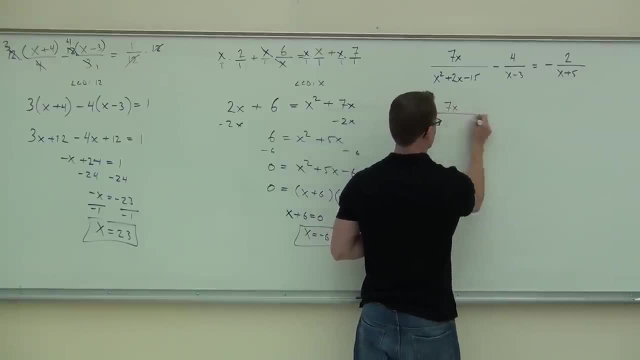 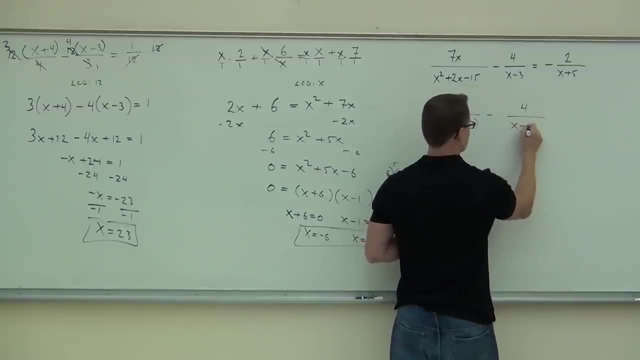 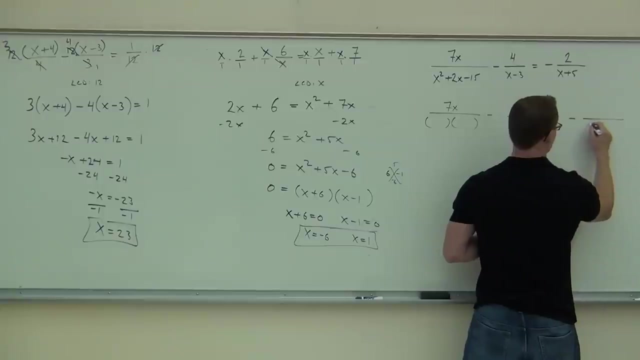 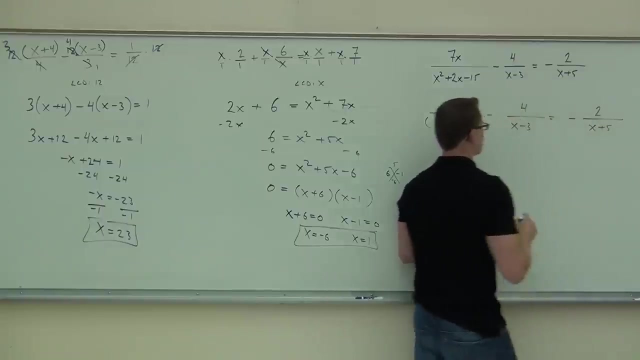 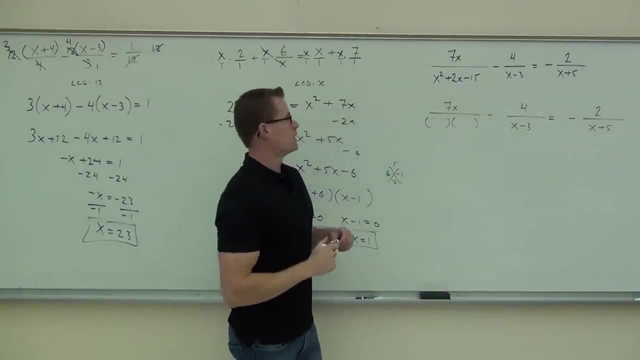 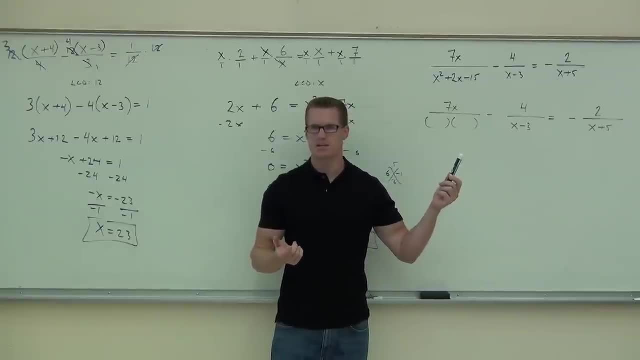 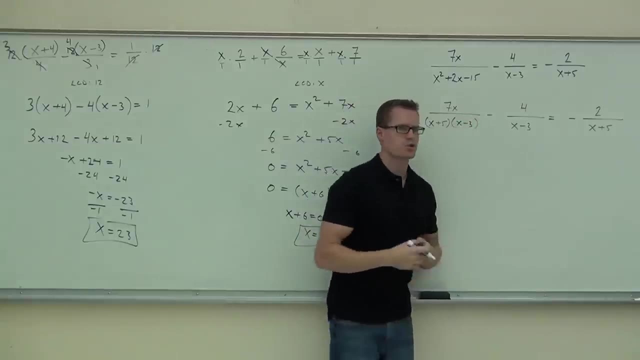 know, the bigger ones got to be positive. Hopefully you've found 5 and 3, 5 and negative 3.. I'm probably going to stop showing you the diamond method on the board, because we've covered it so many times. You know just how to do it. 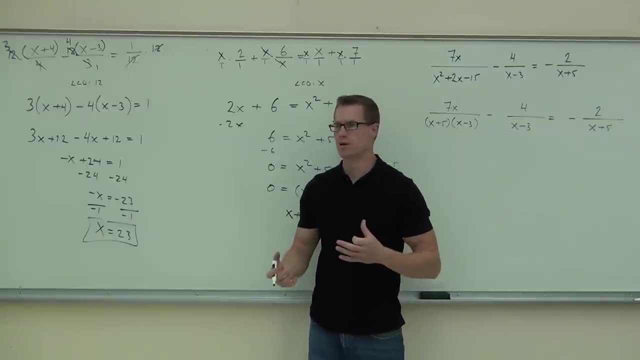 So I'm encouraging you to find the numbers like that. We need to be able to do that on your own. at this point, You can find the x plus 5x minus 3? Okay, Hey, you're also pros of this. 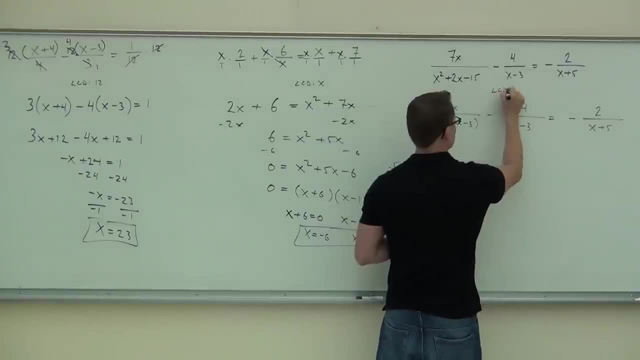 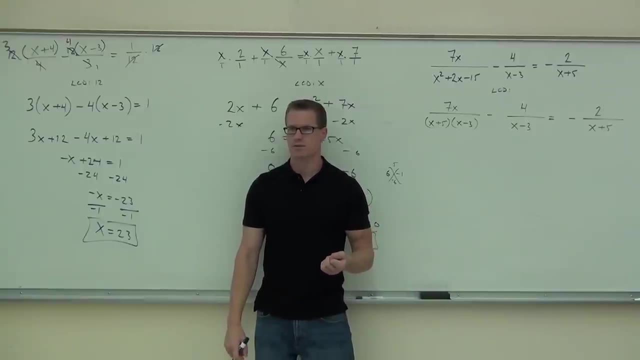 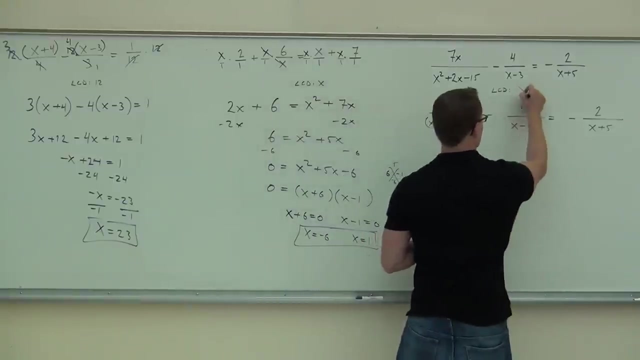 Let's find our LCD. LCD is a listing of every different factor that you have. Can you see the LCD up here? Yes, Yes, What's one factor in here? x minus 3.. Okay, What's another factor in here? 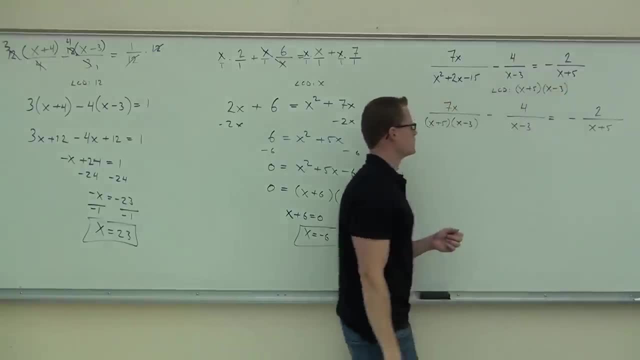 x minus 3.. What's another factor in here? x minus 3.. Is that it Okay? Let's check. X plus 5, we have that. Mm-hmm. X minus 3, we have that, Yeah. 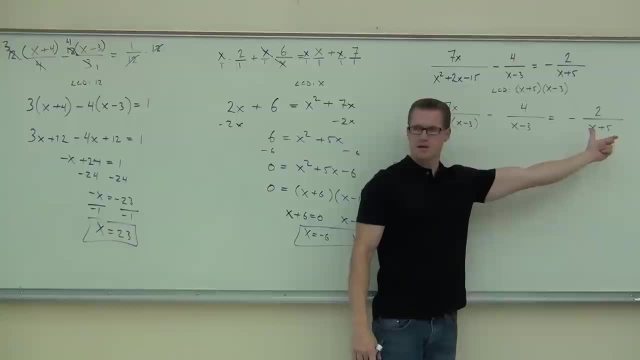 X minus 3? Yes, Already got that. We don't have that. We don't have that. x plus 5? Yeah, We got that. That's fantastic. That's our LCD. Now what do you do with the LCD? 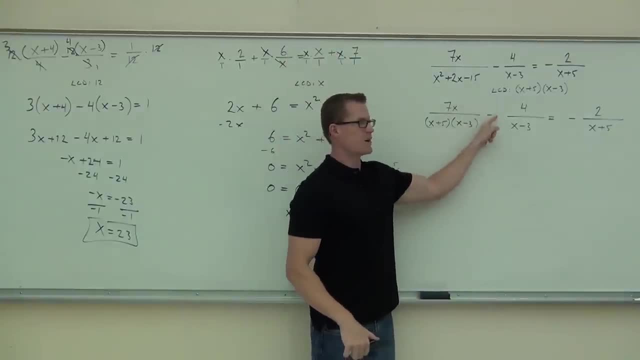 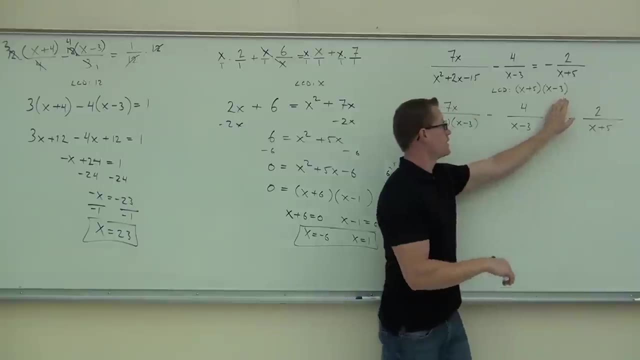 First question: Should I be multiplying x plus 5 over x plus 5 right here? No, Look, If I didn't have this, ignore this side. If I didn't have that side, that's exactly what I'd be doing right here. 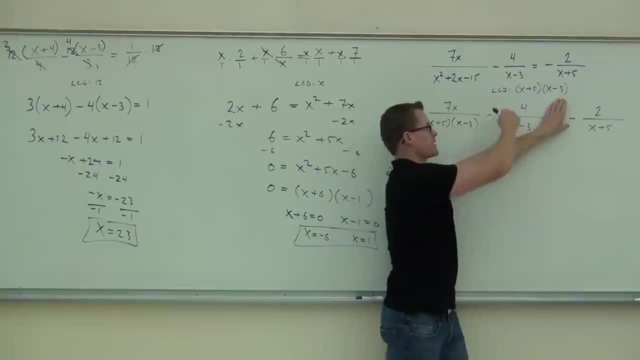 Do you see what I'm talking about? That's exactly what you'd be doing. You'd have x plus 5 over x plus 5.. You'd have a common denominator: You'd combine them. That's what you would do. As soon as I have an equals and sum of the fraction, that changes the plan. 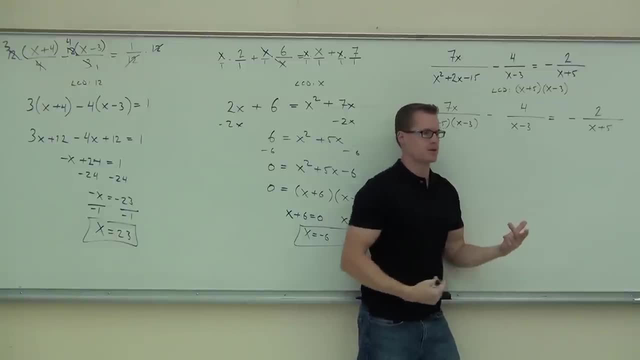 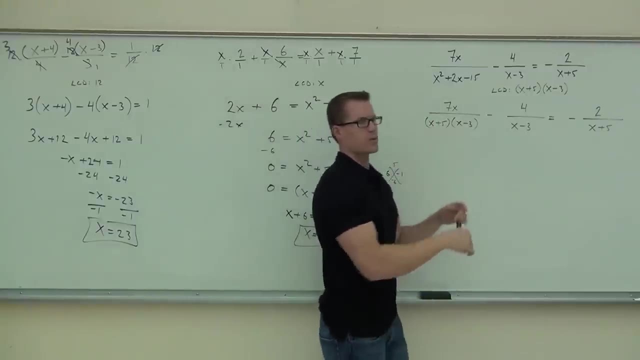 That says oh equals sign. now I can get rid of denominators. That's the goal now. So that's the goal. That means we're going to do this process on that problem. We're going to take the LCD and multiply every term by the LCD. 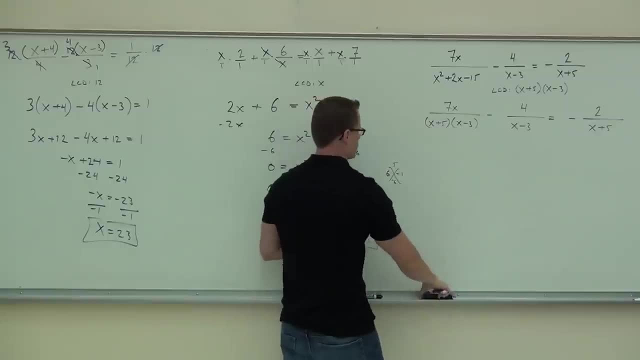 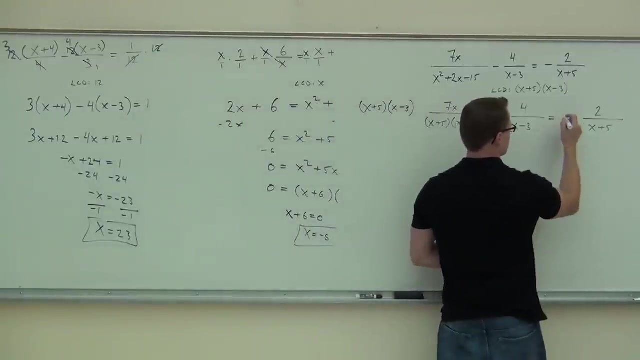 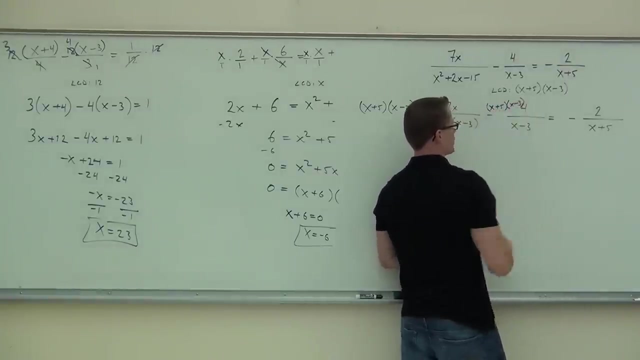 So it might get a little long here. All right, So we're going to take the LCD and multiply every term by the LCD, Because this is going to multiply by the LCD. Okay, that's there. Okay, So I know it's a little squished. 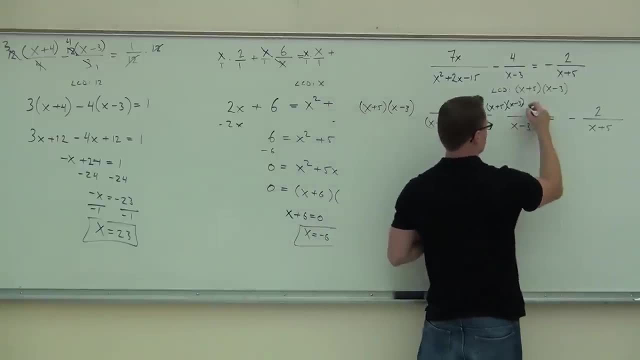 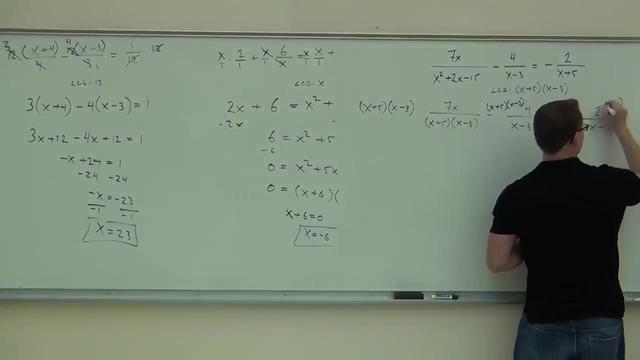 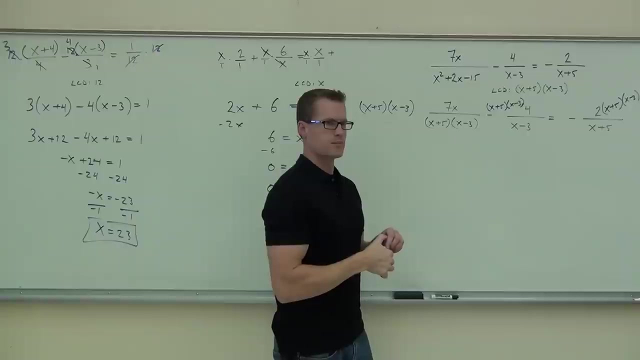 I broke my own rule, But show you All right, Cool, Thank you. See you next time. Okay, Bye, bye. Can you still read that a little bit? still read that in the back. Are you okay in this process? 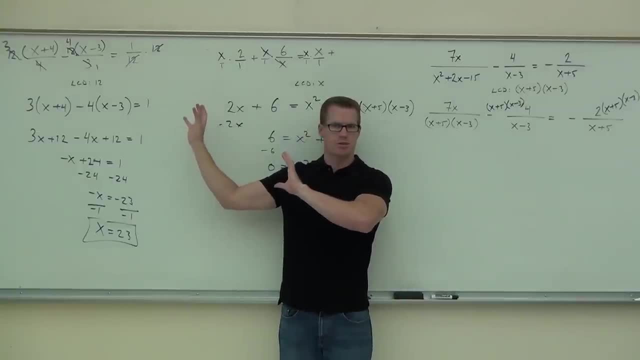 Do you see how? it's exactly the same as what we just did over here? it's just now. we have different factors. Can you see anything that still simplifies? Let's look at the first one. Remember that this is still all over one. if you want it to be like that and you're. 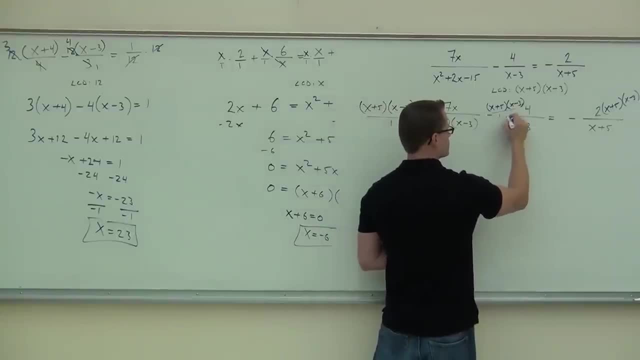 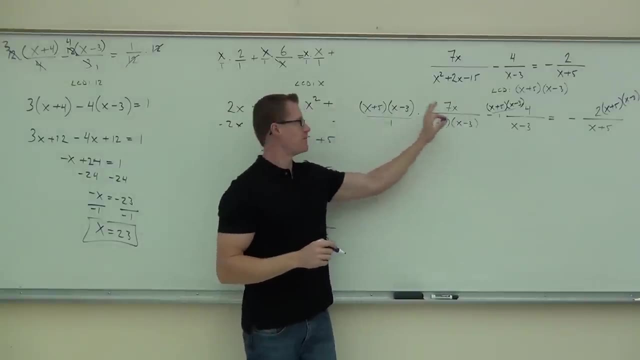 still multiplying. and this is all over one, and you're still multiplying, and so is that one, and you're still multiplying. What simplifies in this first fraction? tell me that, Just like you're simplifying it, like normal, right, you extend the line. we know how to. 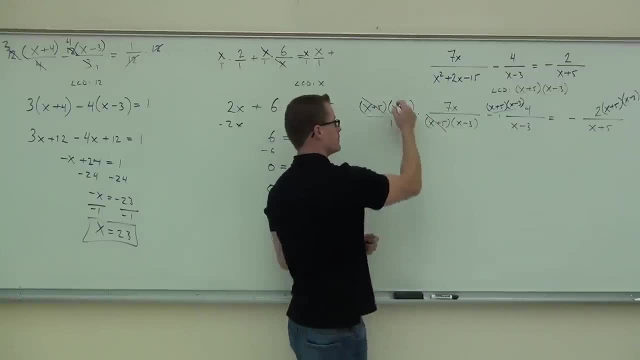 do that. you simplify those out. X minus 3's are also the same. Tell me what we get out of my first fraction: 7x, 7x, 7x, 7x. What's the next thing I'm going to write? 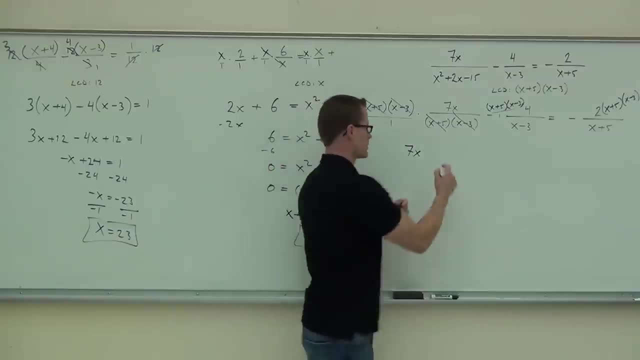 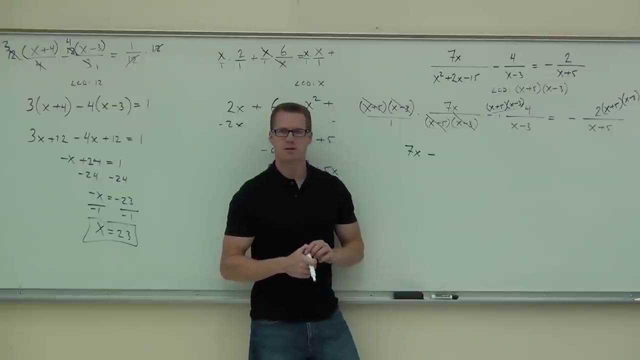 Minus, Good minus. you see the minus, Awesome, we got a minus. Can you look at the second fraction and tell me if there's anything else that simplifies in that fraction? Do you notice how, if you do this process, you will- for sure you have to- if you found? 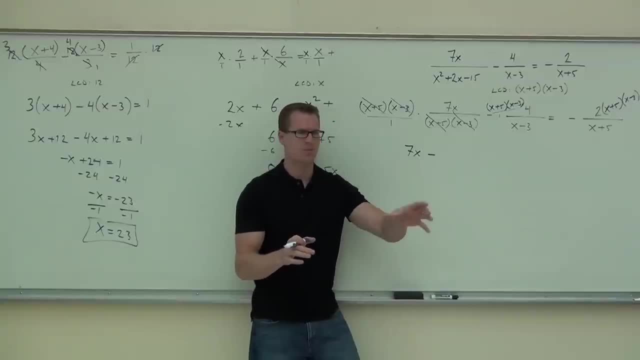 your LCD correctly. you have to get rid of your LCD. I'm sorry, your denominators. do you see that You're using those factors in your LCD? so when you multiply it by it, it's automatically there If you have to cross out, there's no other way around it. 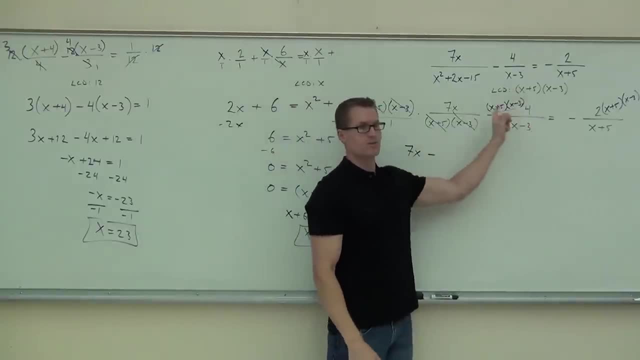 Unless you do something silly like distribute all this. You go, oh, let's distribute that, distribute the 4, and then you can't cross anything out. Then you're kind of stuck right. You have to go back and refactor. 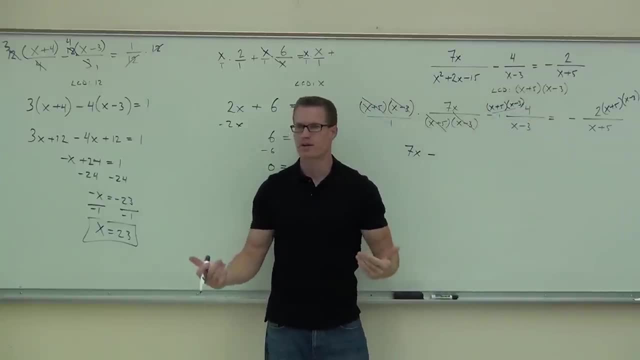 It's very hard to do. You don't want to do that, So here we go. Oh yeah, perfect. X minus 3's are gone. How about x plus 5?? Can I cross out the x plus 5 here, folks? 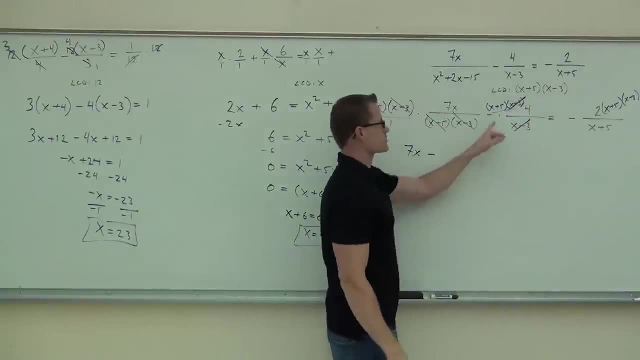 No, Okay, so I already have the minus down. Tell me the next thing I'm going to write: 4.. Oh, don't forget about the 4.. That's there. And then what else? 3., 3.. 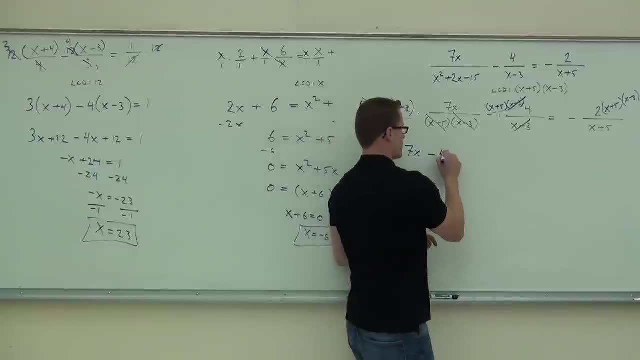 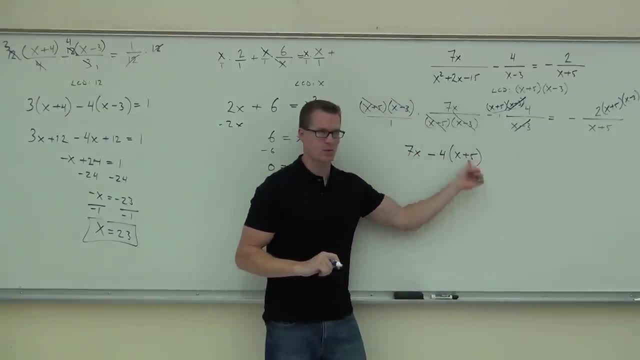 3., 3., 3., 3.. Do you see that when we write it like this, do you see that that negative is going to distribute? Do you see that? Okay, Some of you guys are zoning out here. Zone in. 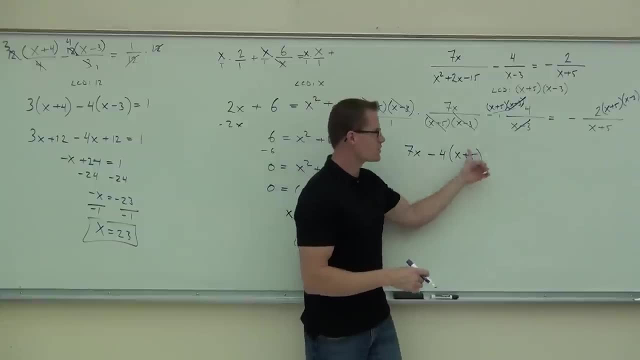 I only need you for 12 more minutes. Let's get going on this. So yeah, that's going to distribute. Then we have an equal sign. What's the next thing I need to write: Minus, Minus. okay, that's good. 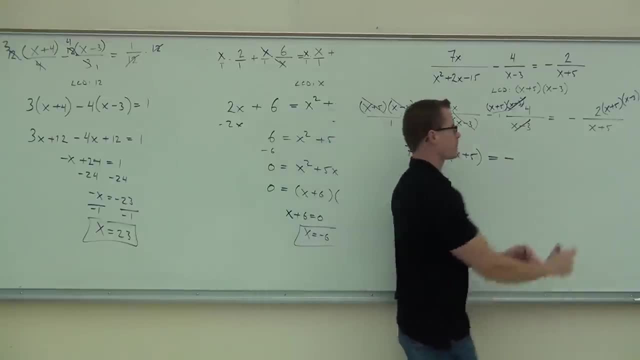 That has to be there. What crosses out on the right-hand side? The x minus 5.. How about the 2?? Yeah, So I still need that and I still need the x minus 3.. Okay, I don't think it's just me. 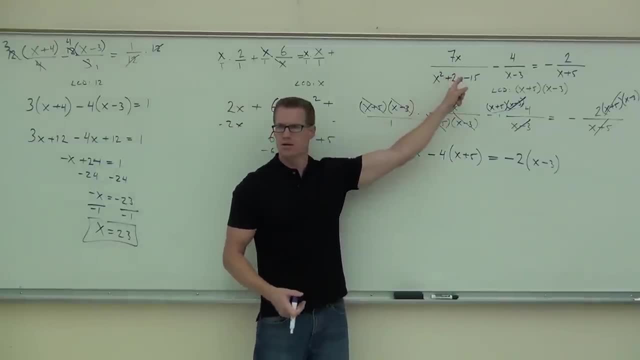 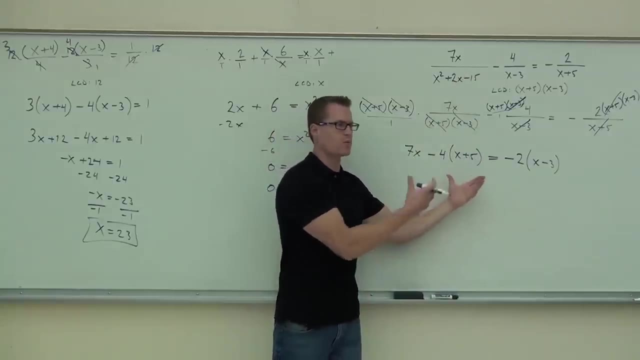 I think this looks a whole lot easier to do than that problem. Don't you think that This looks a whole lot better? This has no fractions. It doesn't even have x squared anymore. We crossed that out. This is awesome. This is what we want to have. 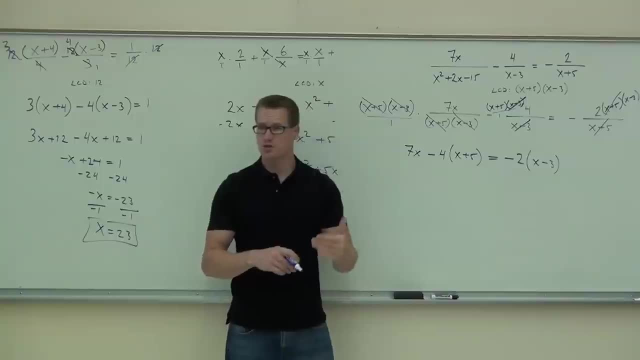 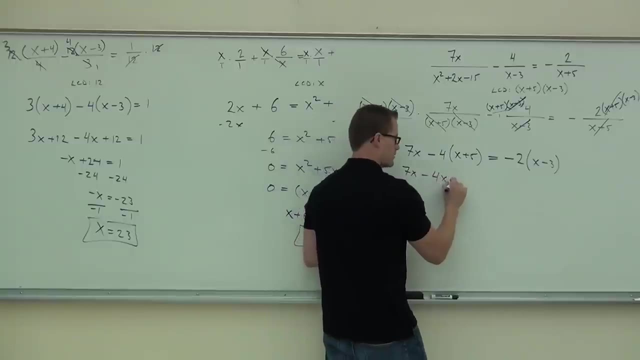 Now all we need to do is what we did on that problem. We're going to distribute, combine like terms that we have and solve. So distributing. we have 7x minus 4x and minus 20.. See where the minus 20 is coming from. 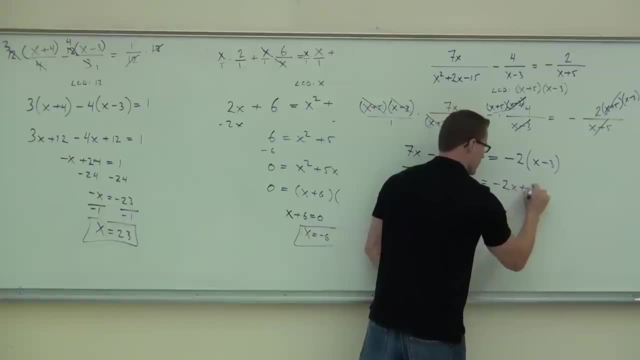 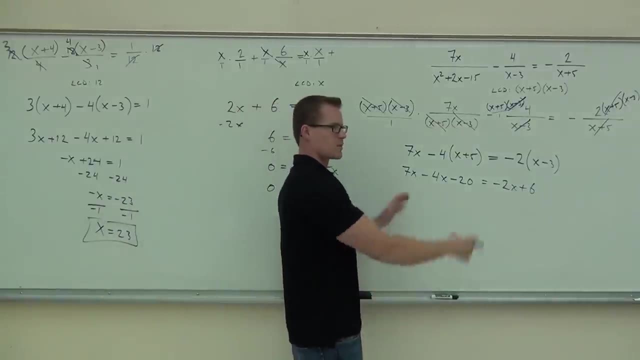 Good On the right-hand side, minus 2x and plus 6.. See where the plus 6 is coming from. That negative is distributed on us When we combine some like terms. remember like terms mean on either side of the equation. 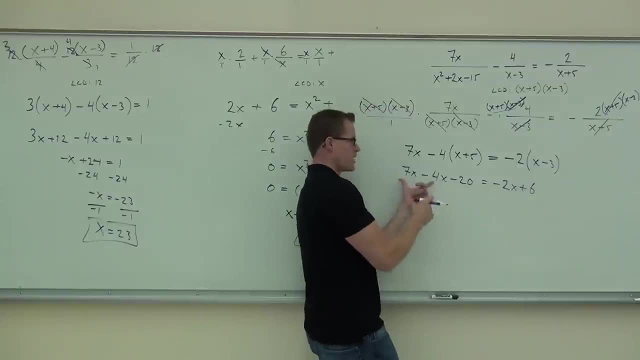 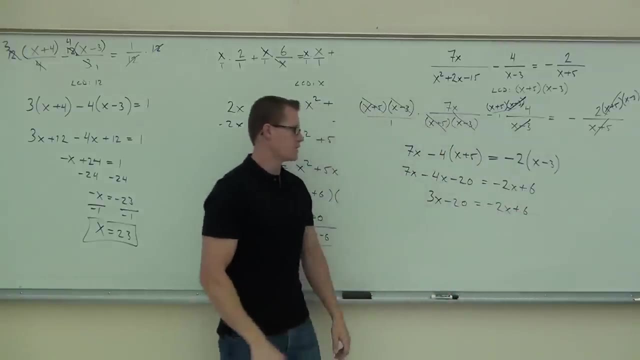 Here you have no like terms. Here you have some like terms. We'll combine our x's. We get 3x minus 20 equals negative 2x plus 6.. Next question I have for you that I want you to answer. 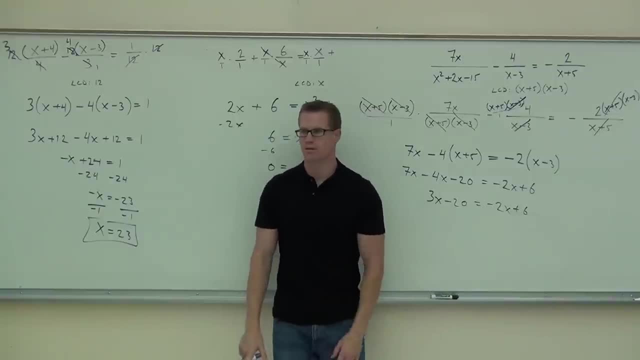 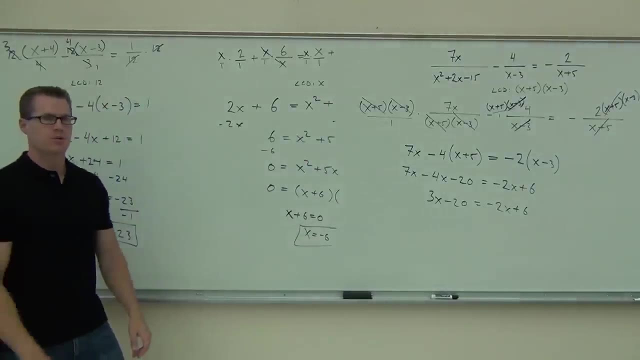 Am I supposed to get everything to one side and zero on the other side On this problem? Is this problem the same as this problem? What's the difference? All right, x squared. that's what we do. That's the only way we know how to solve it right now. 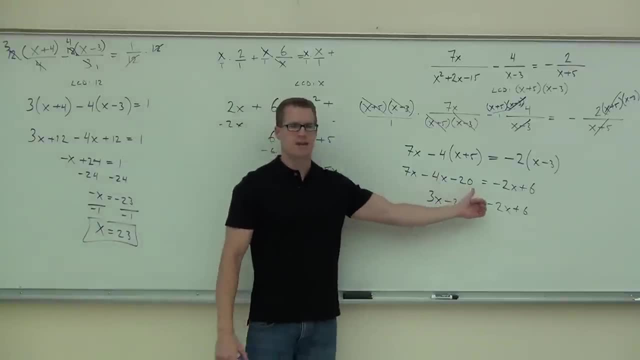 You get it equal to zero and you factor it. Do I need to do that here? The answer is: I don't even have an x squared. This would do me no good over here. This is: get rid of the smaller variable, and then you have something very easy to work with. 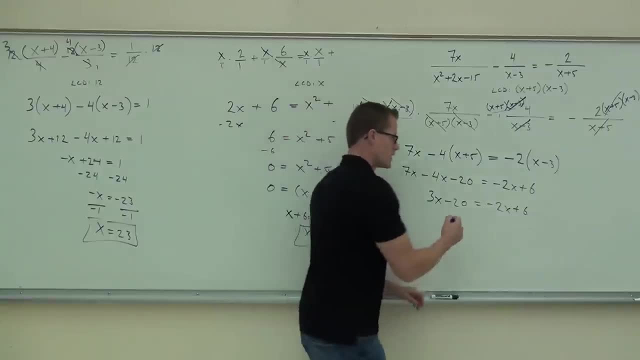 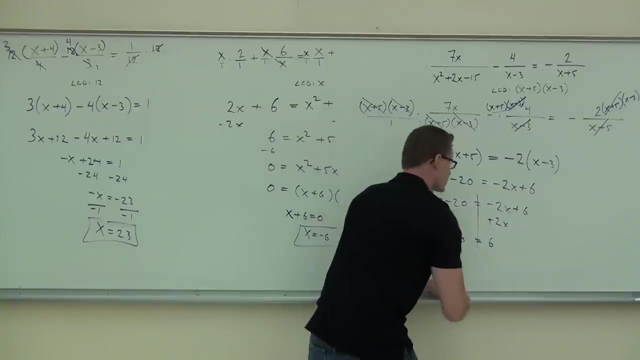 What's our smaller variable up here? Negative 4x. How do you get rid of that? Add 2x, Perfect. We get 5x minus 20 equals 6.. Good, add 20.. Okay, now we're on the whole stretch. 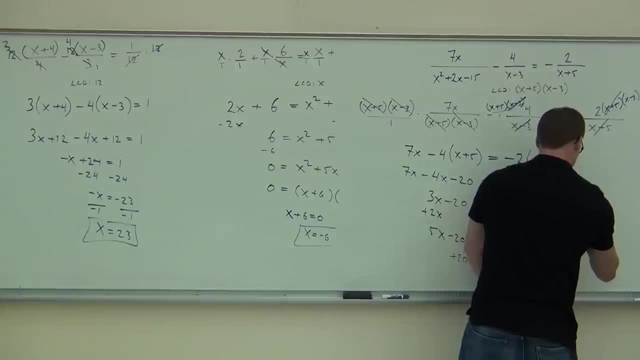 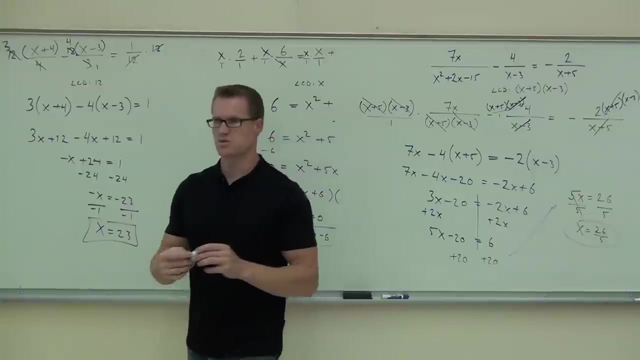 I'm going to move over here. 5x equals 26.. Our last step is always to divide. if there's a coefficient, 1x equals 0.. That's 1x squared Theется. That's it. Good as we can do on that problem. 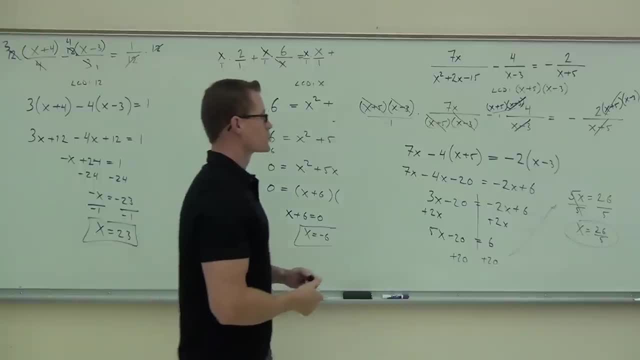 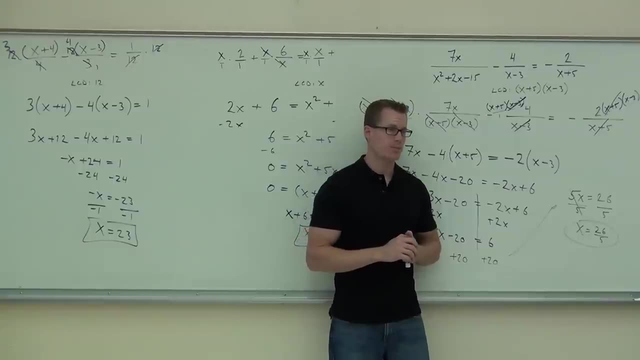 Is it okay to get fractions out of a fraction problem? There's only one thing we need to check. Okay, I need to make sure that you see this Watch up on the board here. There is one thing you need to check: You need to make sure that you can plug this number in and that it's legal to do that. 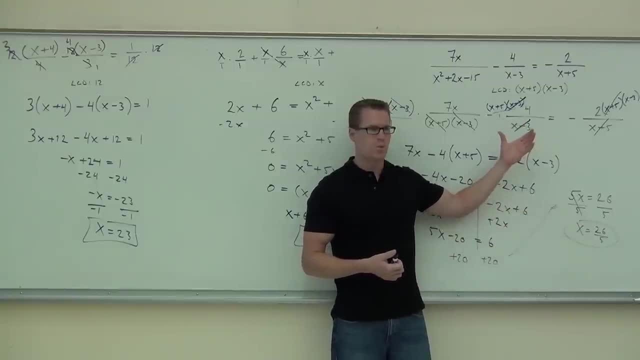 Here's what I mean. Notice, we have fractions here, right? What's the one number you cannot have on the bottom of a fraction? So if you were to plug this in and it made zero here or zero here or zero here, you'd. 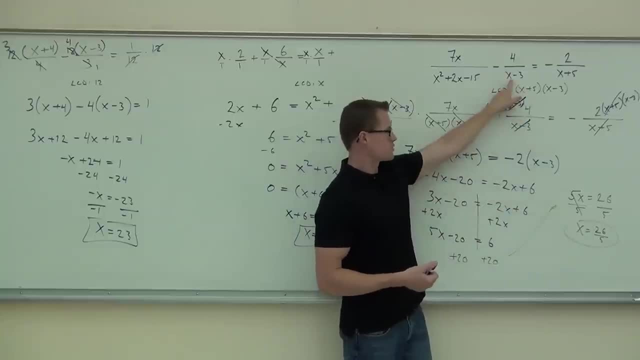 have a problem, right? So you plug that in. Is 26 fifths minus 3 going to give you a zero? No, The only thing that would give you a zero would be a 3 here. right? The only thing that would give you a zero here would be a negative 5.. 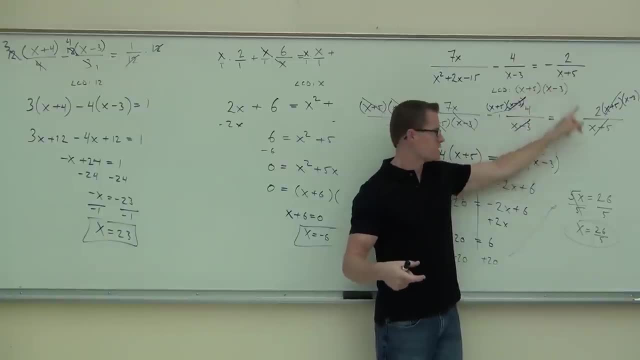 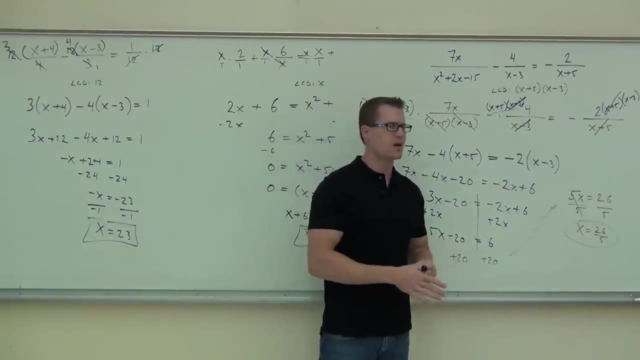 Remember we talked about the domain stuff. So you check that, Just make sure that this number is not going to give you zero and you're okay. That's the solution. If it gives you zero, then you cross it out. It's not a solution. 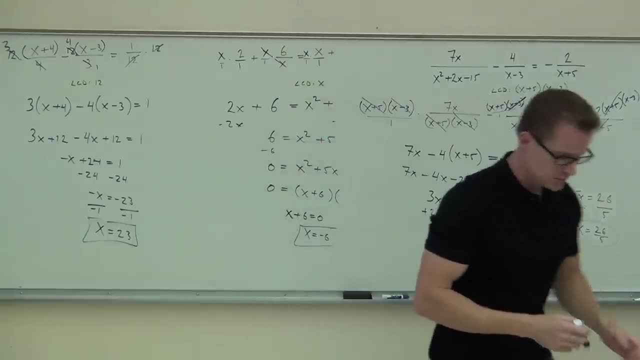 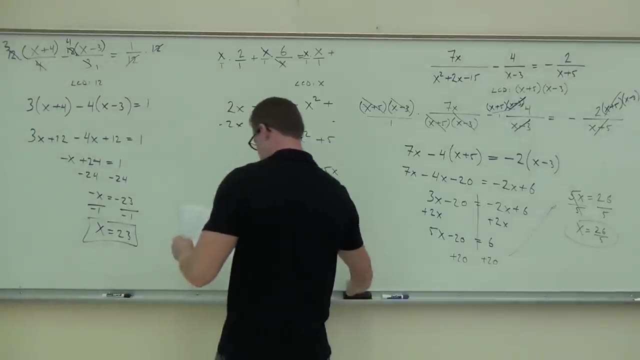 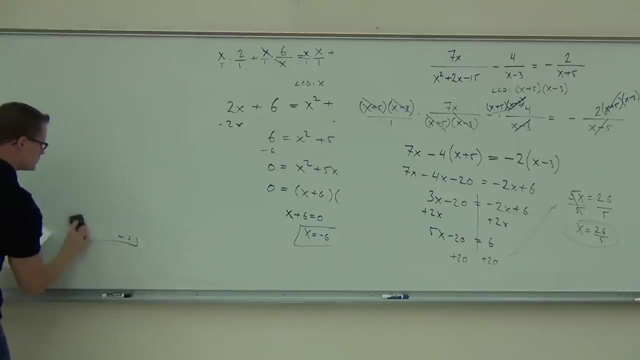 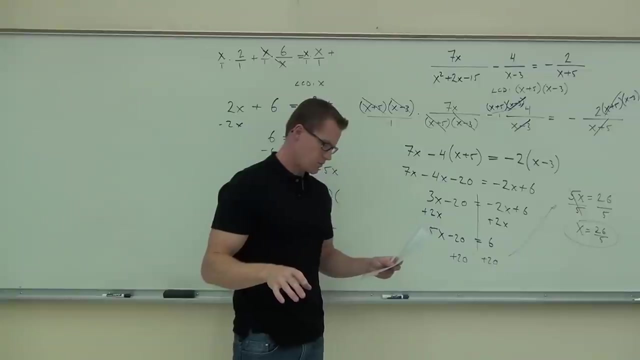 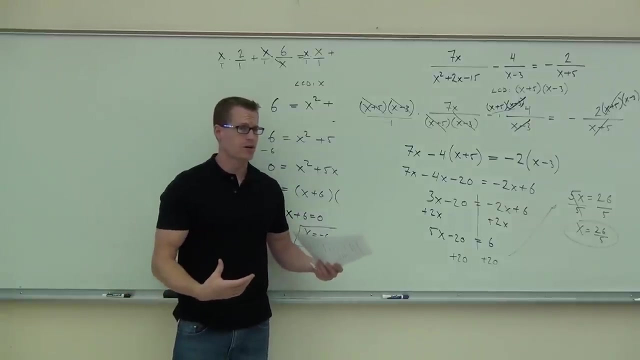 We will understood that problem. Good, All right. Okay, Like I said, we're going to do one more together. I will give you two to three to do on your own, and then we're done. Honestly, we already had this section kind of covered from the first day of class. 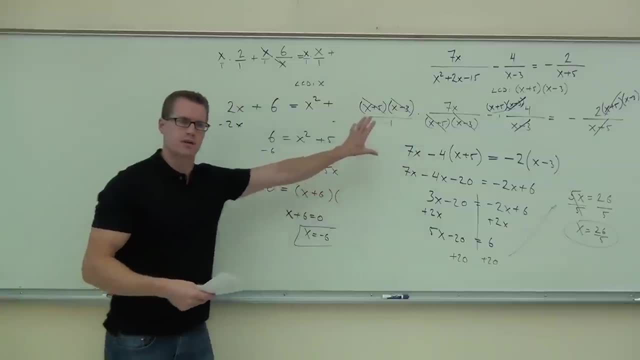 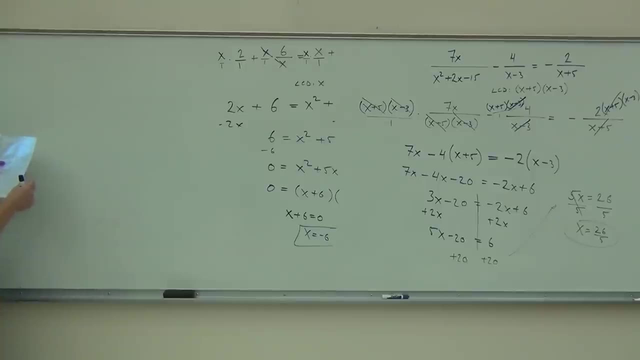 It's the same stuff. It's. just now you're working with expressions like those. So, same idea, So we're going to do that and then give you some practice. Okay, All right, All right. Okay, All right, All right. 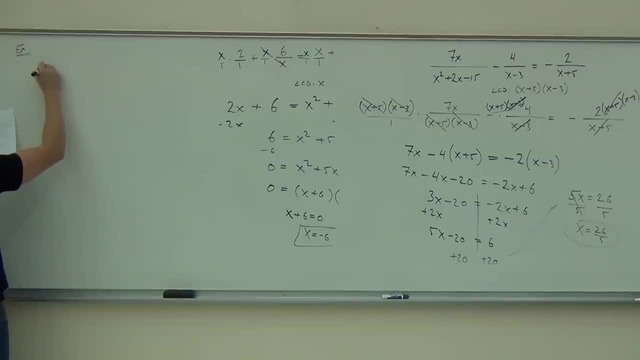 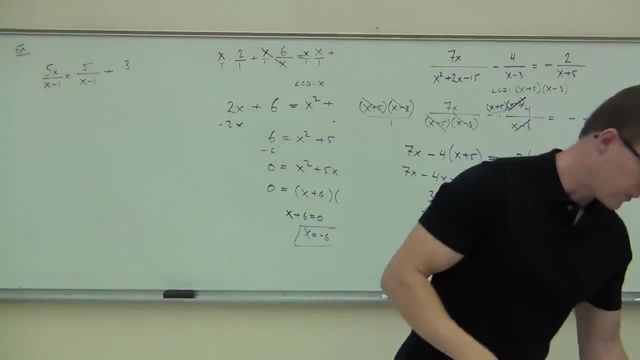 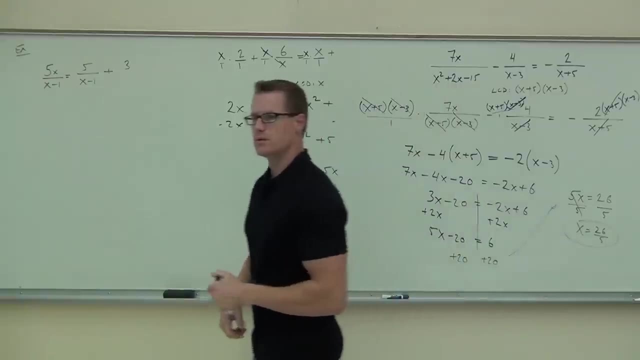 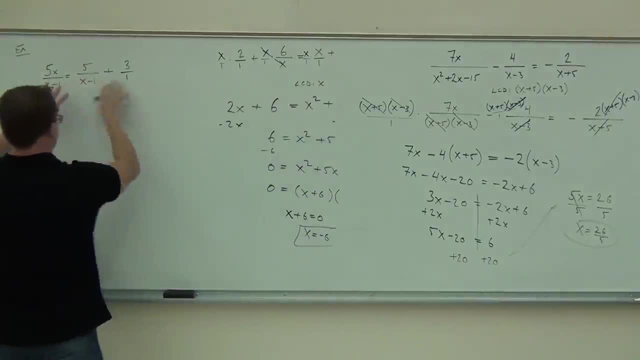 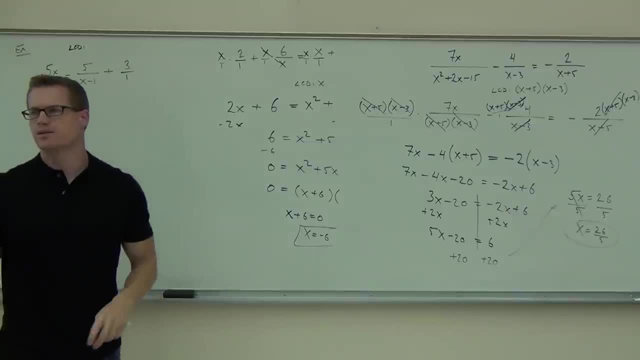 this is three, is not part of our LCD. What is our LCD here? Well, that's not bad. I like that. Okay, We have LCD. what's the next that I'm going to do right now? OK Times, how many things. 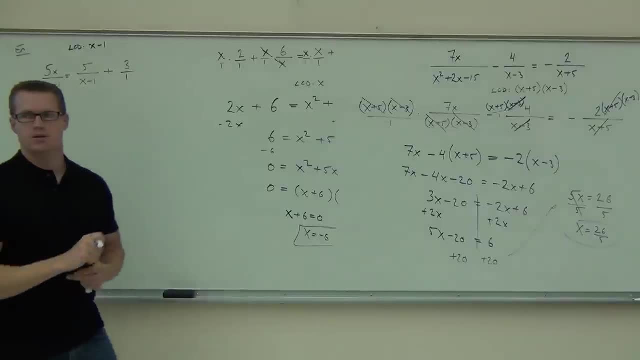 So that's here. I'll put it in parenthesis, I'll make sure it's in parenthesis here as well, which is 20, and then 3,, and then 3, and then need to write after n, So plus x, And then it's also here. 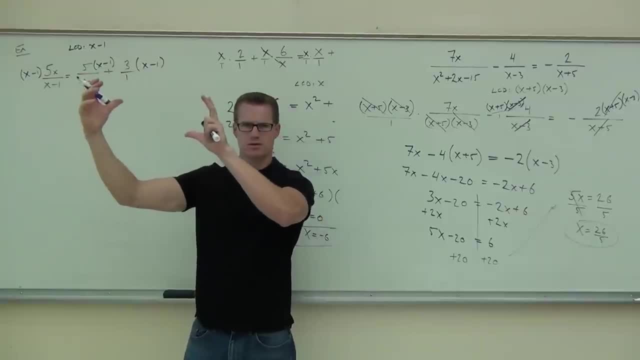 Should it be x minus 1 over x minus 1, or just x minus 1?? Just x minus 1. Over 1.. OK, we can do that also. Why am I able to do this? Why can I get rid of denominators? 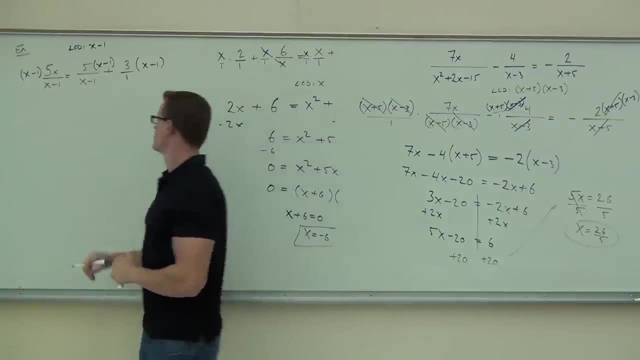 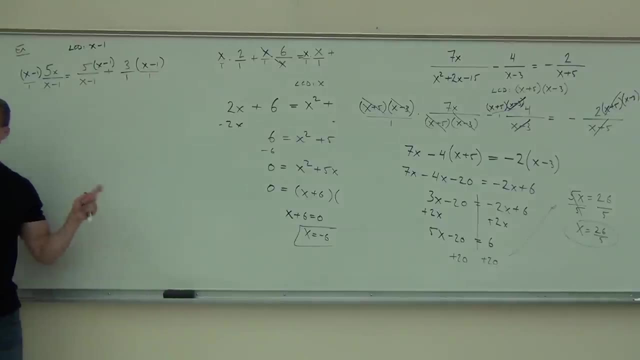 What tells me I can in this problem Equals 3.. OK, so maybe I put this over 1, if you want to show that. That's fine. Let's cross some stuff out. This is the best part of this process. Let's cross some stuff out. 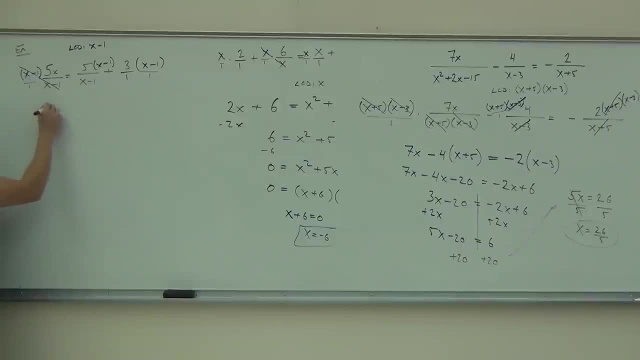 Here I see the x minus 1's are gone. What am I left with? I have an equal sign. Then I have an equal sign. I see the x minus 1's are gone. I get what? 5.. And then over here I have plus 3 times x minus 1.. 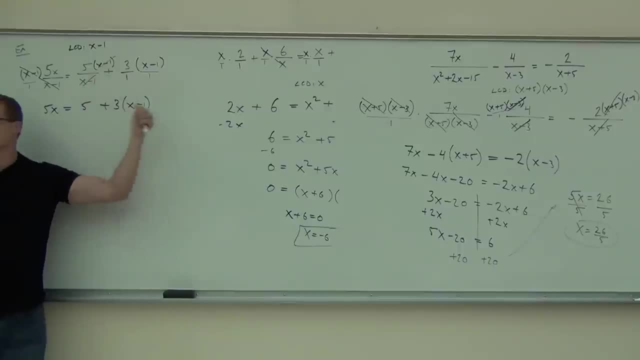 I'm not going to distribute, Just in case that was a minus sign, because I want to see that. So I wait for distribution. just one step, Not a big deal. 5x plus 5 equals 5.. And then we're going to get the 3x minus 3.. 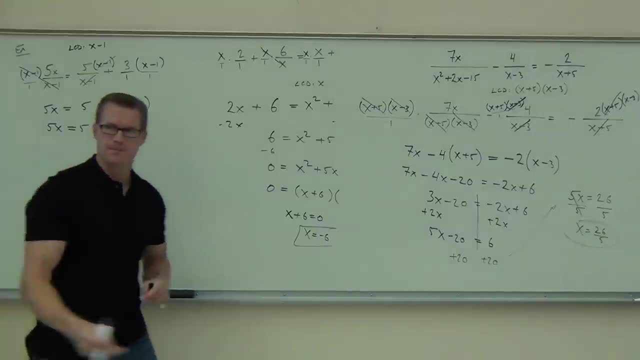 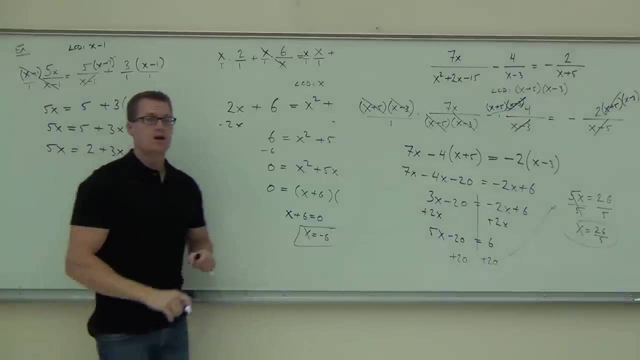 Still OK so far. Next step: what do we do? Quick, So we have 5x equals 2 plus 3x. That's combined like terms. Next step is: well, either A or B Choice. A is you get everything. 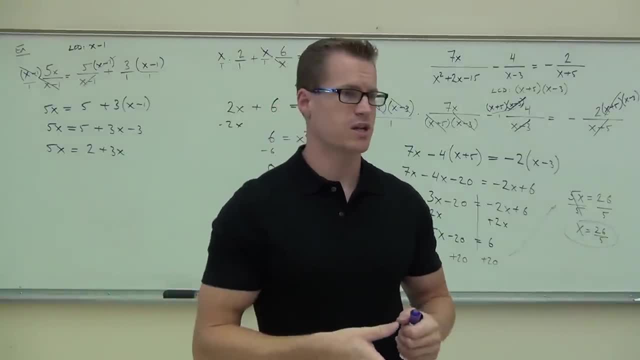 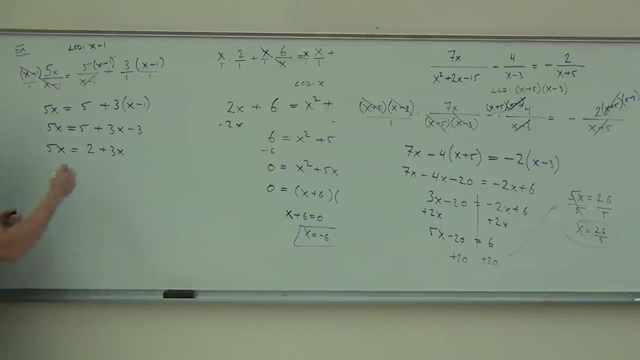 to one side and 0 on the other side. Choice B is you solve this just like it is, because you don't have an x squared? Choice B. So we're going to do what? Minus 3x, Perfect. We get 2x equals 2.. 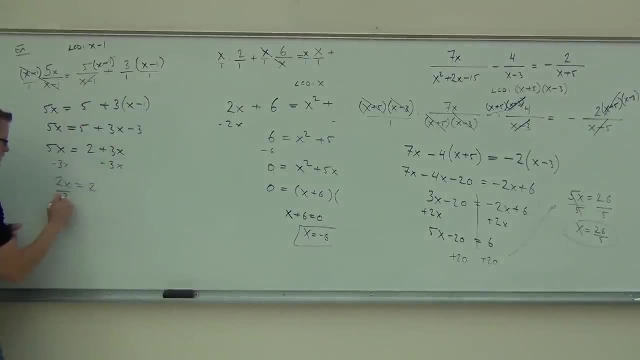 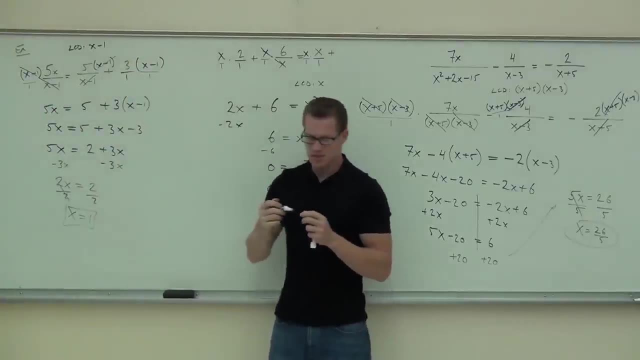 Very good. And the last step is Minus 3x And we get x equals 1.. I would feel good about that solution. I would too. I would too, Except I want you to look back. We just talked about this. 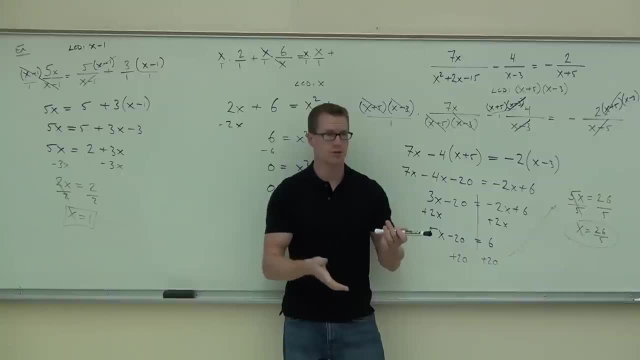 Is that a solution? No, It looks like it right. We solved it. We got an answer. Look back at the original problem. Take that: 1. Plug it in. Look at the denominator 6.. Is that OK? 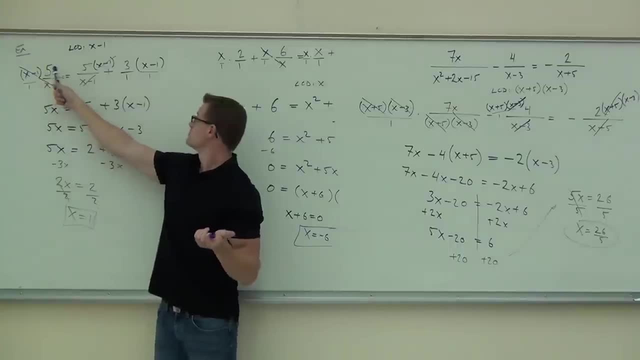 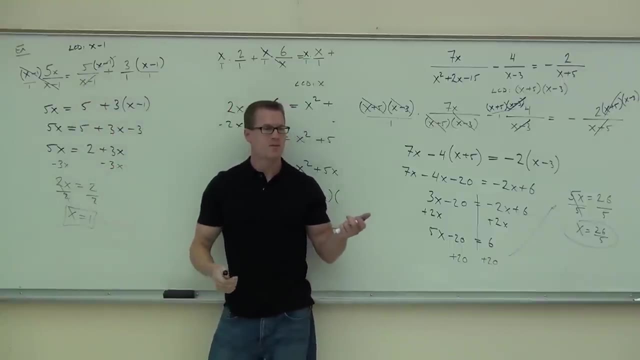 No, Here, Hey, that looks good, It's 5.. Here, that looks fine. That's fine, It's fine Here, it's fine Here. oh crap, What happened? We plugged in 1. We got a 0, right on the bottom of our fraction. 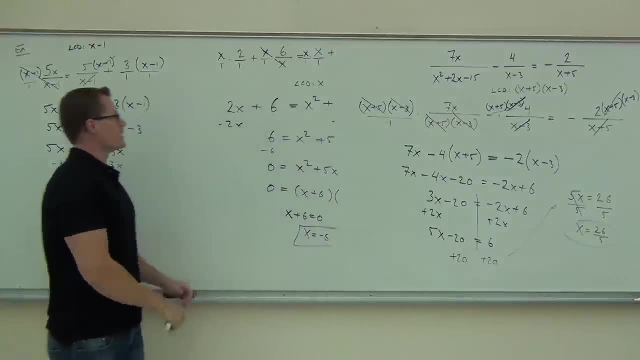 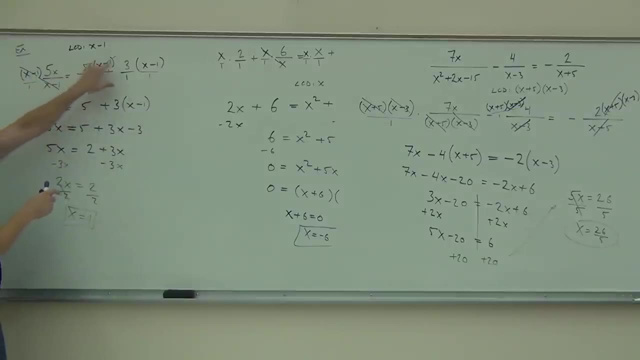 Why does that happen? The answer is: when you take this and you multiply by the LCB, you're essentially moving this to the top of your fraction. Do you see what I'm talking about? Essentially, that's what you're doing. 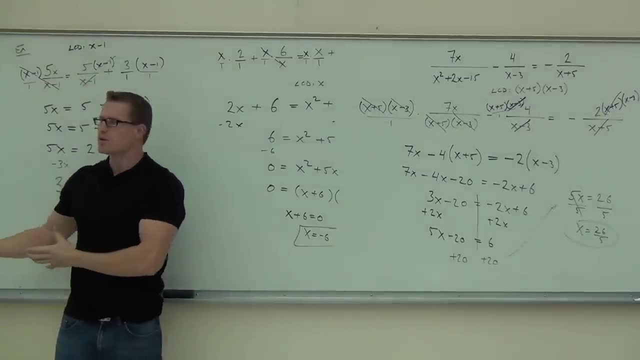 In doing that, you can create something. You can create some false solutions. This is a false solution. So what you do, you get all the way down to here. That one worked just fine. That was fine. It didn't make 0.. 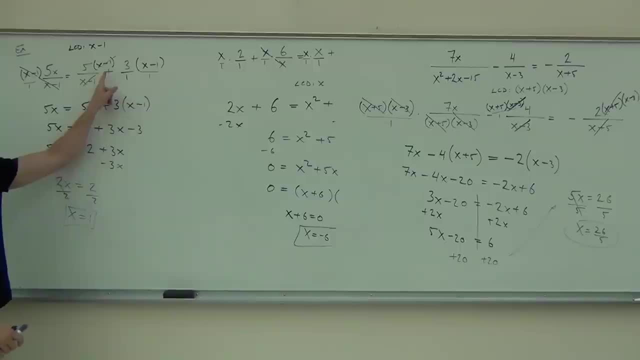 This one. this is a problem Because when I plug this into the denominator, it gives me 0. That's undefined. If you get something that's undefined, all you're going to do is solve it down. You're not going to know until the very end. 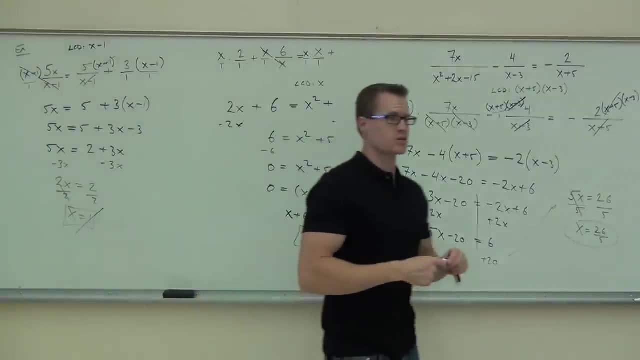 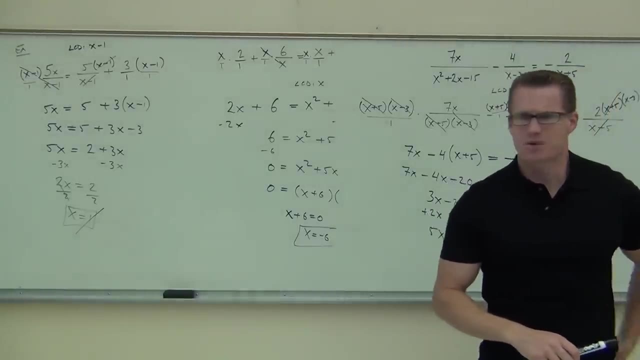 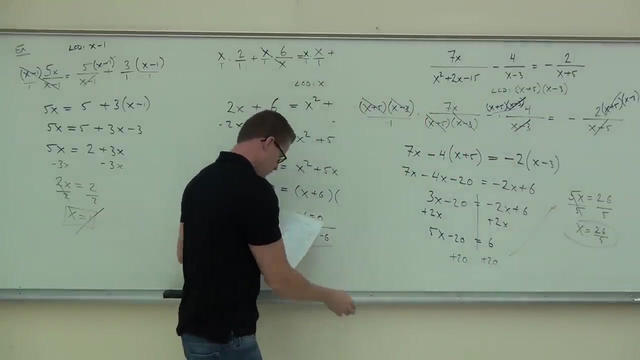 Just cross it out. That's not a solution. There is no solution to this problem. I know you're not used to problems not having solutions, but this is one of them. OK, I'm going to give you two problems to do on your own. 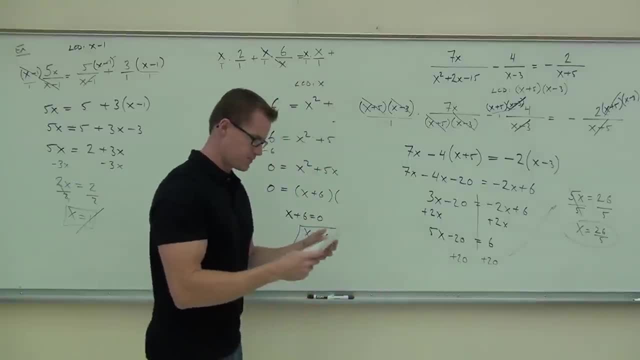 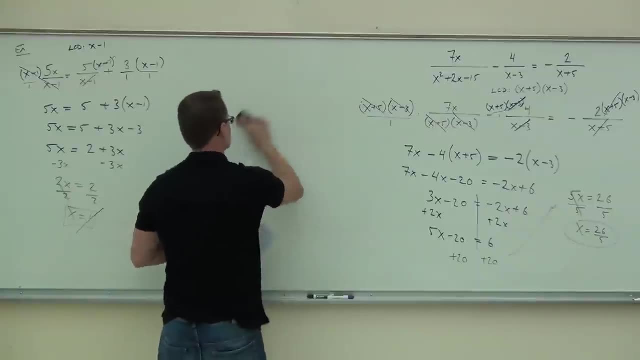 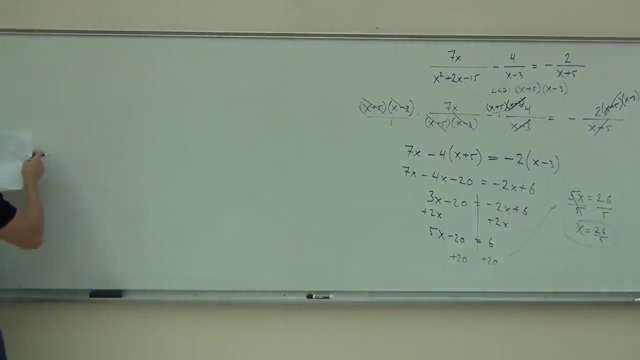 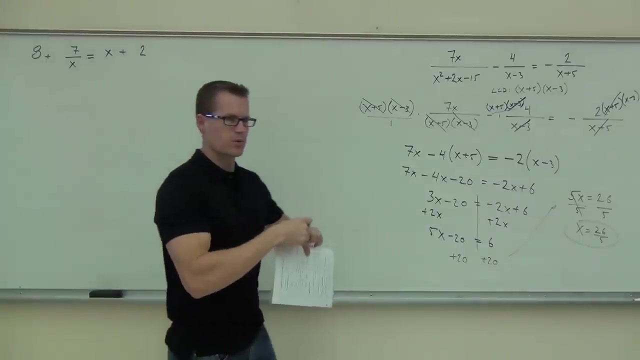 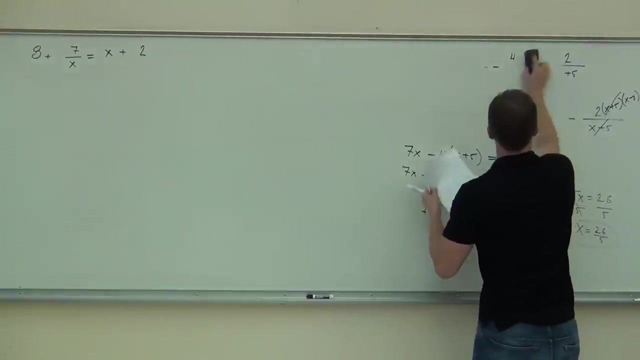 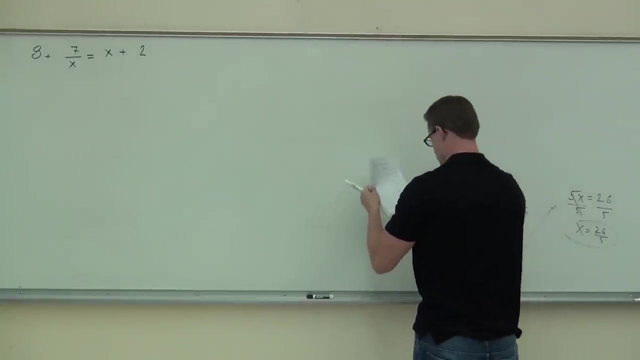 one similar to this one, one similar to the one we did over here. OK, so there you go. Work on that one. I think I'm going to write two on the board. I think we can go pretty quickly through these. I'm going to do it one at a time. 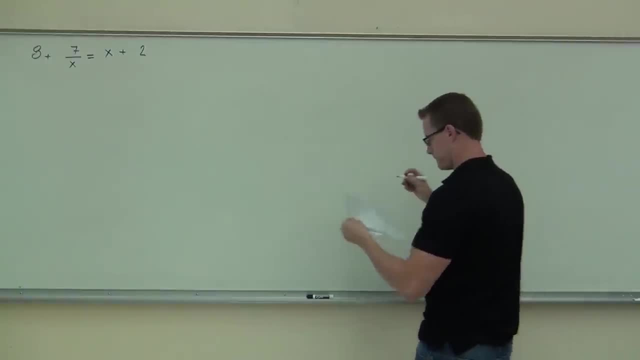 I think I'm going to do it one at a time. You can go pretty quickly through these. I don't know about you, but if you have problems you can go ahead and write them down. I don't want to go all out. 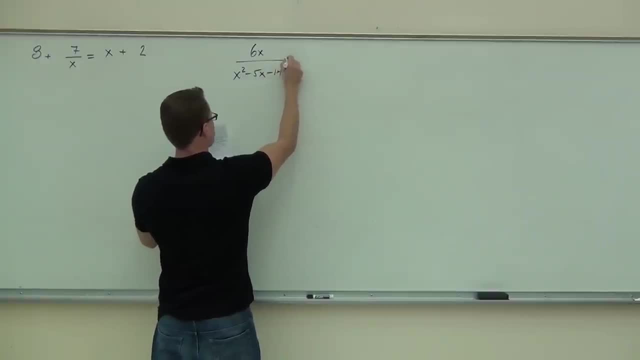 All right, But let's see if you can do it. OK, I'm going to go ahead and talk to this one. All right, All right, Got it All right. OK, next, OK, next, OK, OK. 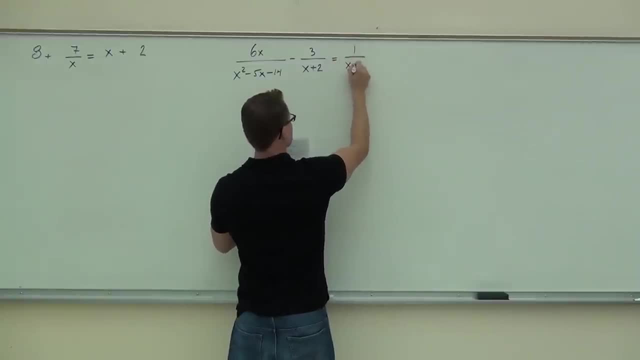 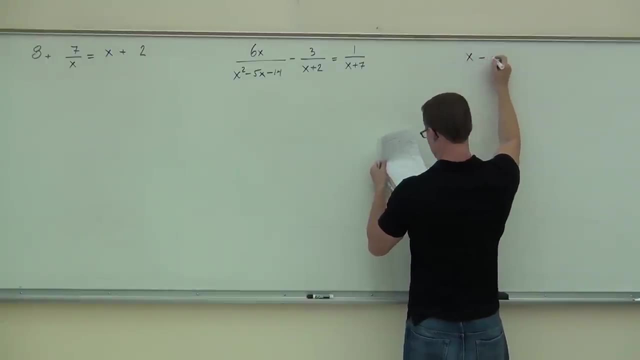 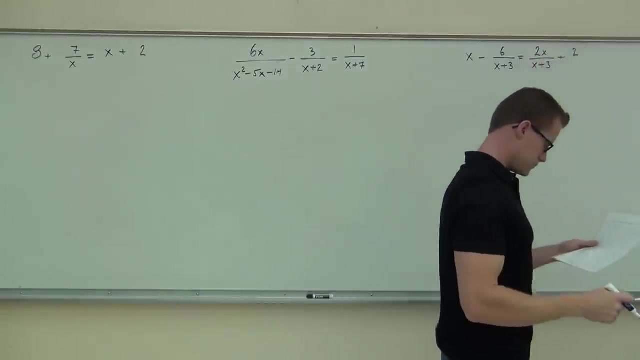 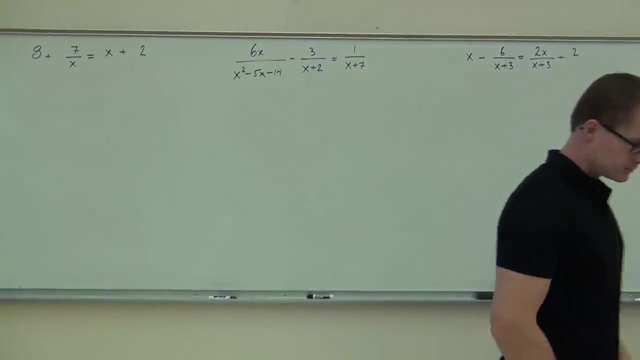 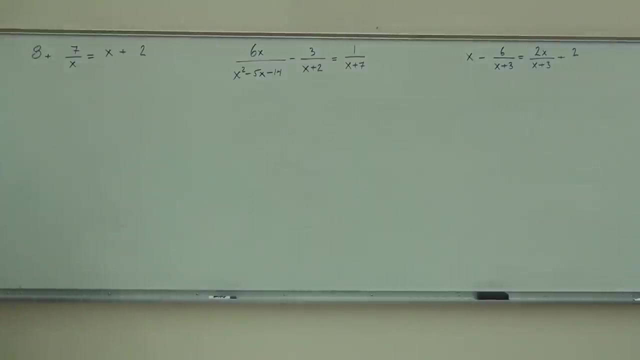 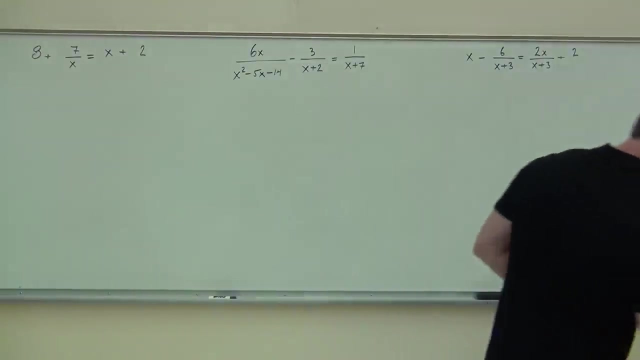 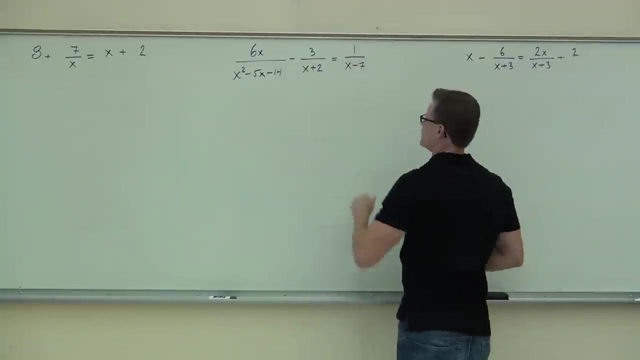 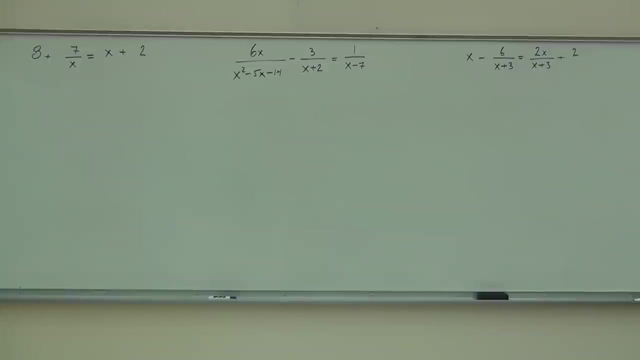 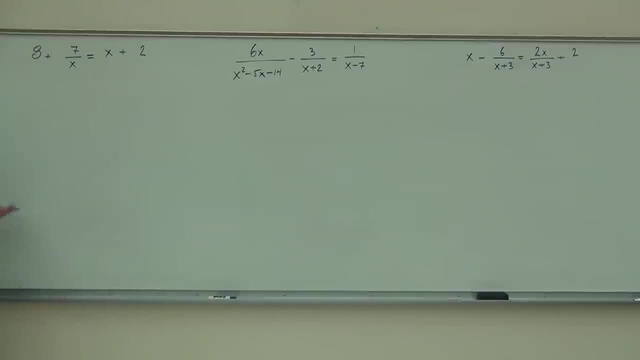 and we're not going to have time on that. So, on the first problem, of course we're going to make this all over one. I hope that you did that. I hope you found your LCD- Your LCD is what here? Good. 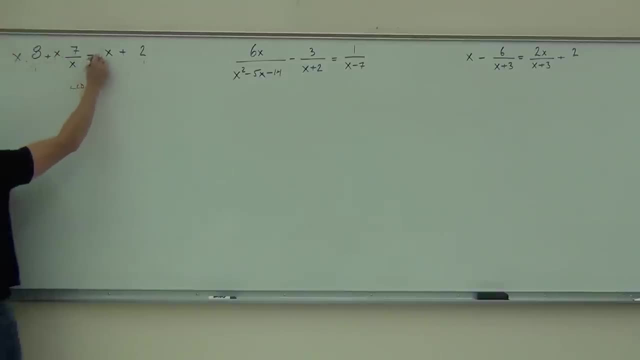 We're going to take and multiply everything by X, Really X over 1.. Let me show you, Let me show that if you want Here, we'll get 8X, We'll get. oh, those are gone, We'll get plus 7.. 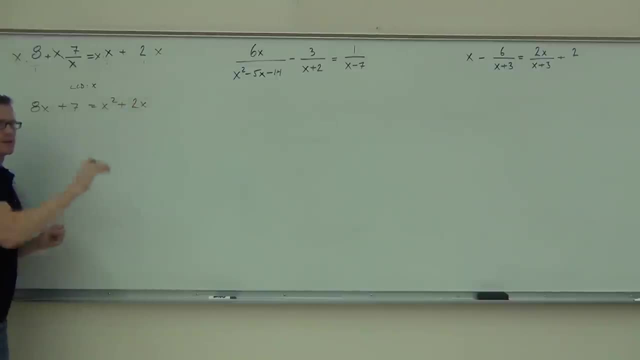 We'll get X squared and we'll get plus 2X. How many people made it that far on that problem? Very good, Now do we solve this like it is, or do we have to get everything to one side and zero on the other side? 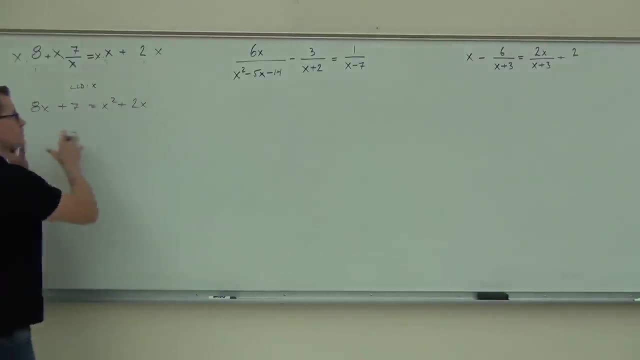 Got to get zero, Otherwise the factor's not going to make a difference. So zero, we're going to move the left to the right or the right to the left To the left, Okay, So minus 8X, 7 equals X squared minus 6X. 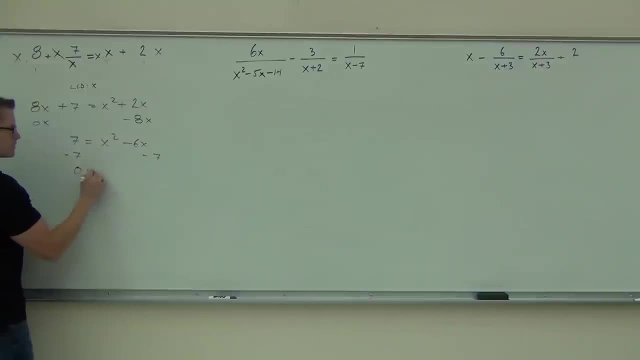 We'll subtract 7.. Zero equals X squared minus 6X minus 7.. You still with me on this, folks, We'll do what now? I'm thinking minus 7 plus 1. You're not quite done yet. You do have to set them each equal to zero. 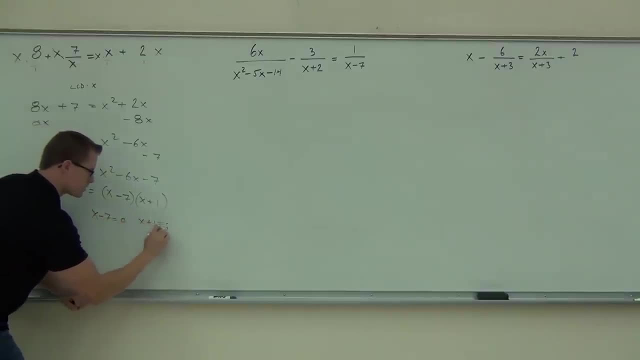 X minus 7 equals zero. X plus 1 equals zero. We'll add 7,, which is 7.. We'll subtract 1.. X is negative 1.. You have to check one thing: Make sure these denominators don't make this zero. 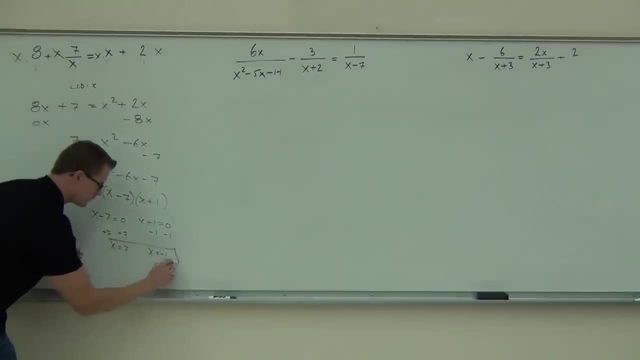 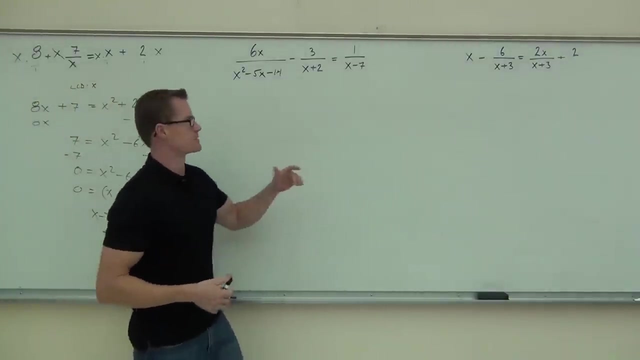 They don't, because they're a positive and negative number, They're integers, So we're good. They're both solutions in this case. Now the next ones. we don't have time to go over. I only have like 10 seconds. 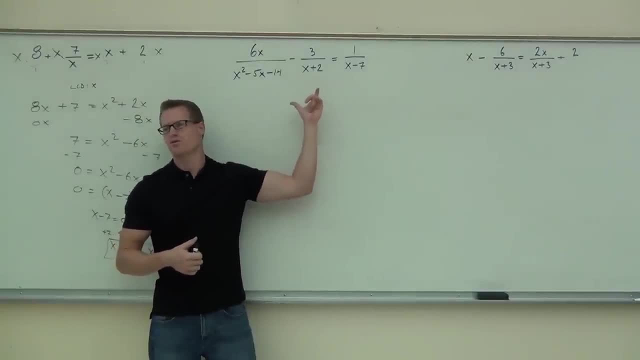 Do you know how to do this one? What would you do? first, Diving, Diving Great Factor. find your LCD, multiply three things by that, Simplify, distribute and solve it. You don't even get an X squared on this problem. 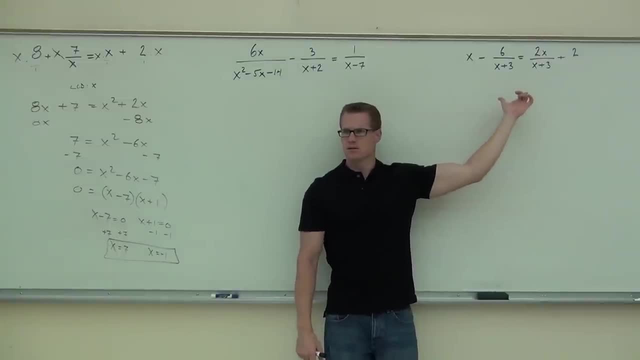 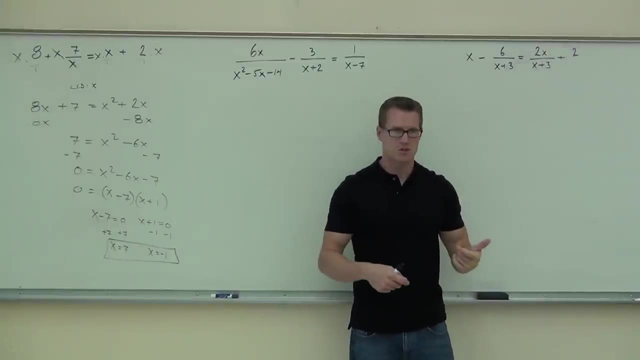 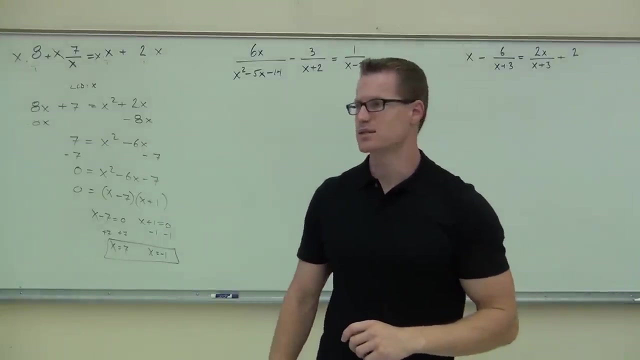 This one. can you see your LCD already? Just multiply everything by X plus 3. Distribute: You will have an X squared. Get everything to one side and solve it. These are our last two problems. We'll do them the first. maybe five minutes of class next time. 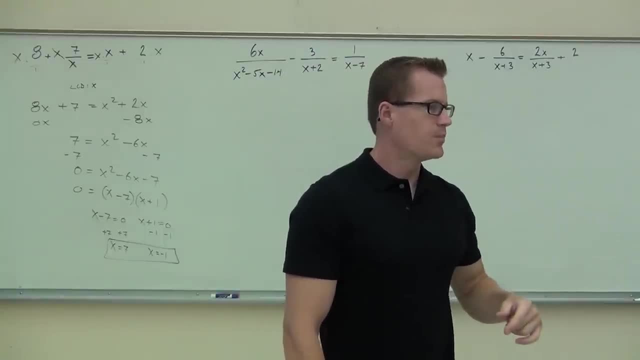 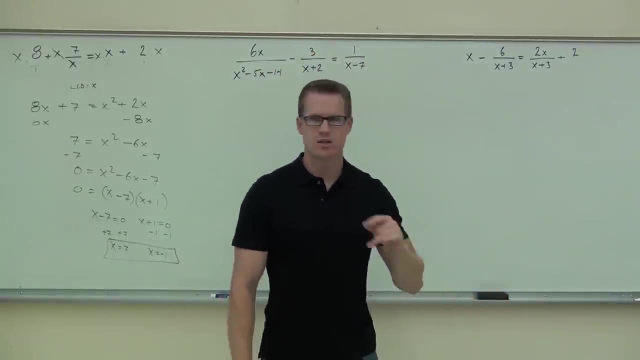 And then I'll post that with this lesson. But we're essentially done, That's it. That's all we've got to cover. So I'm going to give you your homework. It's not going to be due tomorrow, but I really do need you to start on it. 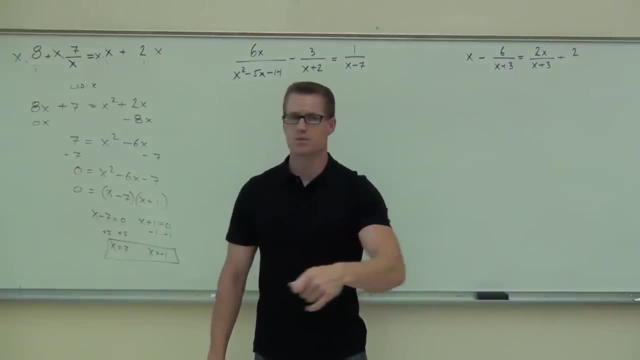 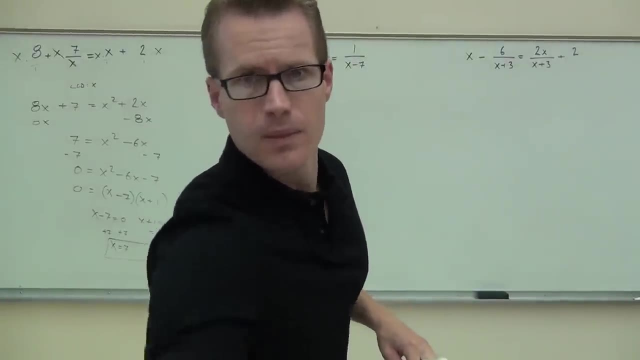 because you're probably going to have another homework assignment tomorrow. okay, So you need to get almost done with this assignment. So here you go. So if you remember from last time we were about to do these problems, Can you tell me what's the first step in doing the problem? 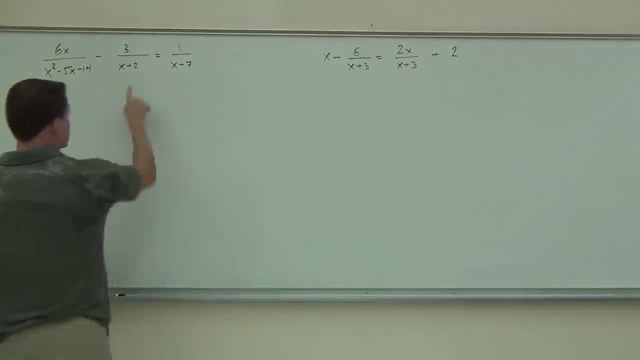 on the left-hand side, which we need to know Factor. So let's factor that. These two, of course, are factored. Okay, But this one we're going to do it, And this one we'll take and factor it 6x and we'll get x plus 2, x minus 7.. 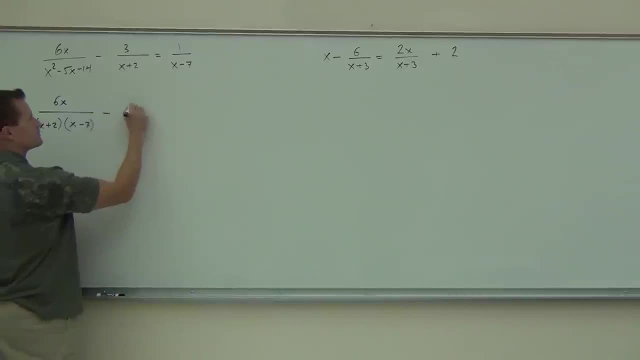 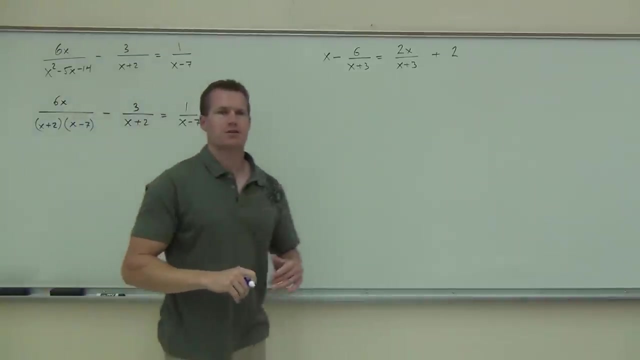 So we should know how to factor the diamond method. no big deal. After you've factored, what's the next thing we should try to do, folks? Okay, Can you see the LCD up there right now? What is the LCD for us? 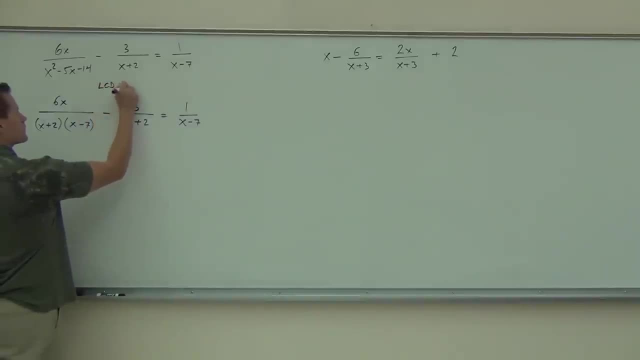 So we have the LCD now. what do we do with that? Are we trying to find a common denominator or are we trying to eliminate denominators? What do you think Eliminate? Great, How do we do that? Multiply the denominator. 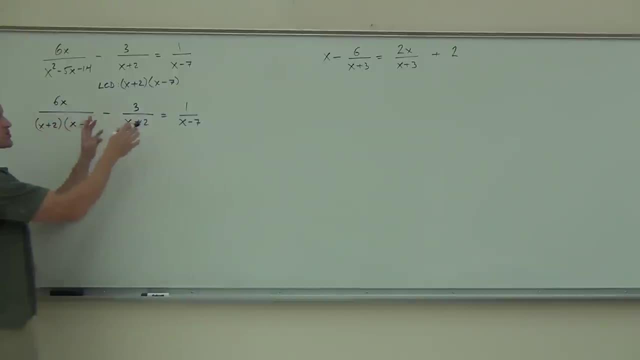 Okay, So everywhere we see a term or a fraction, we're going to multiply the entire LCD. What that's going to do is simplify out all of our denominators. Remember, if you make it to the next step and you still have a fraction. 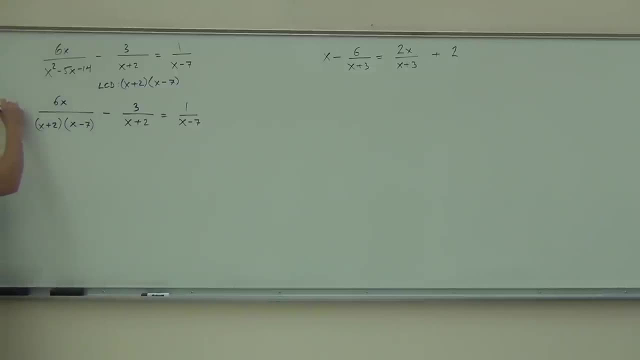 you've done something wrong, go back and fix that. So everywhere we're going to have, in our case, x plus 2, x minus 7,, even over here. Notice that. the reason why we can do this is again: what do we have up here? 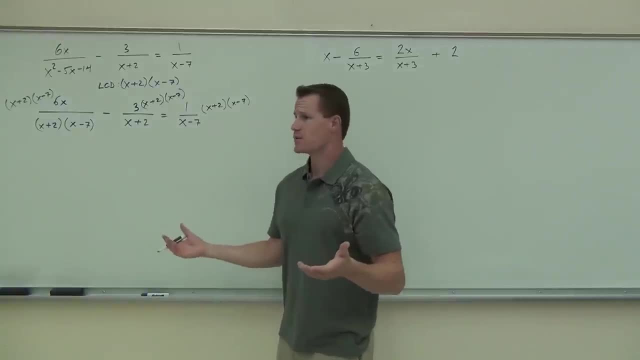 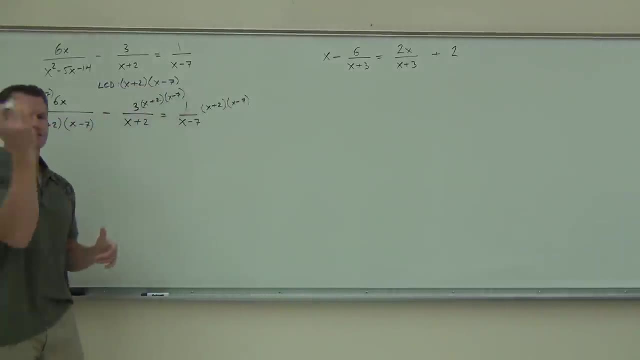 that we didn't have on the last section's homework- Equal sign. That's why That's what tells you you can do it. If you have an equal sign, that means you can multiply both sides by the same thing, Or, in other words, every single term. we can simplify out our denominators. 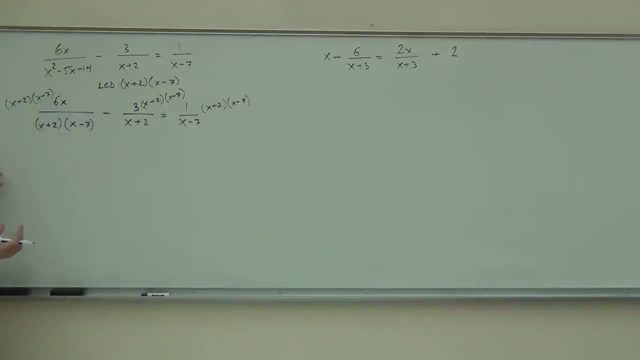 and that lets us do this problem very easily. So what simplifies up here? How about in our first fraction? What are we going to have left? 6x, That's great. So all of this stuff is gone, We have 6x. 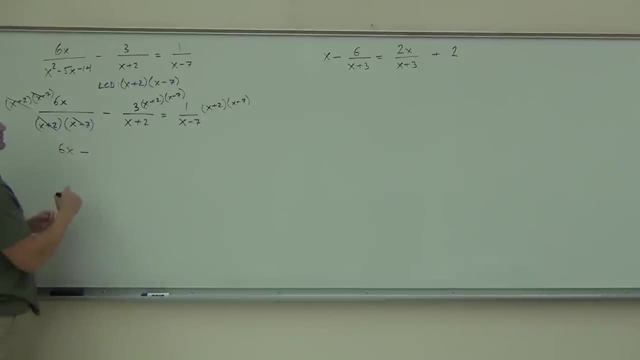 Then we have a minus sign. And what simplifies over here Now. are we going to distribute now or wait until the next step? What do you think? Definitely wait. Yeah, we're going to definitely wait because we want to make sure this minus sign gets distributed with that 3.. 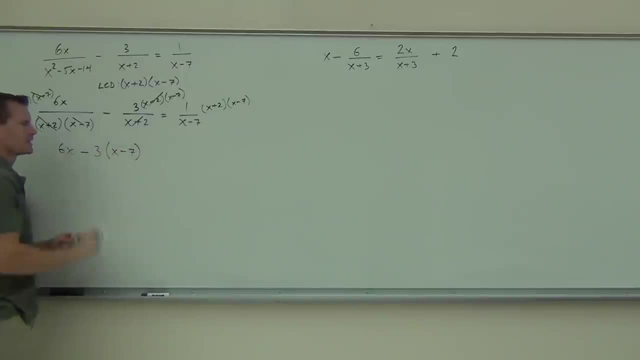 Okay, That's an important step. I'm still seeing that in some of your homework that you're not distributing negative. So when you get this homework back, some of you have the wrong numerators and have crossed it out because you're not distributing the negative. 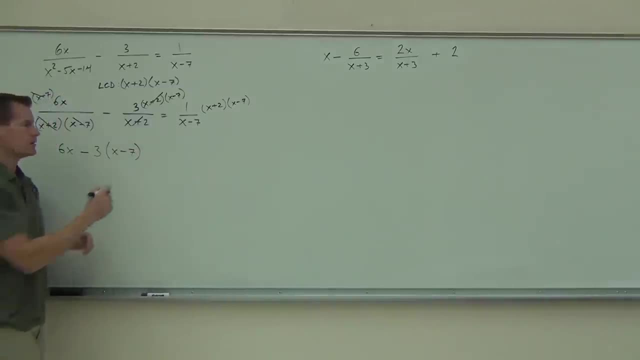 and you're adding together like terms that really shouldn't even be there. So be careful on that. Over here on the far side of our equation, the x minus 7's are gone, We have x plus 2. And now we're kind of on the home stretch. 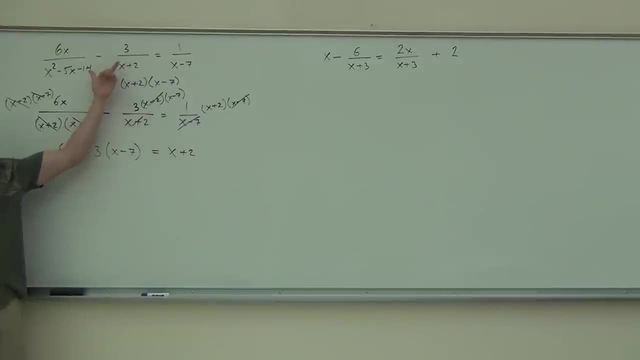 This is a very basic problem. considering we started with that, I mean just one step and we have something very nice. We're going to distribute, So 6x minus 3x and of course we're going to get plus 21.. 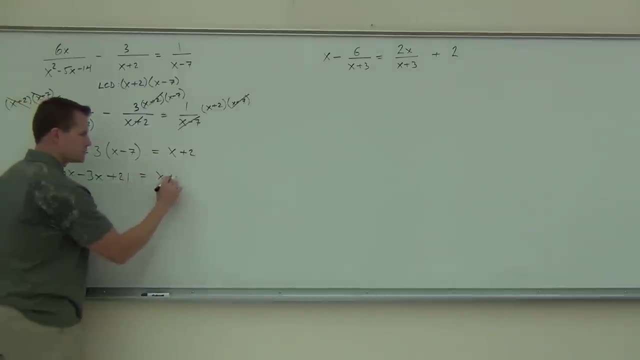 Do you see where that's coming from? Equals x plus 2.. We're going to combine some like terms, if we can. Here we have 3x plus 21, equals x plus 2.. Get everything to one side or solve it directly. 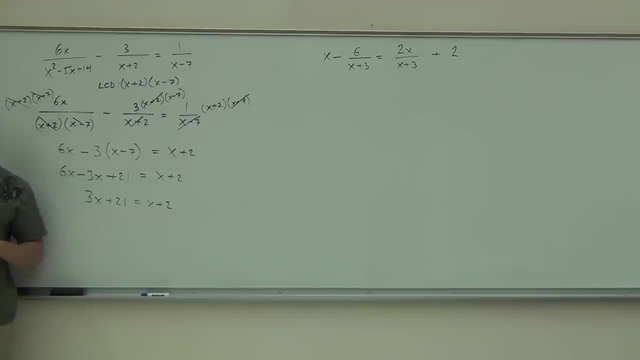 What do you think? One side? Do you have an x squared? No, No, No. So do I have to get everything to one side? No, Okay, So we're going to subtract the smaller variable From there. it's a piece of cake to solve. 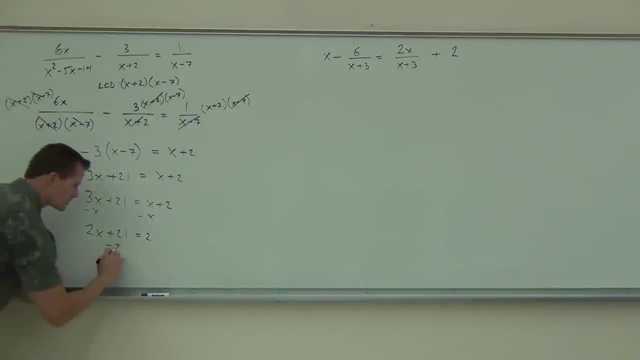 We get rid of the constant and our last step is to divide. So we'll subtract 21.. Divide by 2.. Unless we've made a mistake somewhere, that should be our answer. Huh, How many of you will feel good about doing a problem like that one? 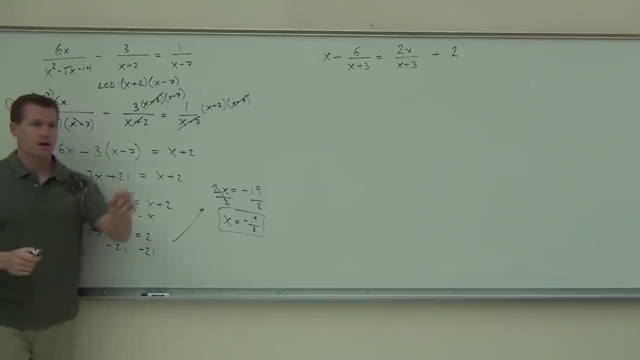 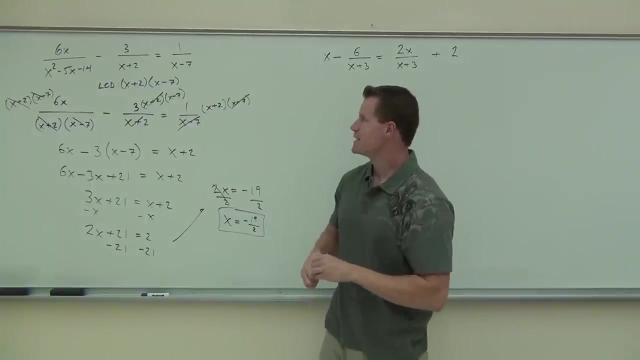 Middle row. are you guys okay with that? Yeah, Okay. How about left row? Are you guys okay with that? Yes, No, Yeah, Okay. So the whole idea is: factor: find your LCD. use that if you have an equation. 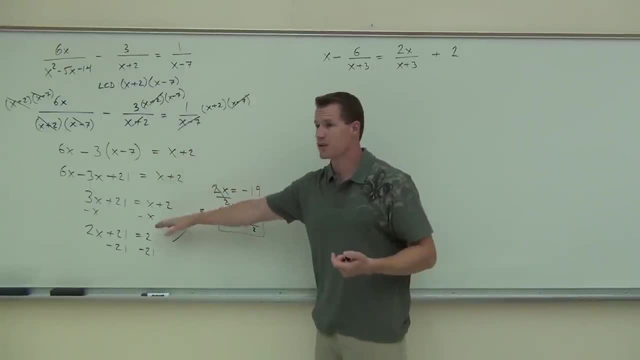 to simplify your denominators. After this, I went through this really quick because this is old stuff. I mean, this is really really old stuff, So this from here should be like a no brainer. The really the only thing I've taught you in this class is how to do. 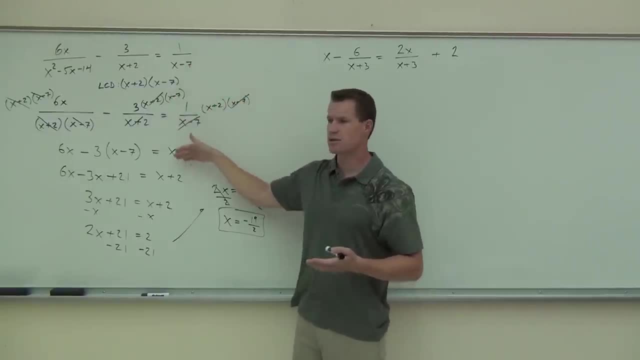 well factoring LCD and then using that to get down to this stuff. This is really this class right here. This stuff is all pre-algebra stuff, right here. Okay, now the next one. we're going to go ahead and look at this. 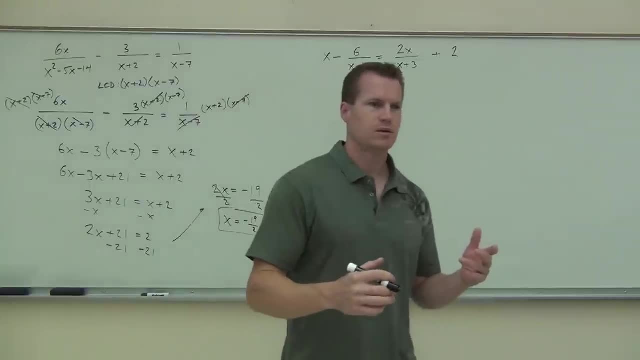 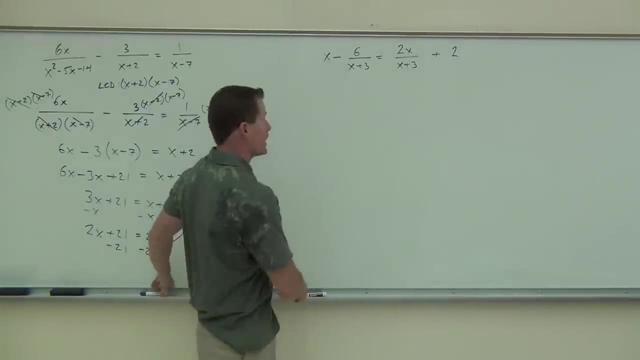 Before I even think about the LCD. what should I do? Okay, so maybe make these things into fractions. so you're not considering this and this as your denominator, So we'll do that. We'll change this into a 1 and over 1.. 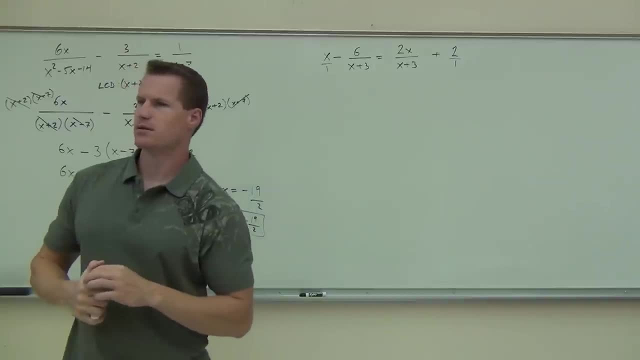 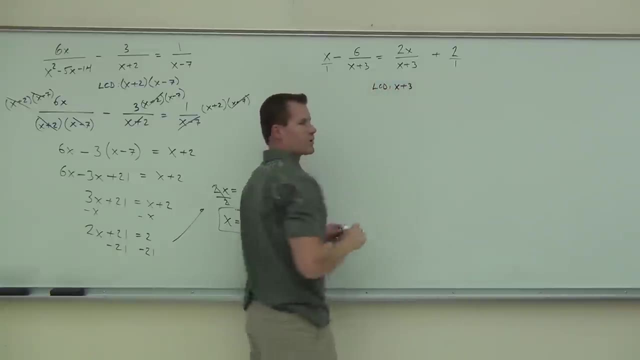 Ladies and gentlemen, I hope you enjoyed this. Thank you, Okay, everybody, what is my LCD here? X plus A, That's great, Okay, What am I going to do with that LCD? Multiply it by each term. How many terms are there here? 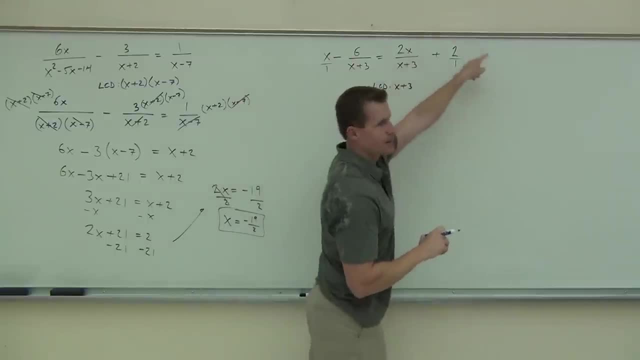 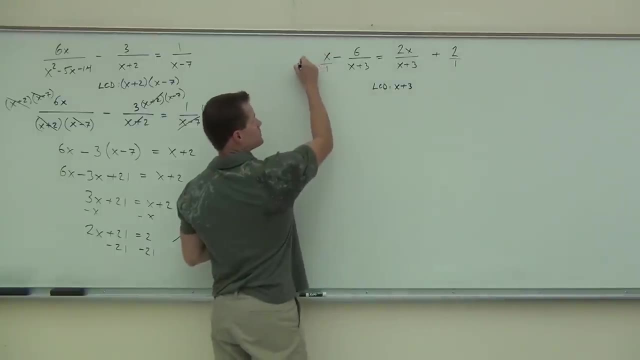 Four, Four. So that means here and here and here and there. Am I doing X plus 3, over X plus 3, or just X plus 3?? What do you think? Just X plus 3.. Good, So I'm going to do X plus 3.. 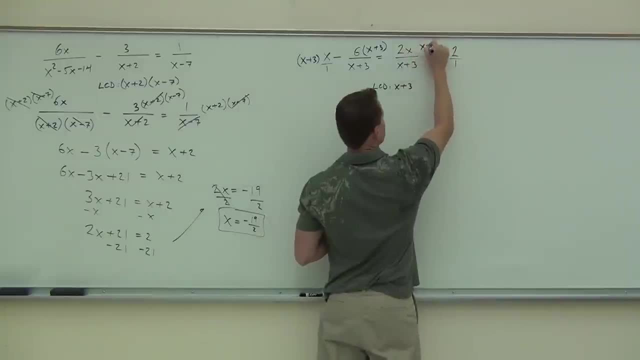 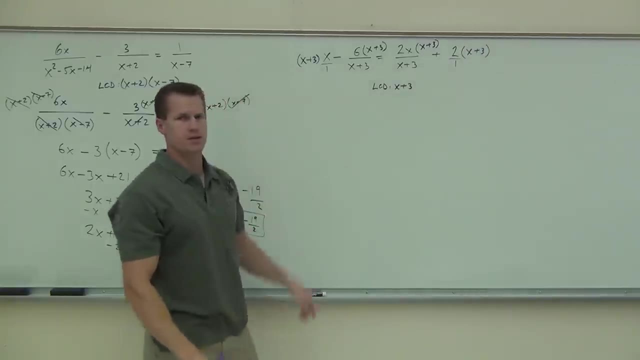 And here I'm going to have to have this. I'm going to have to have some parentheses, Of course, if you want to show it over 1, you can do that as well. I don't choose to, because we really know what's going on at this point. 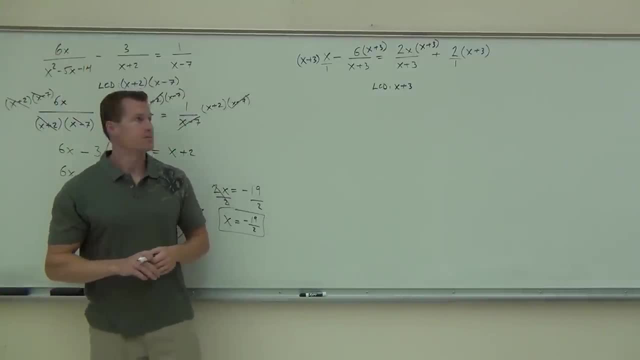 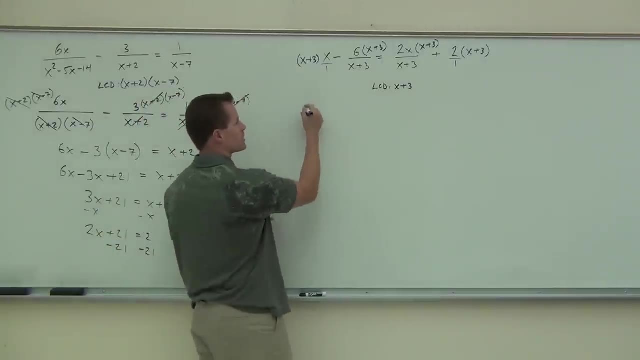 Do you see anything that's going to simplify X plus 3.. How about here? No, No, So before I distribute that, I'm just going to write it a little bit different, Just to make sure I see the same process here. I'm going to write it X times X plus 3.. 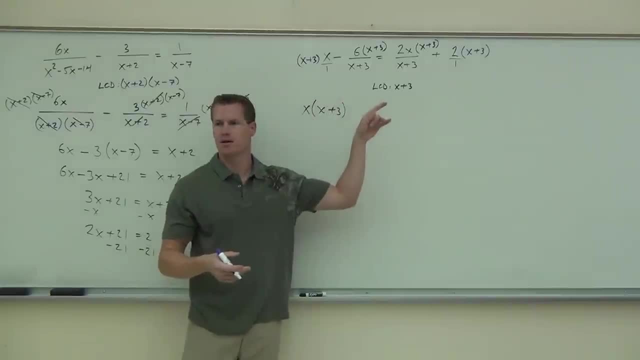 No problem, Nothing simplifies there. How about the next fraction? Does anything simplify? Yeah, there you go. So what am I going to have? Negative 6.. Negative 6.. Okay, That's the left side And I have an equal sign. 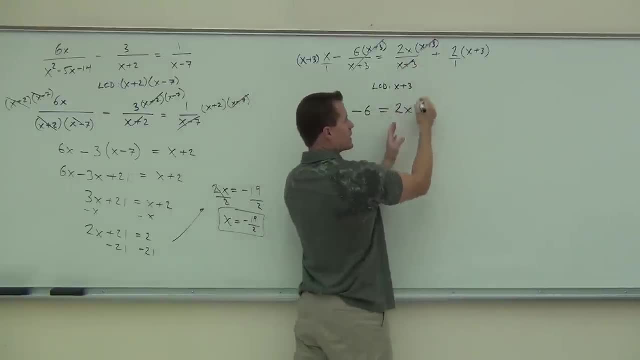 Here I also see the X plus 3's are gone. I get 2X And then I get plus 2 times X plus 3.. Again, I'm not distributing it in my head because I want to make sure that this sign. 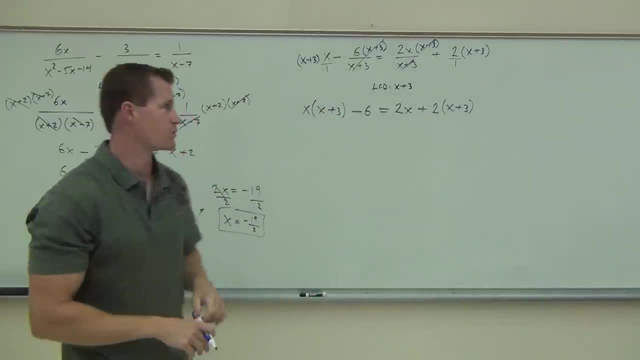 whatever it gets, whatever it is, gets distributed. That's kind of an important process for us. Okay, Well, that already looks a little bit better. What are we going to do next? Distribute, Distribute, Distribute, Distribute. 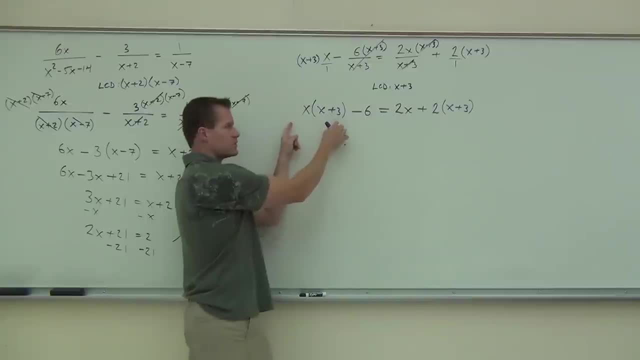 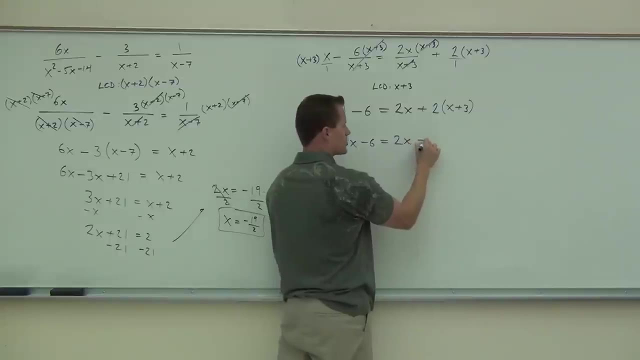 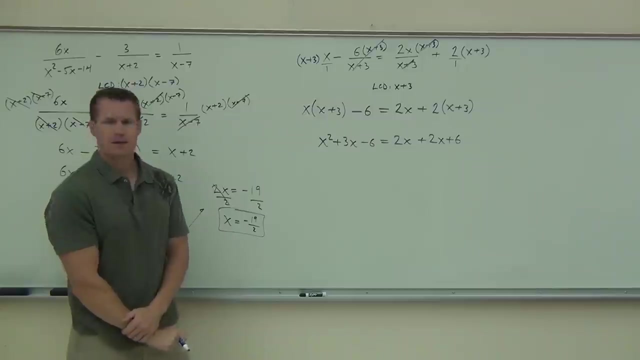 What am I going to get when I distribute this? first, X squared plus 3X, I still have that minus 6, then I have 2X and I'm going to get 2X plus 6.. Keep going, Someone on the right-hand side of the room. 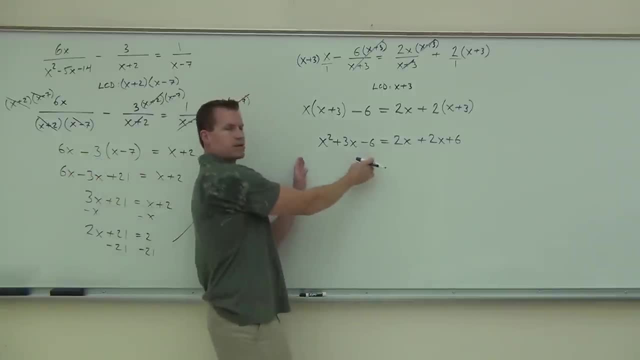 What now? Okay, Do I have any? on the left side? Right side, Yes, Okay. Now here's where you need to know what to do. Either you know what to do or you're going to get stuck on this problem. 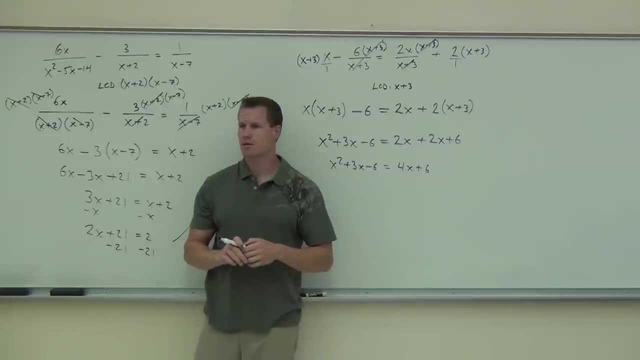 Do we get everything to one side or do we solve it directly? What do you think? Everything to one side. Why is that different than this? Because it's X squared. That's right. That's exactly right. So here I'm going to keep X squared, positive. 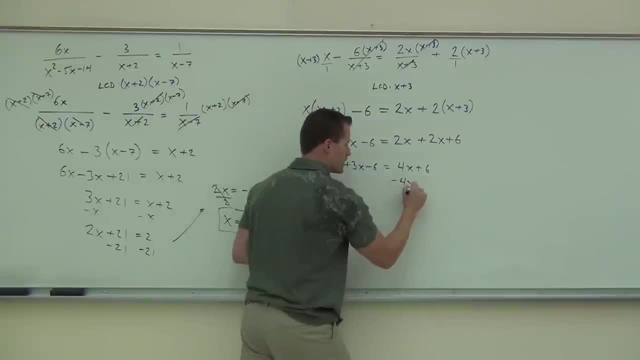 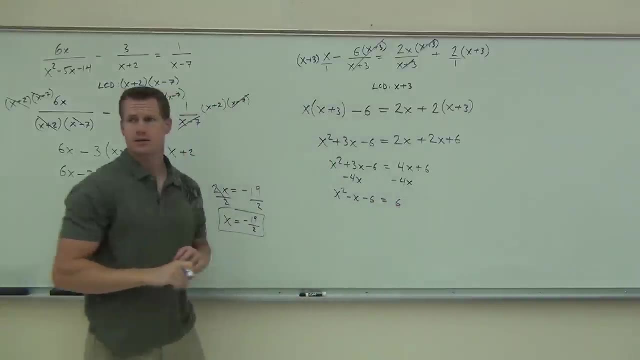 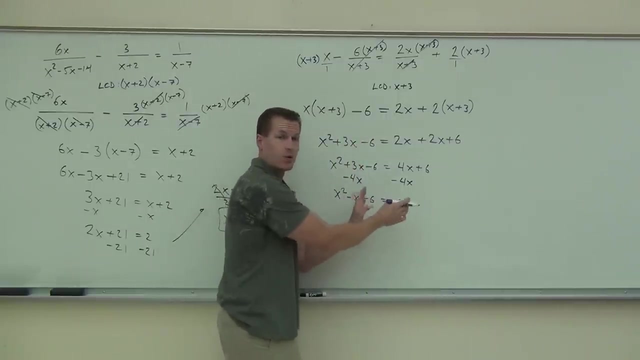 I'm going to move this stuff over to the left-hand side. So minus 4X. Then Let's do that. We can't do this. we can't factor yet because we don't have the zero. We need a zero over there for the zero product property to work. 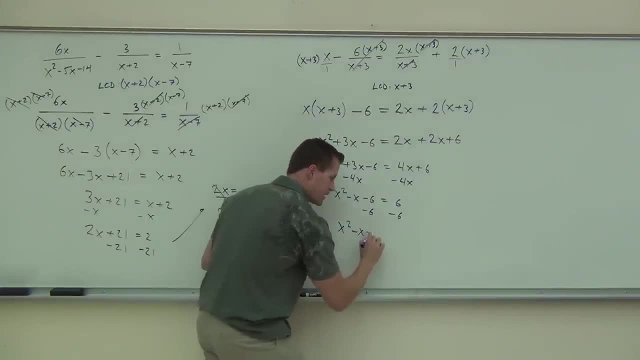 So that's why we have to keep going and get X squared. minus X minus 12 equals zero. That zero, that's really important. We've talked about that a few times in here. You have to have the zero. Okay, We have the set equal to zero, and now what do we do? 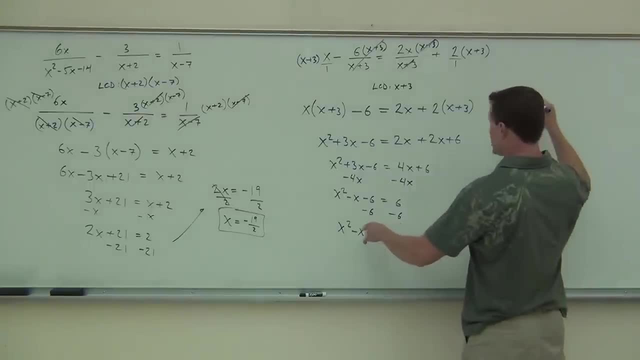 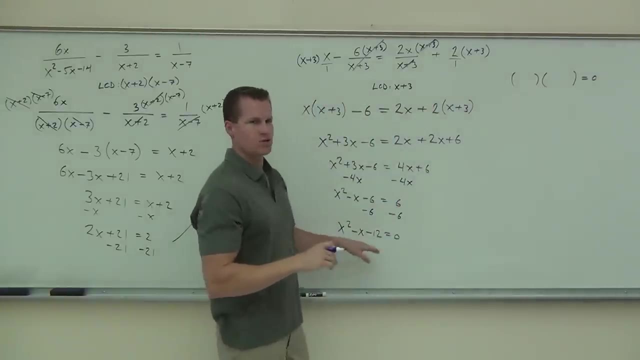 Yeah, The diamond method says we're going to factor that thing, And here at this point, we should be really good at factoring these problems. There's no extra step, It's pretty basic. We're going to get X minus 4 and X plus 3.. 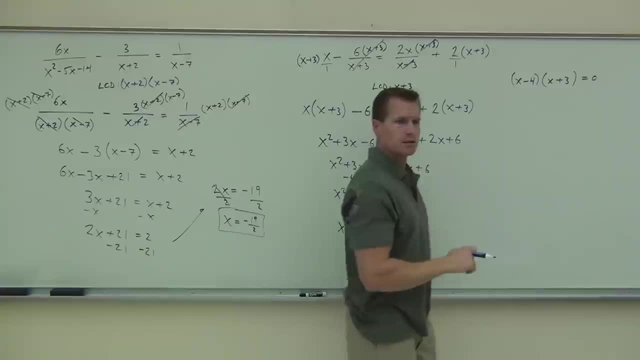 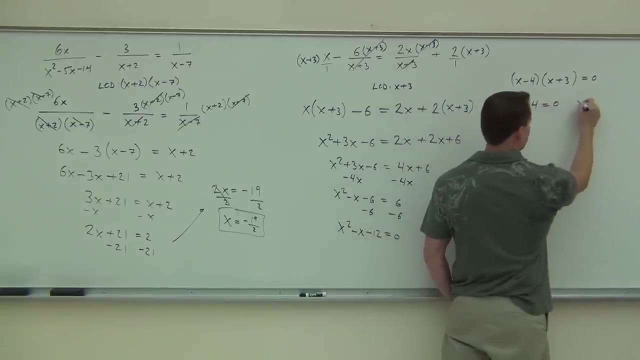 So far, so good. Are we done? Now? what Set each one equal to zero? Okay, One last little step. We add 4.. We get X equals 4.. We subtract 3.. We get X equals negative 3.. 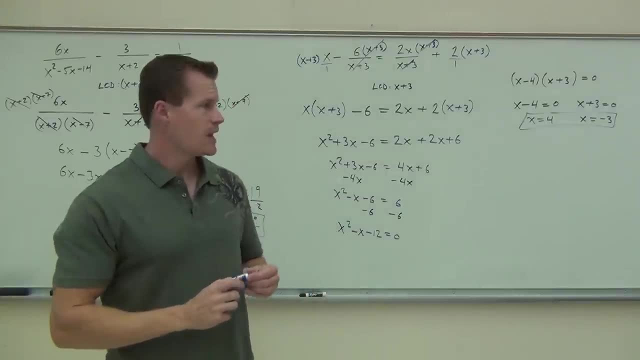 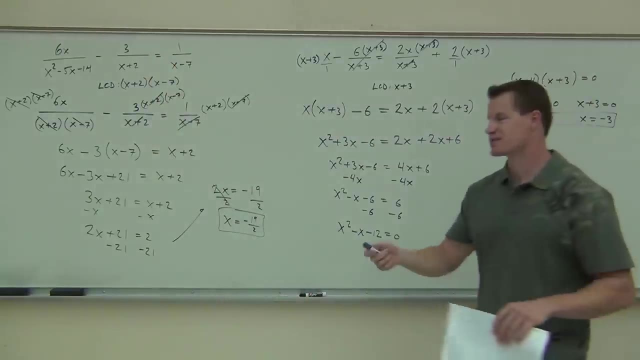 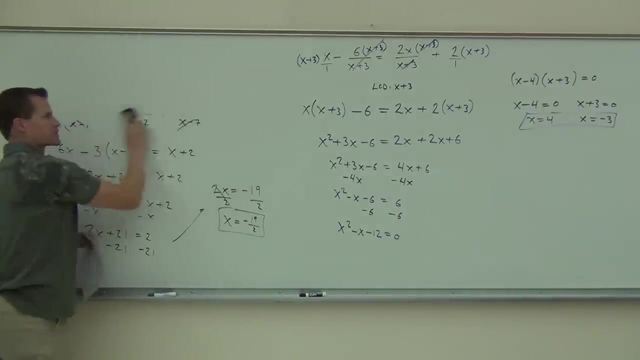 And we're done. How many of you feel okay with solving these things? Good, Very good. Now we get to move on to Chapter 7.6, or Lesson 7.6,, I would say- And in this section we're going to talk about how to solve some problems. 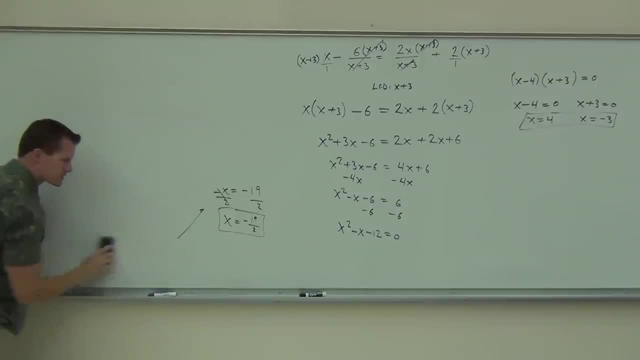 I'm going to give you a couple techniques. We'll be able to deal with several different problems. I know problem solving is probably not your favorite thing in the world. It's probably not your favorite thing in the world to do. Yeah, Isn't the negative? 3 negative. 3 plus 3 equals zero. 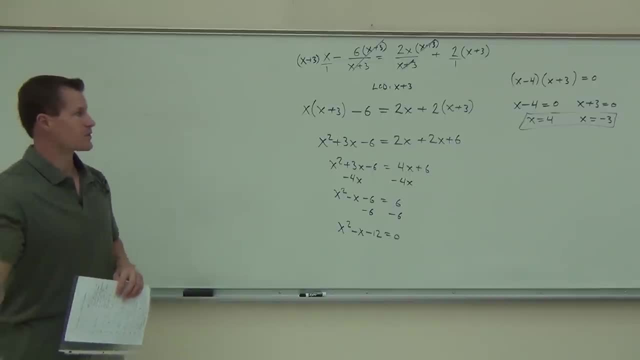 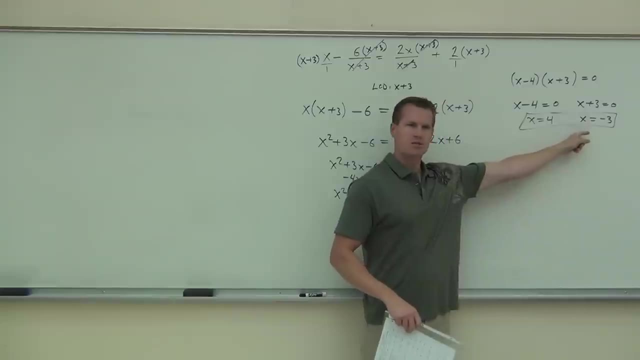 And that was kept from the last one. Oh good, Yeah, we had to keep. we forgot to check that. Yes, you do need to check your answers. So the 4 works. You caught the negative 3.. Does everyone see what she's talking about? 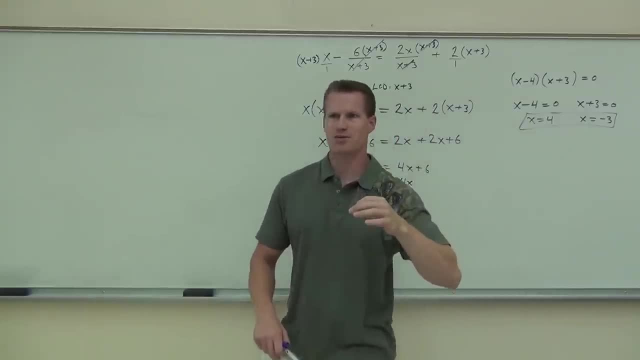 Yeah, I said last time I broke my own little rule. Good catch, I was just testing you. You passed. Yeah, The 4 is just fine because we plugged that in and it makes 7 and 7.. But she's absolutely right.